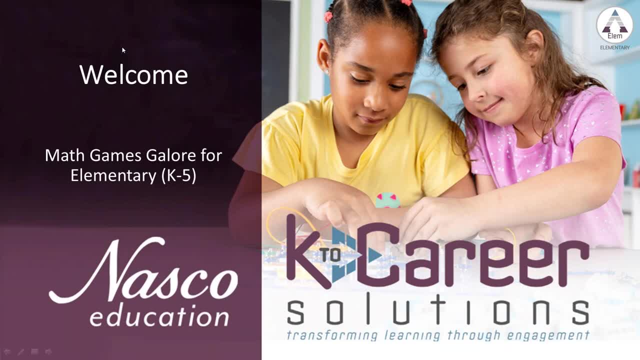 you've heard of us, Maybe you haven't, and that's okay. Either way, my goal is to make sure that you leave this webinar with new insight and can use it for your own needs. With that being said, as attendees are signing onto the webinar, I did want to mention to 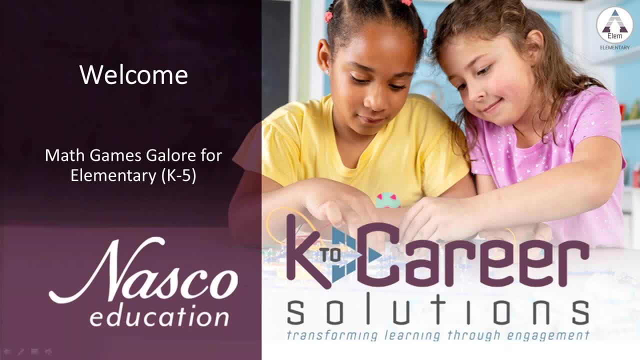 everyone how you can communicate with me. today. You'll see on the webinar control panel, there is a questions tab, and this is how you can ask questions, write comments and interact with me throughout this webinar, Since I have a lot to cover and I want to maximize your. 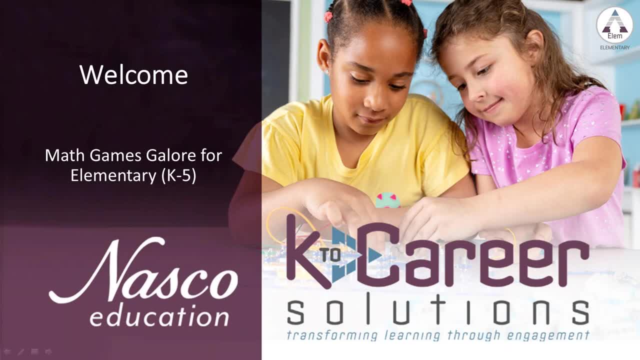 time. I'm going to answer questions at the very end, but feel free to introduce yourselves or add comments along the way in the questions tab, And also keep in mind that this webinar is being recorded and you'll have access to it about two hours after the presentation. 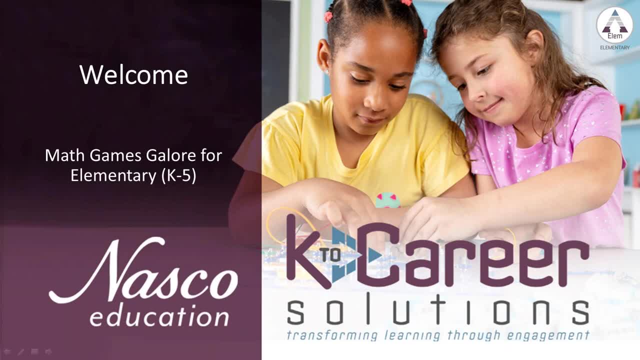 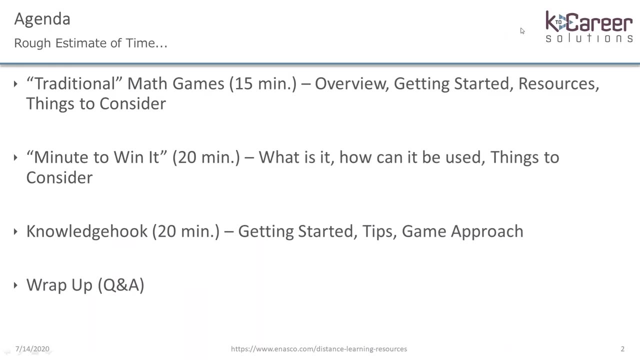 And you'll want to fill out the survey too, at the end as well, because we use this feedback to improve our webinar. So, with that said, we're going to dive right into the meat of this presentation. So, agenda: Here's the agenda, what we're going to do. 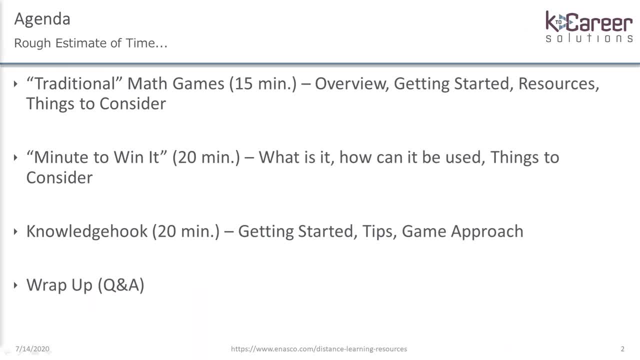 for today. We're going to be give you a quick overview of games in general. We're going to be talking about online gaming. We're going to be talking most of you already use a variety of games or and or looking for other games. 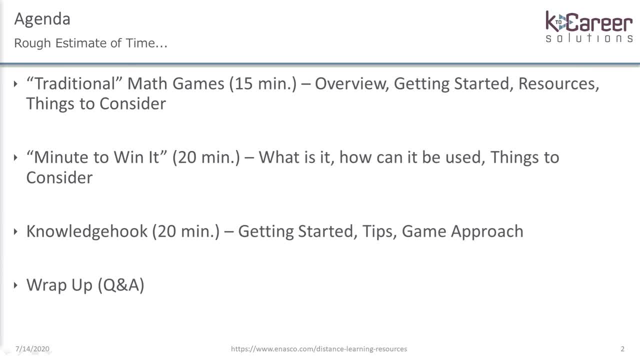 to use with your students, but we'll cover some aspects- resources- that maybe you haven't discussed or thought of. we're also going to be covering something called minute to win it. I recorded a separate webinar on this topic, but this is also something that can be related to fun interactive games. 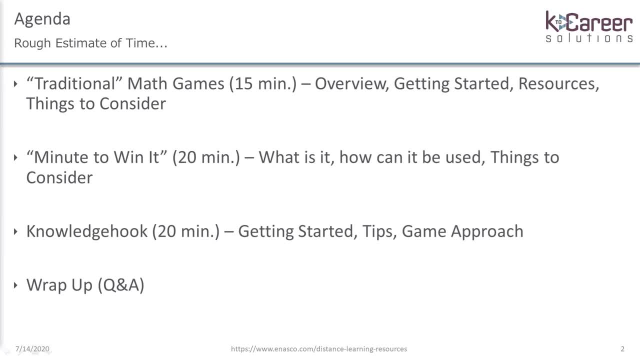 you can do with students either at home or in the classroom. we're going to be focusing on math concepts that you can use with this strategy. next, we'll be leading into our conversation into knowledge hook, an interactive guidance system that really works well with incorporating games and engaging. 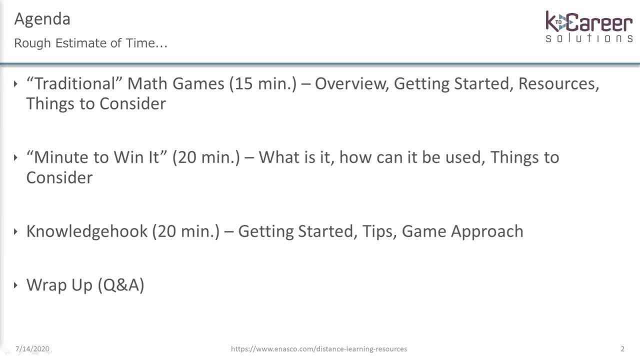 components for students learning and driving student outcomes, and then we'll be wrapping up with a Q&A. so this is the webinar. it's gonna feel pretty fast paced because it again it's only one hour and there's a lot we're going to be covering, but what we're trying to achieve today is exposure to a lot of. 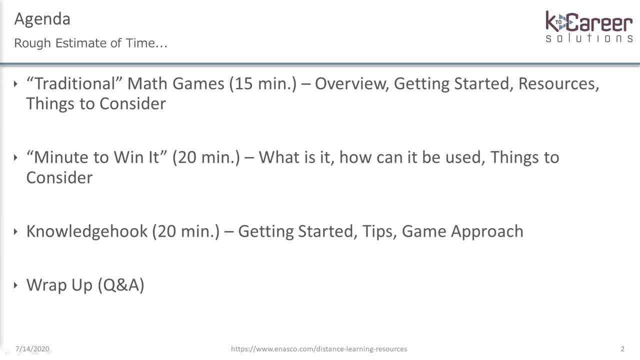 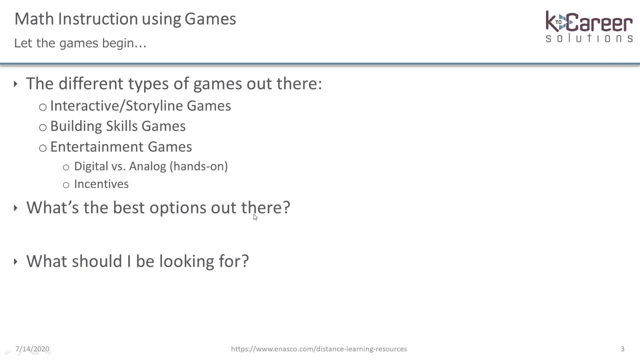 different resources and ideas that you can use immediately following the webinar. so let's have some fun and let's jump right into the meat of this presentation: math instruction using games. using games isn't necessarily a new concept to the classroom. growing up, I remember a lot of different games we played in school. 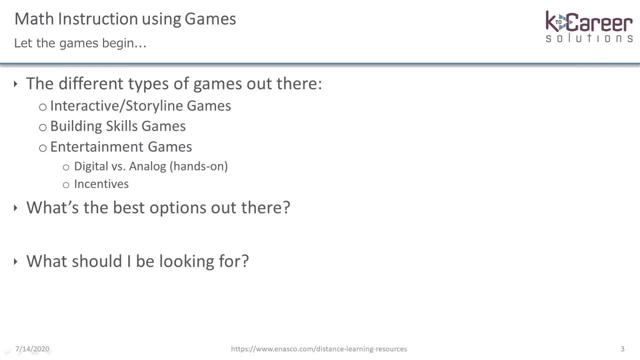 Simon Says, Red Rover Heads Up Seven Up Twister, Oregon Trail, etc. and as I reflect on my own education, I know that some were more educational than others. right, so some were just fillers for time. you know, some are used for building a positive classroom environment by having 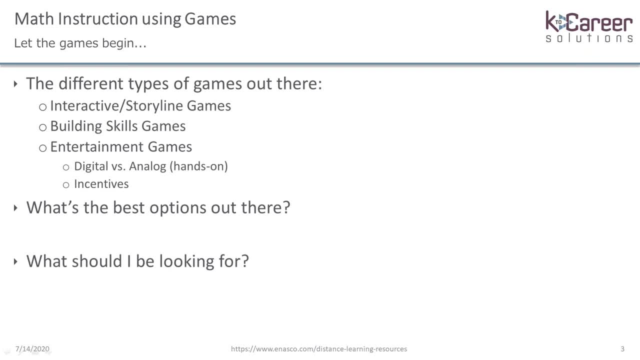 students interact socially, and so there was a variety of different uses for games, and even today, the games are shifting. instead of using, like you know, bingo or Jeopardy, now they're using things like Minecraft, sims and like Carmen Sandiego on Google Earth. it's not to say the current, older games. 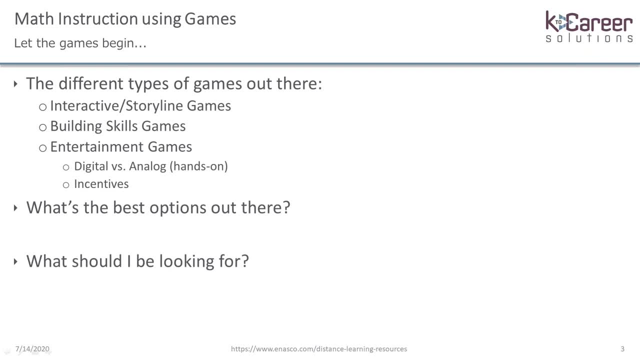 are antiquated, but the advancement of technology. it's only natural that the games coming out now are more advanced and sophisticated. but that's just not a good outfit. that ya know. on esports we don't have a class area on campus, right. yet you know, with first of all those mobile games, whether you're using games. 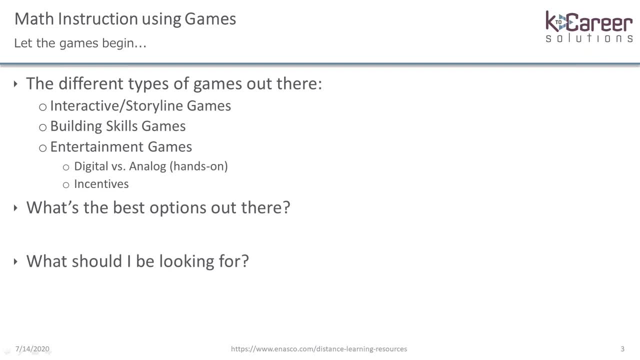 you know, or devices when you're operating systems, because if you're using screens applications too early, you knew you wouldn't even be pushing all your things. That doesn't necessarily mean that they're more educational. It's just that we're going to be focusing on a lot of our discussion on that today. 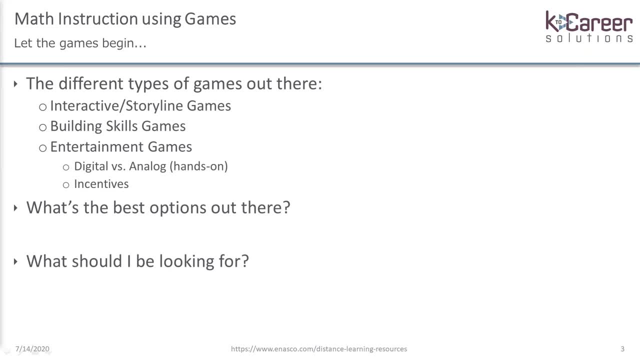 So there's many different types of games out there, but I've more or less kind of bundled games into two areas One. the first area is interactive or storyline games, meaning there's a plot and story along with the game that the student engages with when playing. 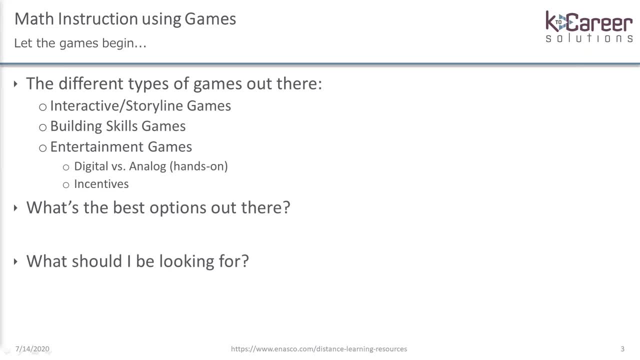 You know, you gain levels, power ups, new information about how to solve the main problem, etc. These types of games typically take the longest to implement and use in the classroom, but there's good benefits of using them if used correctly. The second type is game is most traditional in the classroom. 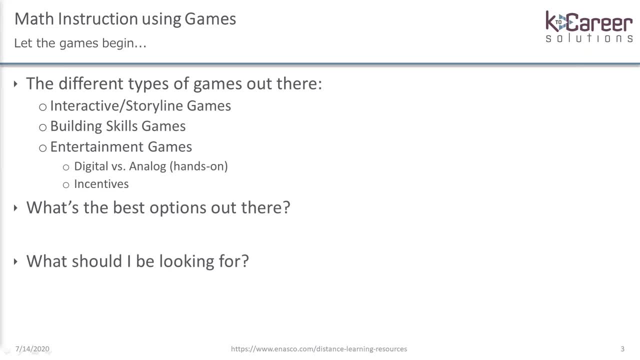 It's your classic game that teaches you how to play the game by giving the rules or instructions in the beginning And then, as you play, you become more familiar and get better over time. It's a game designed to teach something, usually specific, like addition, subtraction, multiplication, decimals, etc. 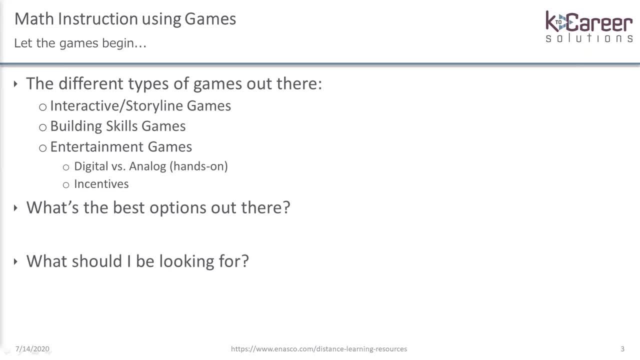 And its purpose is to mainly enrich the curriculum or lesson. that was done To help students hone their skills. the Len, you know. the last area revolves around simply pure entertainment. These games typically have little to no educational value and the focus is students who are bored and want something to do right. 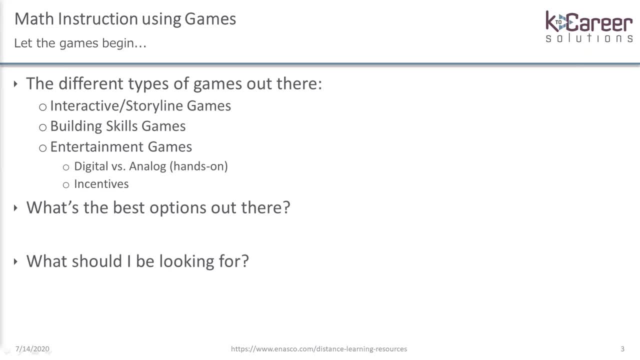 These. these can be deceptive to educators because it might appear that students are engaged, but there really isn't learning happening. Games can be disruptive or seen as barriers to learning if not managed or implemented properly, And we'll get into those in more detail throughout this presentation as well. 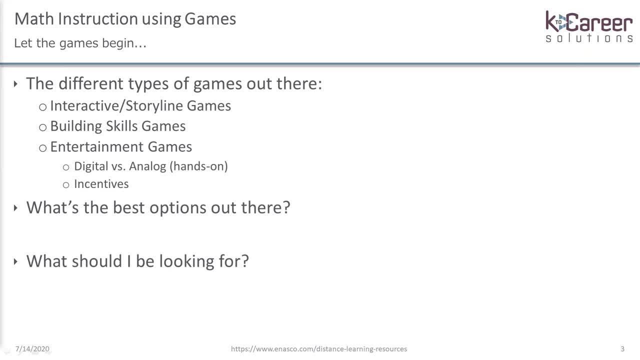 But I want to emphasize that each of these different areas are not truly representative of everything out there, but represent what I've come up with when the within each of these areas you can have incentives tied into the game. You can have it delivered digitally with, like an iPad, Chromebook, computer browser like Firefox, Internet Explorer, Chrome, etc. 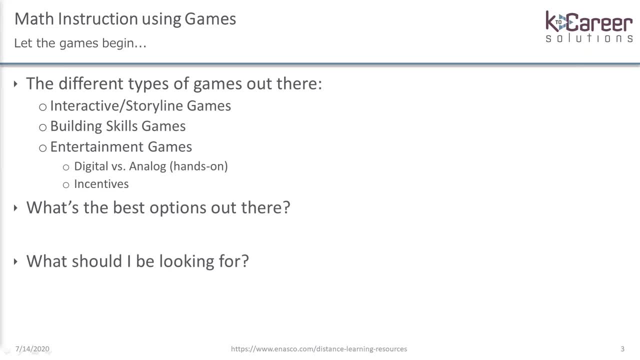 Or it could be, you know, quote unquote- old school, with paper and materials laminated and used over and over again. So, either way, there's a lot of a lot out there, And there's a lot out there, And there's a lot out there. 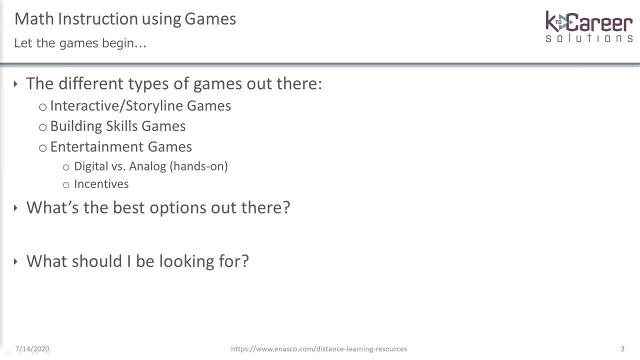 There's many different types of games to explore and learn about. So where do you start? What are the best options out there? What should you be looking for? These are the kind of questions we're going to cover throughout this webinar today. So, math games: you know the good, the bad and the ugly. 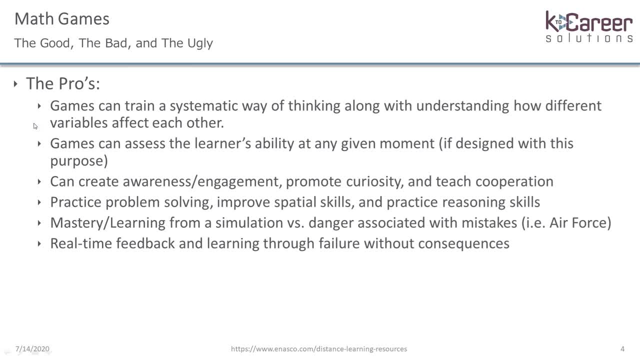 So let's talk about the pros and cons and everything in between. It's good to go through some of this and also realize this doesn't list all the pros, but it gets you thinking about what games can do in the classroom. Oftentimes, students are presented with a problem that they can't solve. 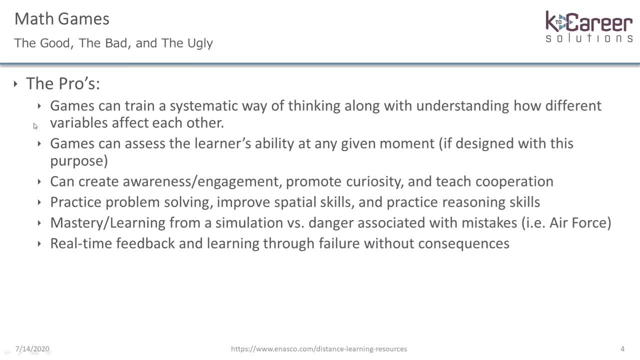 If they have to solve they need to get into, you know, point A to point B. There's but there's obstacles in the way. So students are kind of quote unquote, stuck in with solving how they're going to travel the distance needed to move to the next level. 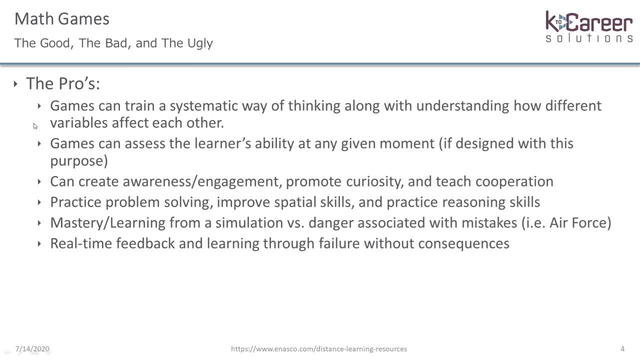 They're. they're sometimes limited on how they can move, when they can move, what they can use along the way, etc. So students instinctively go through this thought process and solving the problem without realizing they're synthesizing information and making informed decisions about how to solve a problem. 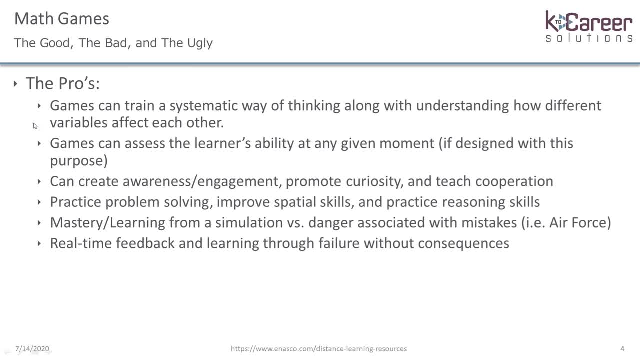 So, And then research has been done for a long time around assessment, both formative and summative. Games can also be used with these types of assessment if built correctly, and it can be used to better student outcomes if done effectively. There's a lot of studies around student outcomes from using games with instruction anywhere from increasing engagement and concentration, teaching cooperation, critical thinking, reasoning and spatial skills, time management and comprehension and evaluation skills. 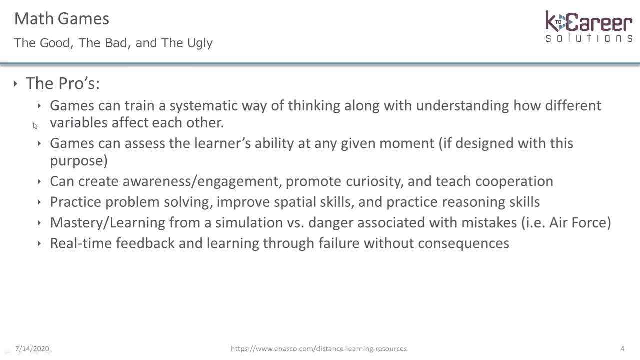 Then there's also the benefit of simulating real world Applications and life skills with training, for example, simulating landing a cargo plane or simulating owning a veterinarian shop and taking care of animals, where students might learn time management, materialistic value, day to day activities to run a business, and safety protocols, protocols. all of these are good training talking points and worth discussion if considering games into the classroom. 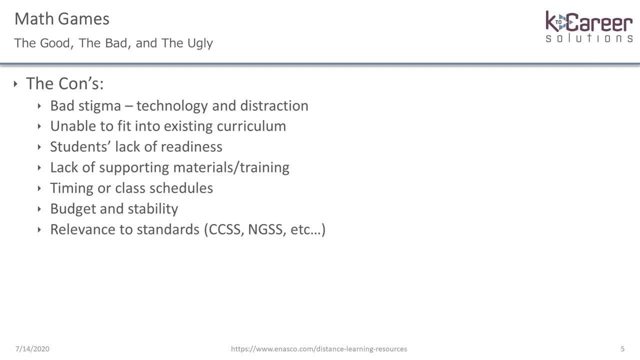 So let's talk about the cons. So let's talk about the cons. So let's talk about the cons. Right, One can argue that kids in general already spend too much time using technology, And this is based on their day to day activity. 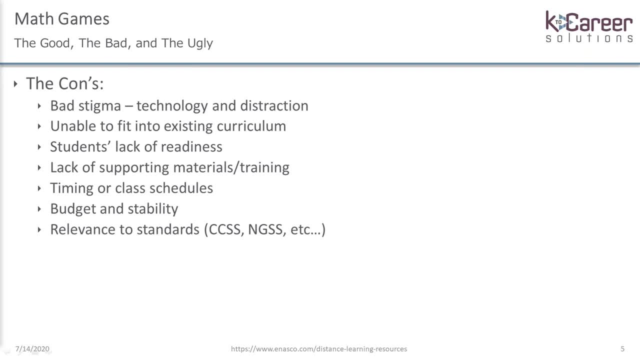 Excuse me, Students are estimated to be using between seven to eight hours a day using media already, And that's a lot right. And not only that, but games and or video games are seen as kind of a leisurely pastime for students and not considered a way to teach academics. 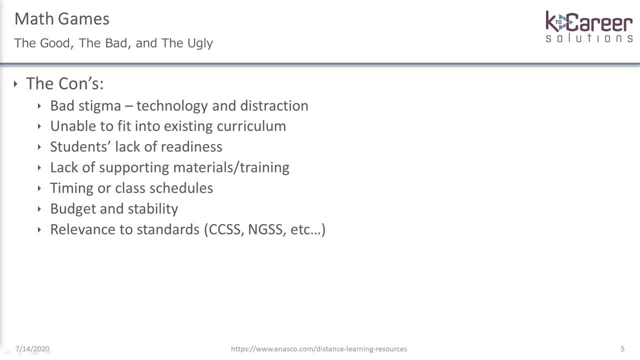 And, And so more Than 12 days a week, So than just an unproductive activity and distraction to the classroom at home- and this might not be your own personal viewpoint, but this does exist out there and you might have to overcome this in order to use gaming into your instruction. uh, with curriculum generally, 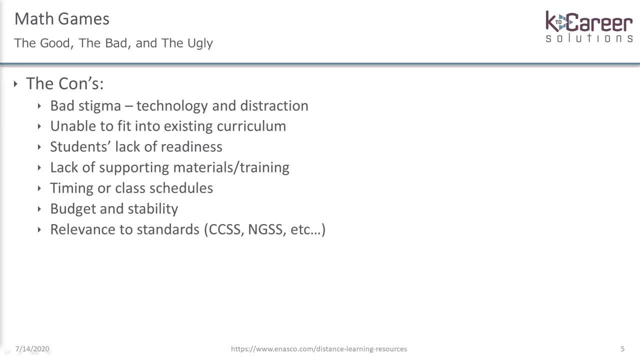 uh, being present around in classrooms, it can be hard to find the time to justify using games in the classroom, let alone an educational game that is also fun. now, some curriculums are designed with games in mind, but then there are others that do not, so it might depend on the situation. 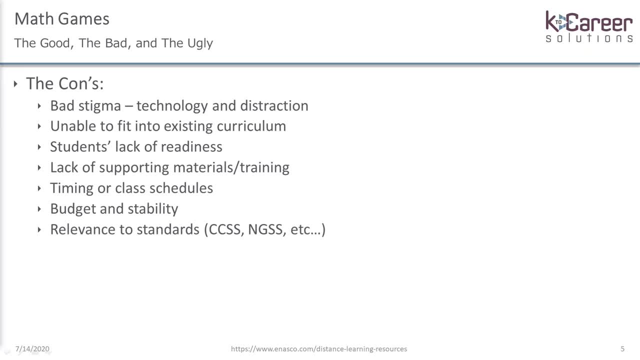 students lack of readiness, and this goes along the lines that all students have different, varying degrees of skill and computer literacy. students have to be able to learn games and sometimes games are harder for students to learn that tradition than traditional audio visuals, you know. also consider that students can lose the desire to learn in the traditional setting after. 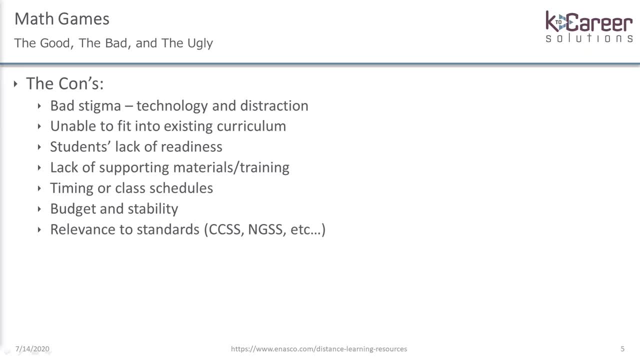 becoming maybe addicted to gaming. right? we ultimately want students to understand that learning can be fun, regardless if it's done with the game or not. you don't hear people often say: you know what? i just hate knowing so much right, like it just doesn't happen. uh, but math games might also. 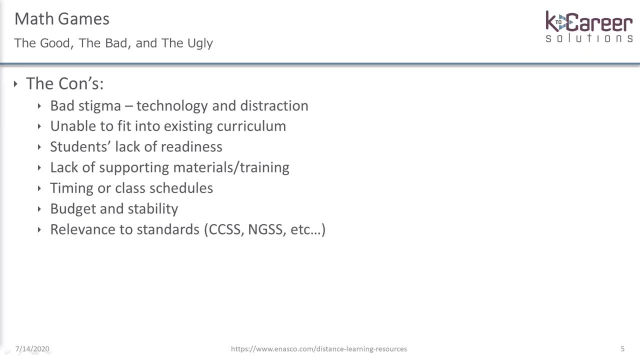 have something working against them right from the get-go, because many teachers have little to no experience in using games to teach or don't have access and support to work with students alongside games, so games become kind of underutilized. it's it's important that teachers 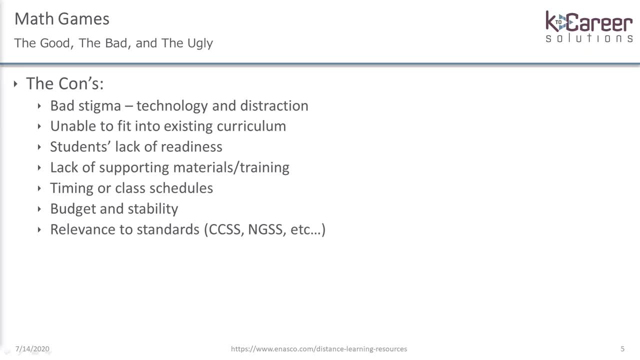 have training and time dedicated to be pd uh to implement games successfully. just keep in mind, though, that school districts have a certain budget, and while some are willing to invest in these kind of options, others are not as fortunate, especially if administration a principal or a fellow co-worker. 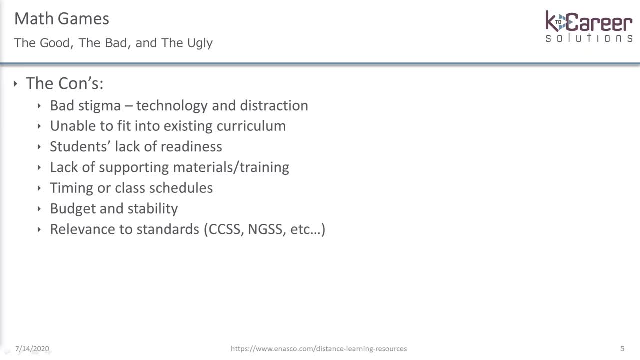 already have a bad stigma towards games to begin with another another con? um. that is that sometimes games require more than just a time frame allowed to implement a more complex game. sometimes sophisticated games can take more than a couple hours to learn and more time to play with certain. 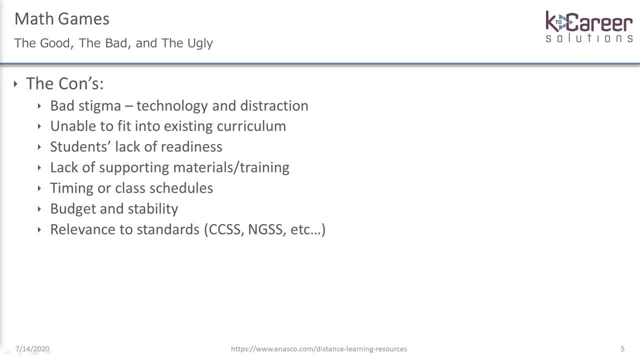 class schedules and how to the back to school. and we have an example of an astrophysicist who calls adults to go to school, and um, and he says i have an escape plan and i have to take three classes to go to school. um, and he's. 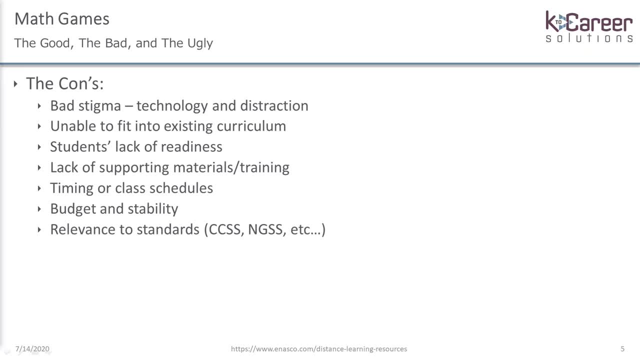 like: okay, i guess you could offer me a day off per class. uh, and he says: you know, you can take an extra hour to just go to school and you get a day off, but you don't need to be in school because most schools are open to you. know, you don't need to be in class, you just need to be in. 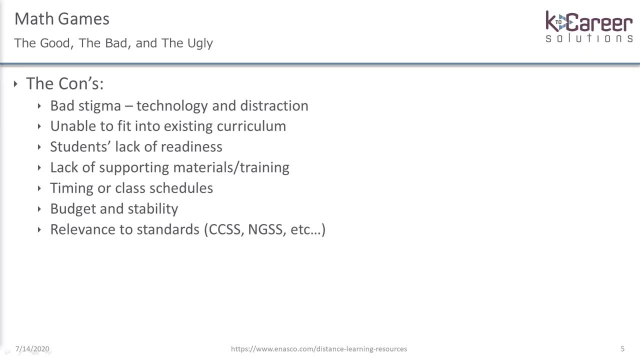 class to figure out what's going on in your environment. you don't need to be working and going to school. it's very simple. it's very easy to do it and that's what people think of things as robust as paid ones. so if your budget is limited, this also might limit your options. 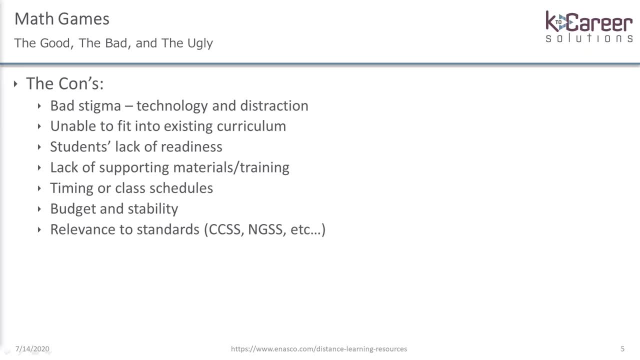 and present a problem to overcome, you might have to rely on additional funding or grants. so how do you make something happen long term if this is the route you plan to go right? and then, lastly, the relevance to standards: making sure that skills students are learning appropriate skills or 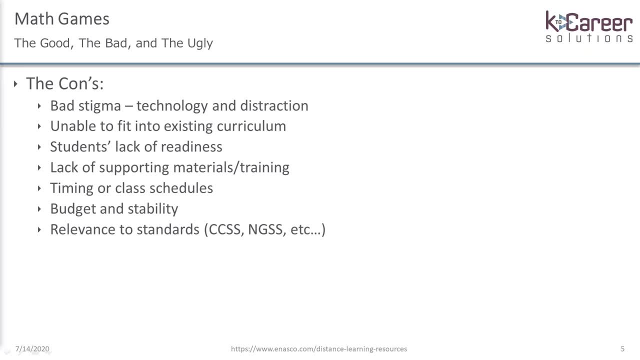 content. the last thing you want to do is mislead students. so while you're eager to play a game with them, you want to make sure that it's age appropriate and is providing the appropriate student outcomes you need to address. so sometimes it's unclear, so it takes an intuitive educator to 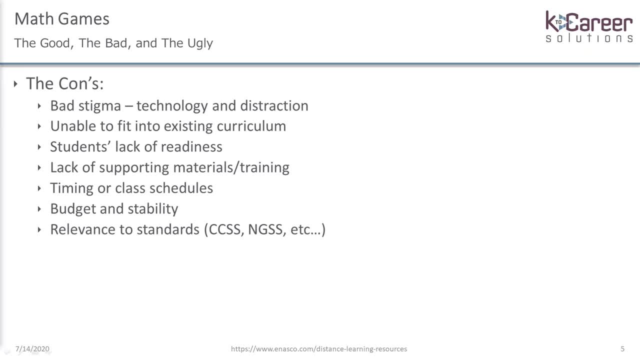 really understand how to utilize the game effectively, or more time to dedicate to the area? and let's be honest, who has just extra time sitting around to do extra projects? it just it's. it's tough already, um the adjustments that we've had to make, especially with going to. 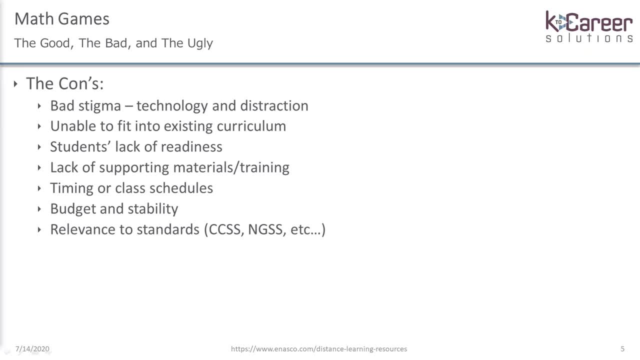 distance learning this year. uh, so there's a lot to think about and, as we move forward in the next couple of weeks, we're going to talk about some of the things that we're going to talk about in the next couple of weeks, we're going to talk about some of the things that we're going to. 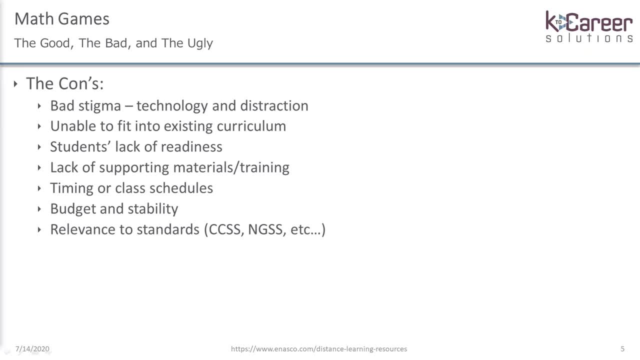 discuss how games can be incorporated in instruction. um. what we're going to do next is kind of review some games together and we're going to discuss what we think of them as a group. um, and this is this is where you can. you can do um and leave comments in the questions tab as well. 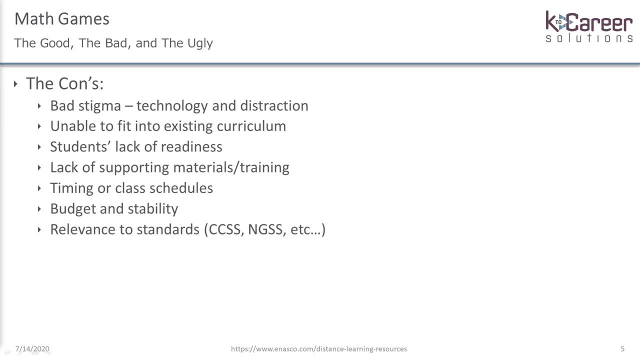 along the way, and for today's purposes, i was going to focus on free content and resources, because i know that's important to those that are out there right now. also, note that as we review these different games, don't worry about writing down the your url or feeling like you're missing. 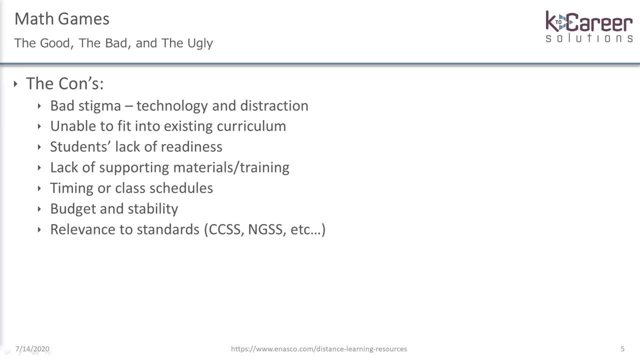 out on links. i'll have them in the deck so that you can go back to them later. after um, you are sent the recording of this webinar, so let's jump into our first uh set of lessons. we're going to uh go to something called um math nook um, and so i'm gonna exit out of this presentation, so you. 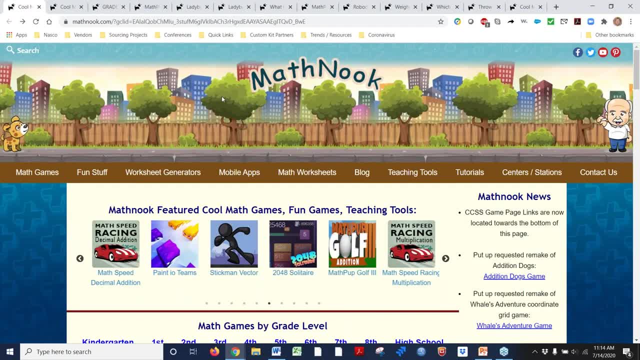 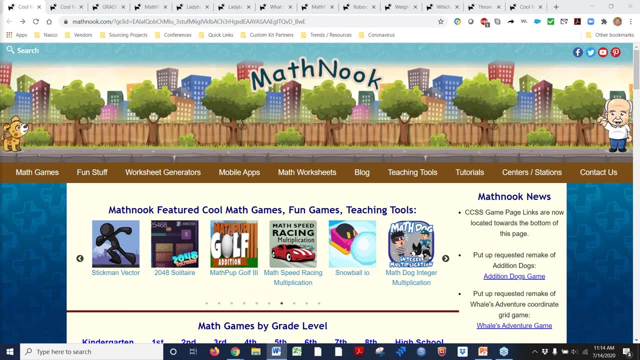 can kind of get a good see or visual of math nook. um, the first website, um, like i said, it's going to be matt duck, it's one word. maybe you've heard of it, maybe you haven't, and again, that's okay, it's website. there's a variety of games, the resources you can use. uh, first thing i want to show you is 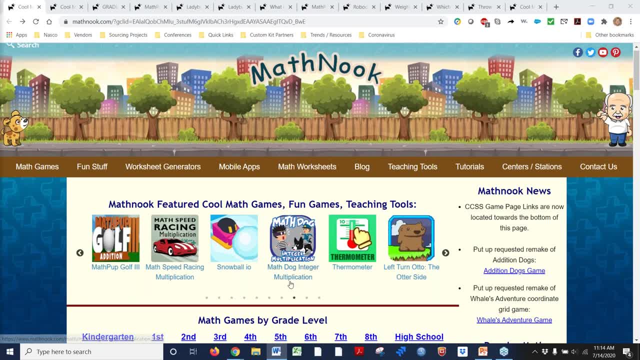 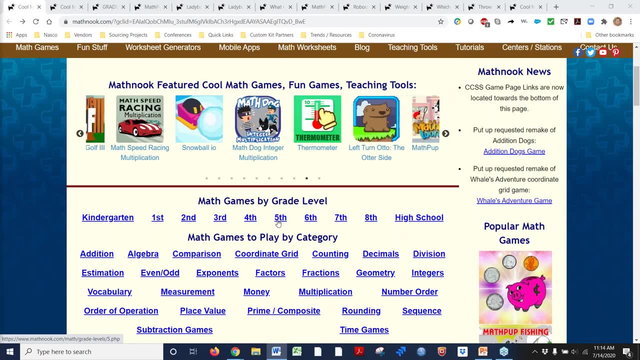 that you can split up by gray levels, so it's a little bit easier, uh, to be able to implement. now we're k to five, so we'd be focusing on these different tabs right here. um, what's also nice, though, is if you scroll down to the very bottom. what they have here are the common course, uh. 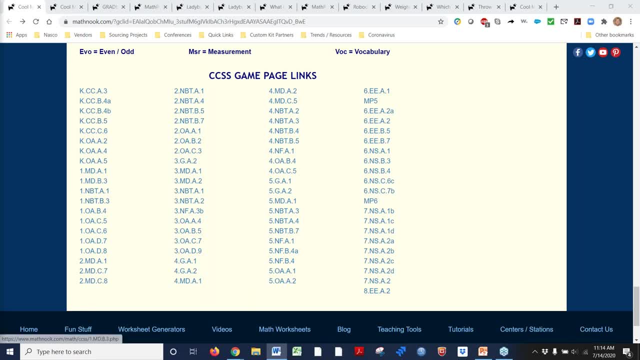 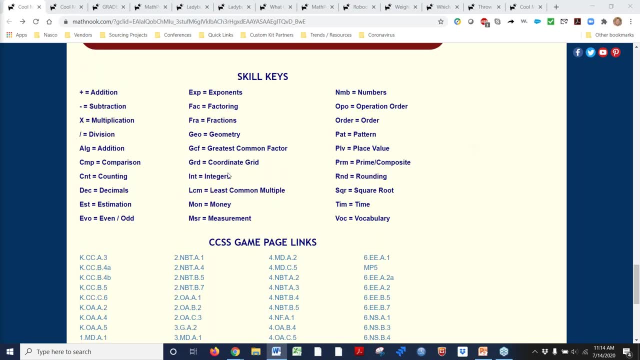 links so you can easily click on these different links to get the Common Core games that are linked to those standards as well. And then they also have skill keys, So this is important. So if you're looking at a game like Geo, this is geometry. 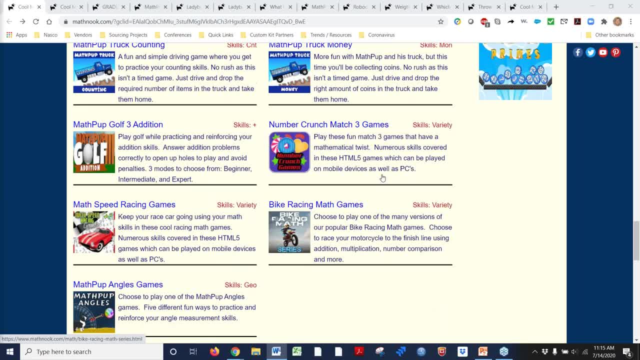 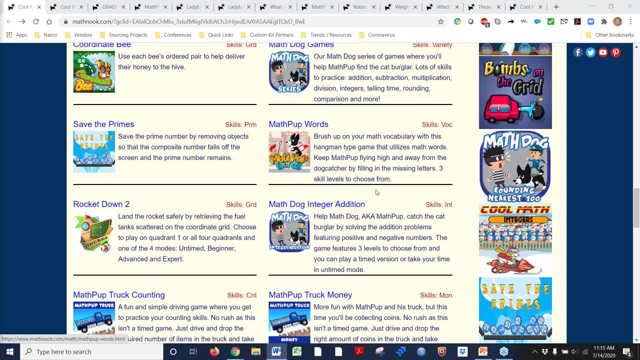 When it says skills variety, this might be a variety of different skills. You might have counting, You might have coordinate grids. If you're looking at this, you might see that, oh, this is EVO PRM R&D. 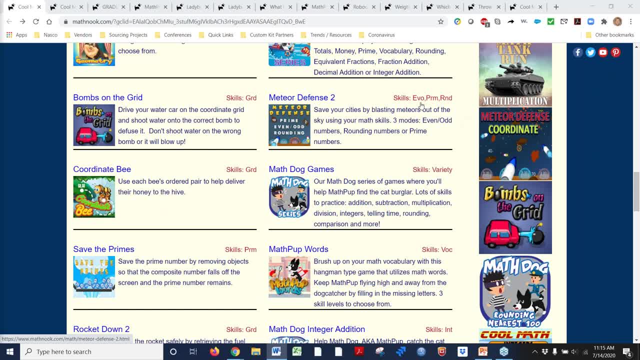 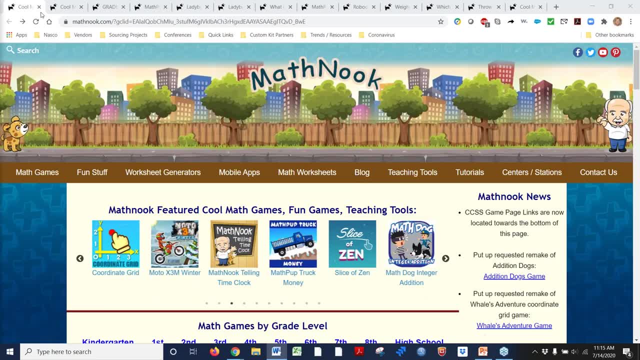 What does that mean? Well, that's prime numbers, even odd numbers, and rounding. So those are different skills that you might see for different games. So that's how this is kind of organized, But I've kind of jumped to different games that we can just jump right into to be able. 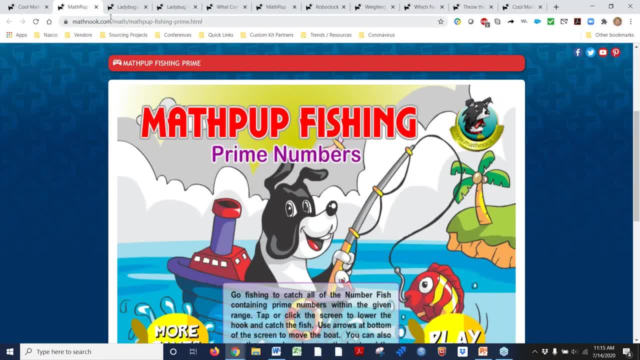 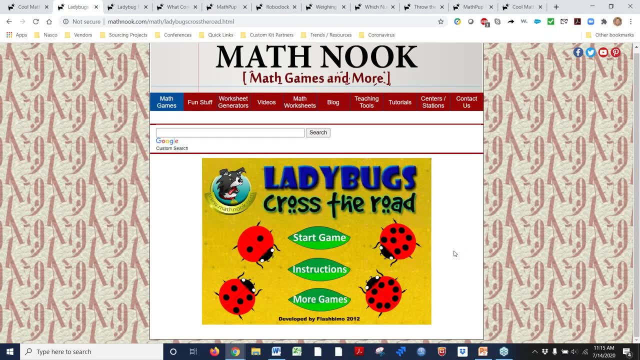 to use right away. So the first one that I'm going to- I'm going to actually throw this over here- The first one we're going to actually do is called Ladybugs across the road. So let's just jump right into the game. 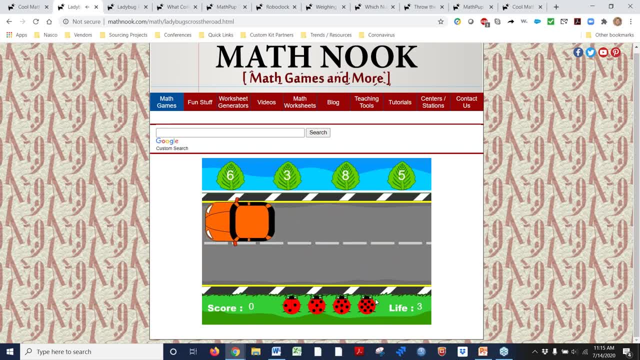 Now you can't hear the sound, but essentially what you have are Fort Earth and Ladybugs down here, So you've got one of those. You have the six stores that you're going to be able to walk down to here, which is the other game over here. 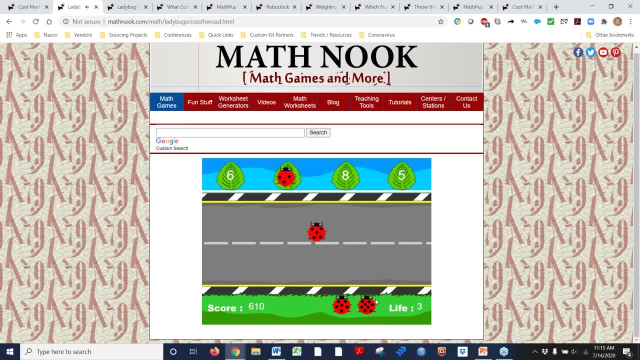 So now you'll notice that you have to run through your numbers just to see which one you're going to. So I'm going to go to my number one. It's going to be the number two, And I've got a little more of an idea than I see here. 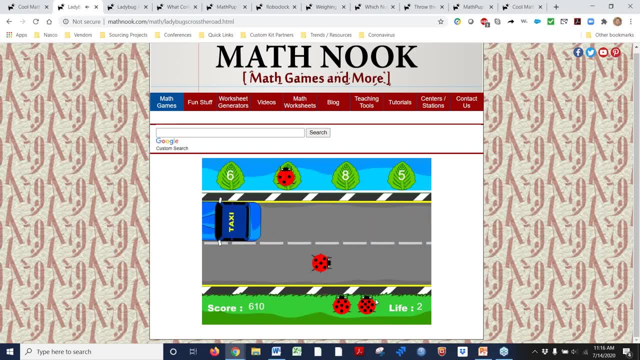 So I'm just going to go ahead and say, well, let's see if I can run through this. So if I can run through this number, I can see that we have a box right, And then I'm going to go over here and then I'm going to hit space bar. that's to the 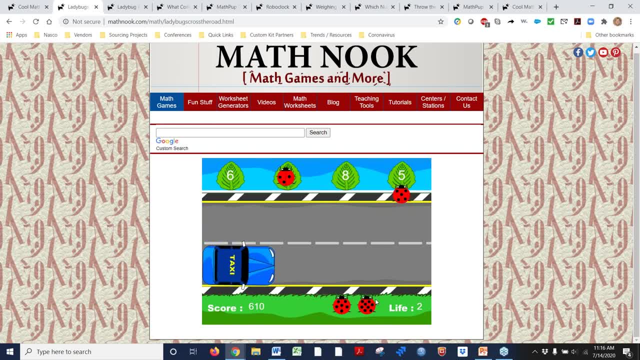 next one, And then I'm going to hopefully not get run over here. Oh, I did number five. I hit spacebar, I'm ready to go. so then I come up here to number six. and again, this is just a very easy way, as soon as you know the functions of the game, to be able to start. 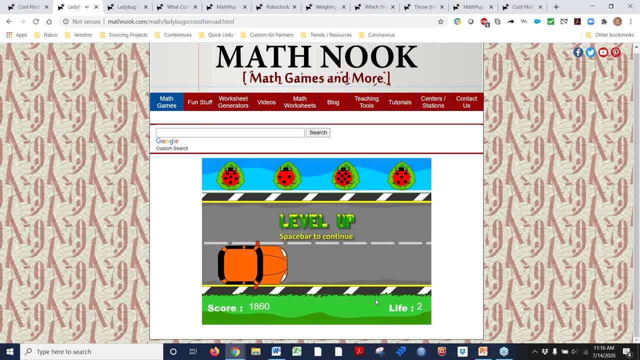 interacting with the game itself. now it says level up. you press the spacebar, then you're able to go to the next level. so now we have a little bit harder right. so we're doing three right. so now these moving leaves are going to be able to interact with you and notice I have to hit. 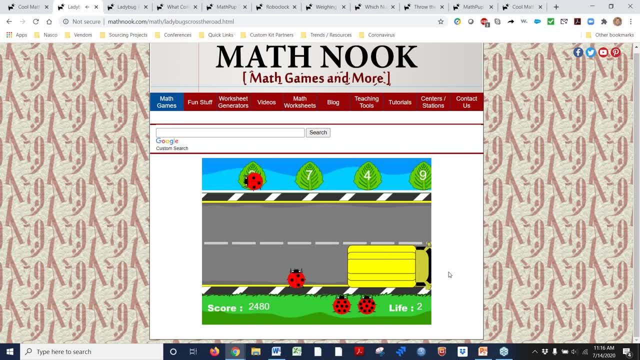 spacebar in order for it to stop. so one thing that you're going to notice, though, is that, as I'm going to be doing this, I'm going to show you a little glitch that I found when I played this and this. this is something to be aware of with all your students. now watch what happens when I come up. 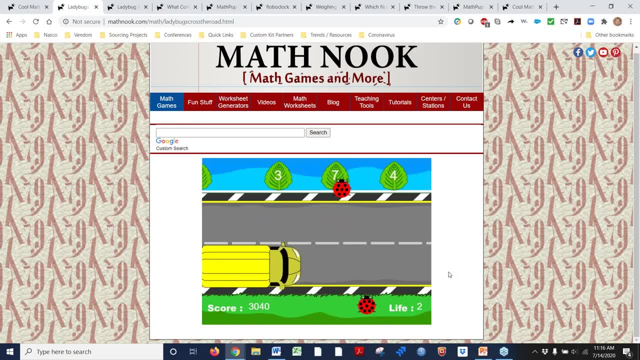 here. notice I'm in the water but I didn't fall in. this is known as a glitch, because if I go up here and I come down what, I fall into water. so this is a glitch. because if I go up here and I come down what, I fall into water. so this is a glitch. 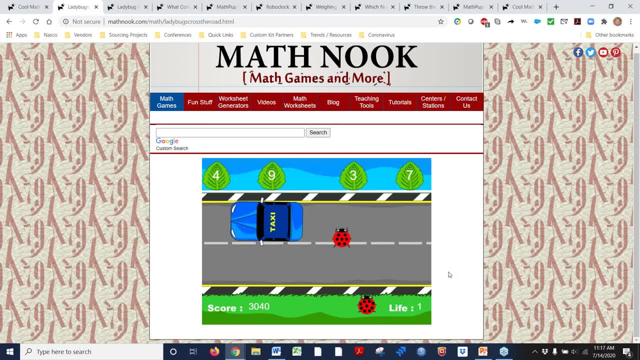 this. this is something that students can find. so, theoretically, students can actually cheat at this game based on this glitch, and so I can come up here, um, and I'll do that, but then I'll. I'll just wanted to kind of show you that, because, students, regardless of what games you play, if there's a 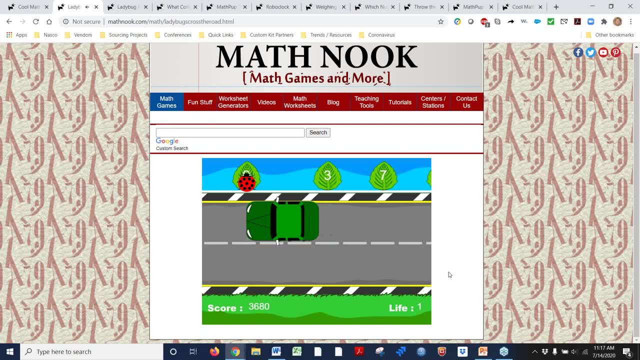 glitch in the game. oftentimes they are going to find it, so that's just something to be aware of whenever you're playing games. so, again, this is an easy counting game that you can use for kindergarten level. make it interactive. but again, if you can find a glitch in a game, um, you can make the difficulty a little bit easier. now notice, I won't. 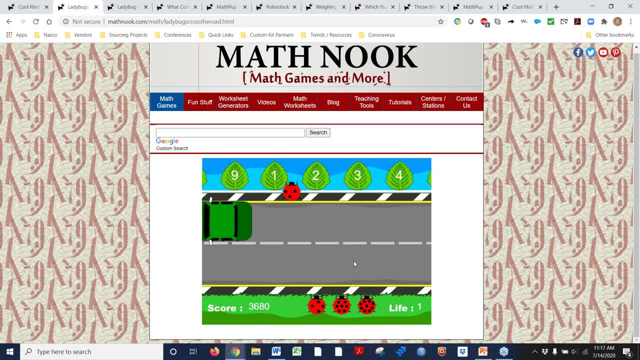 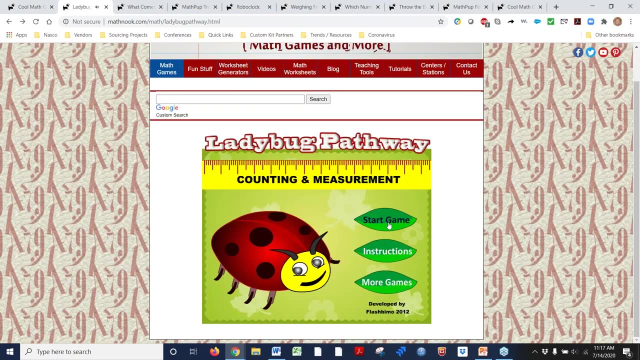 get hit by the vehicle, um, but yet I I'm not falling in the water either. so this is the easy way, but this is just something just to be aware of that you can play for um the kindergarten level, and so you can play it again, Etc, um. the next one we're going to be focusing on is ladybug pathway, so 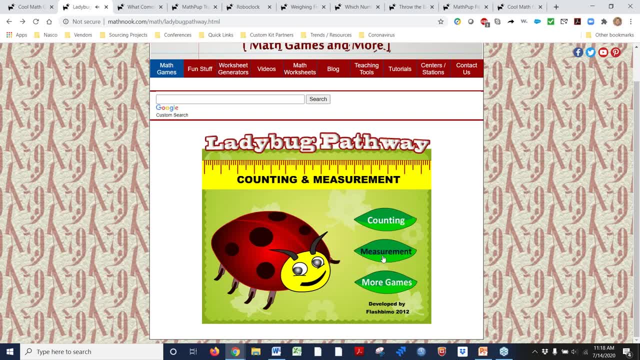 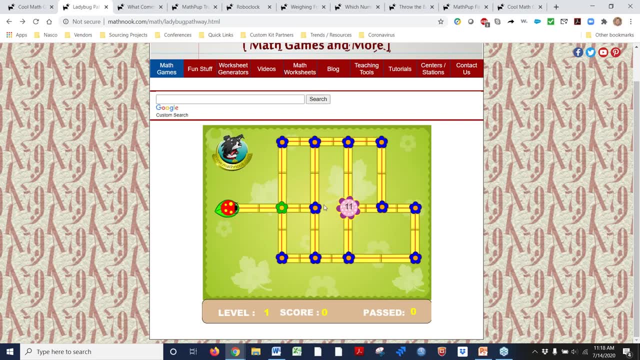 we're going to be starting a game. there's two different versions. there's counting and there's measurement. um, so if we go to counting, what this is doing is saying that, hey, we have to have X amount of paths, or uh that, to actually reach this flower. so if notice that the green highlights where we 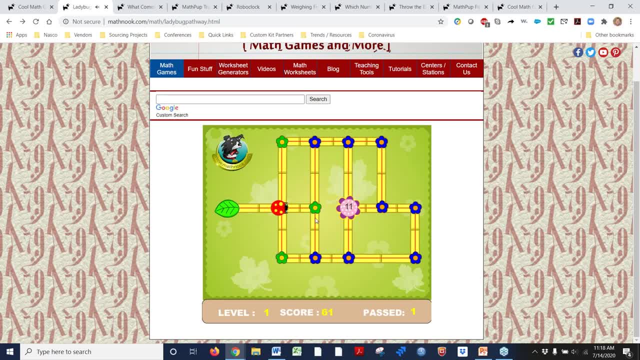 can actually go with throughout this game. now I have a different options here. now, if I want to go straight, I can still go straight. now I have two different other options and notice that, um, as I'm going this, my score is going up, but also how many moves I'm taking as well. so, as I'm 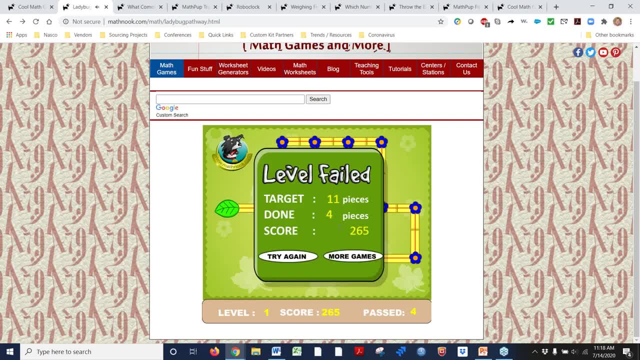 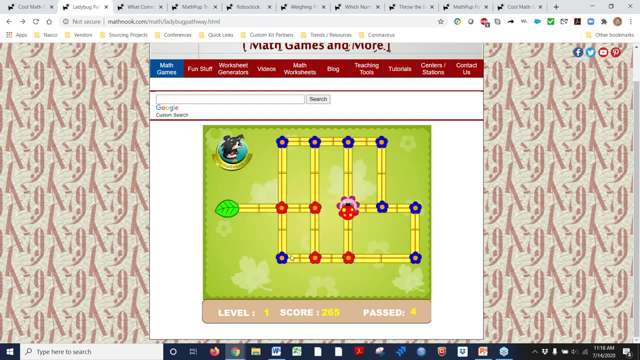 going this way, notice that if I come back up here that oh wait a minute, I failed, right. so Target is 11 pieces, but I've done it. I did it in four. so even though I thought I solved this problem, I actually did- I didn't take the appropriate number of steps to be able to do this. so then I would go. 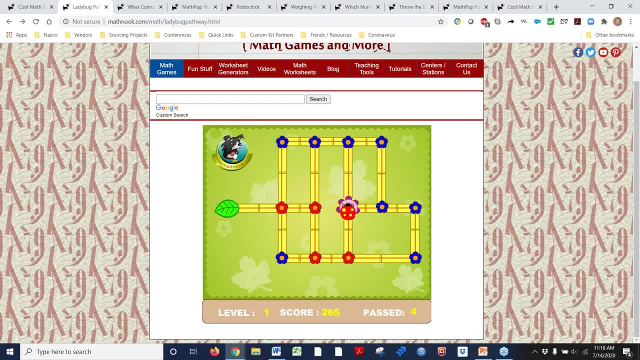 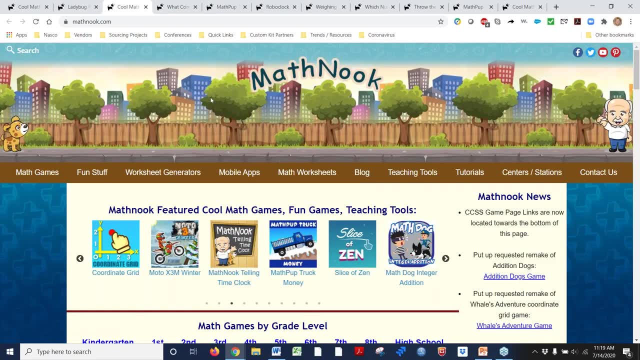 and try it again. right, and then we'd be able to reset. um, so then if you go back to into the game as well, um, so you notice as well. this is one of the errors that I don't like is that if you're done the game, you click it, it jumps you automatically out of the game. so even though you send the 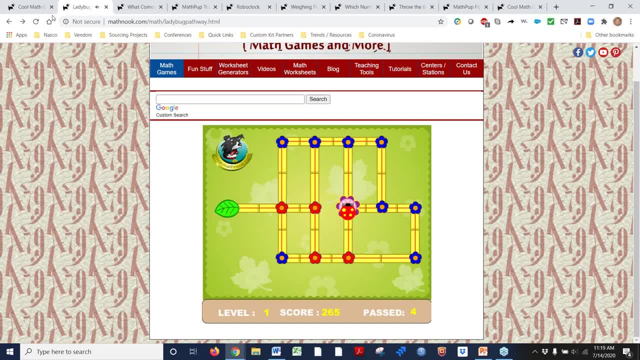 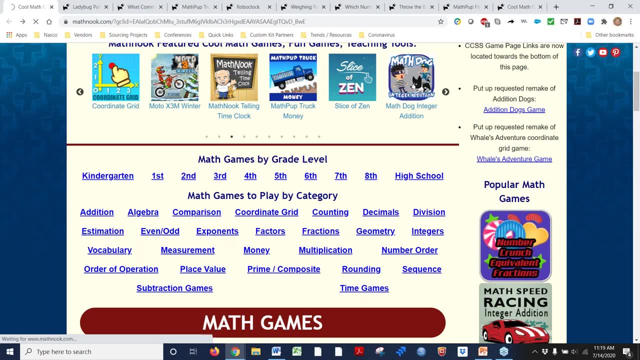 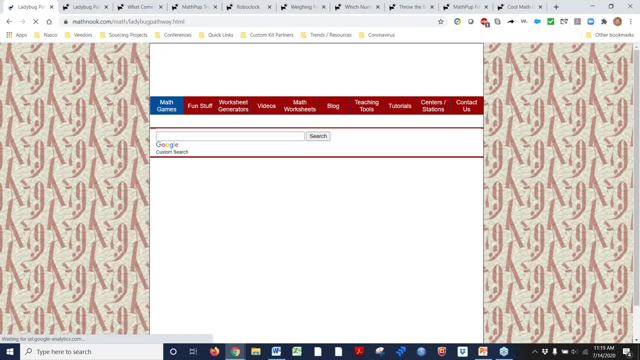 students the link to it. it does push you back out of the game. so if we go back into the um kindergarten level, we'd have to go right back down into um, the actual game again, counting the ladybugs pathway um, just to be able to start this up again. so this is this is something just to be. 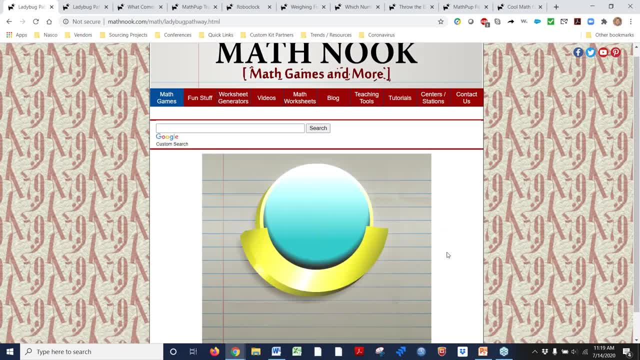 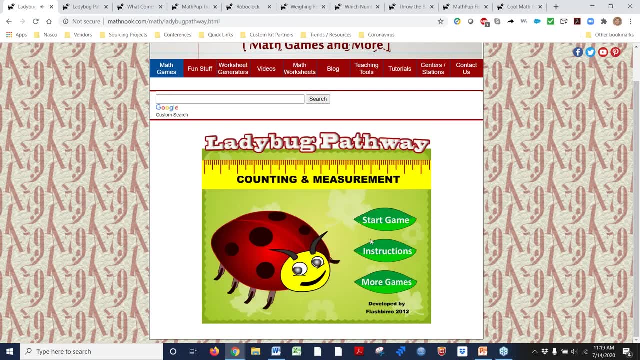 aware of. whenever using free content, you'll also notice that sometimes there's more ads and other things. commentary on free content: that's the other thing that usually you have to kind of worry about. so if we start the game, we do measurement. this is a little bit different in the fact that now we can 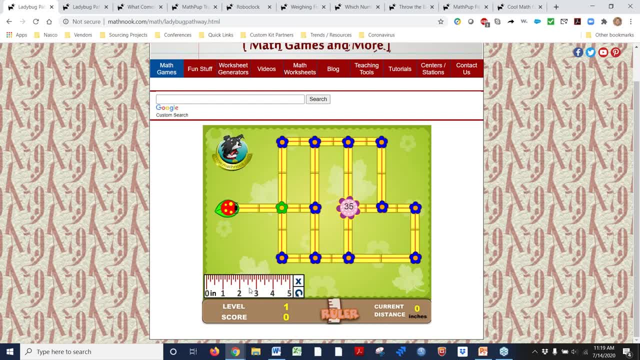 use a ruler. now we have to use 35 inches, meaning that from our start to beginning, how many inches are we actually using? you can use a ruler here. so we know if we take this path, that's five inches. well then, if we took a different path up, how many inches is there right, and then you can start. 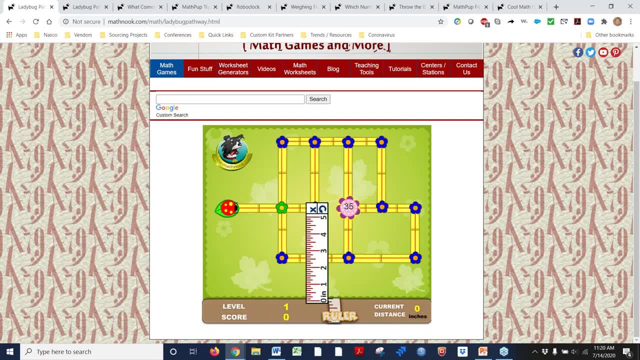 adding this up so that by the time we get there we know before we even begin where we should be able to go to be able to equal that distance. now we currently did three inches right. so we can do this two ways. we can do it where we can just kind of estimate, or we can use it where we're actually using a ruler. 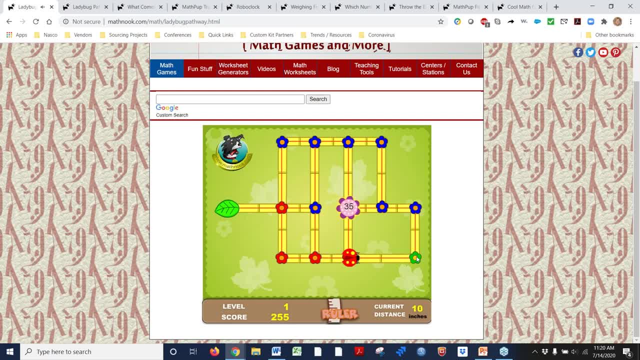 throughout this process. now notice that, oh, I'm only at 10, so I have to keep going and just to be able to reach my goal of 35 inches, and so I'm just kind of quickly going through here. now I'm at 25, so, notice, I didn't measure where to go, so now I'm thinking that, oh, wait a minute, do I? 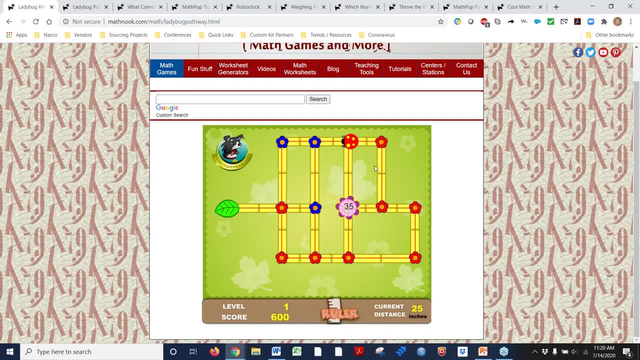 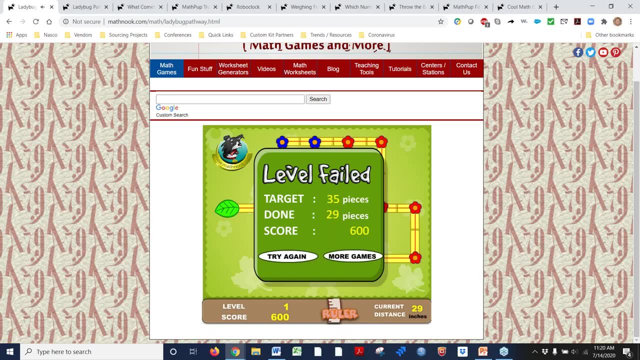 I, I can't go this way now because it's not highlighted. so notice that I can only take one pass. so when I come back down here, I notice that, oh well, you know what? I only got 29 pieces, and that's the reason why we use a ruler thing. so again, using measurement and incorporating into the 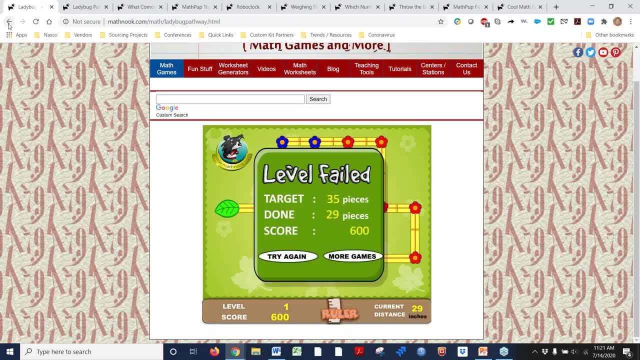 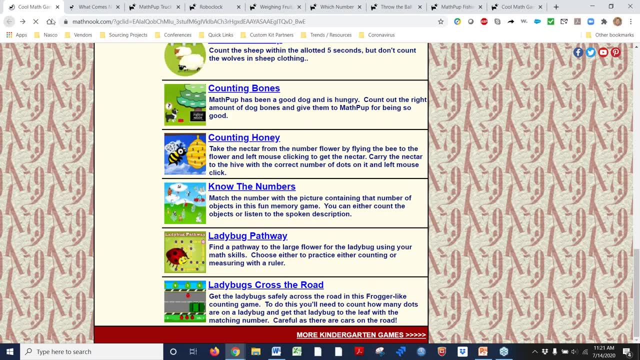 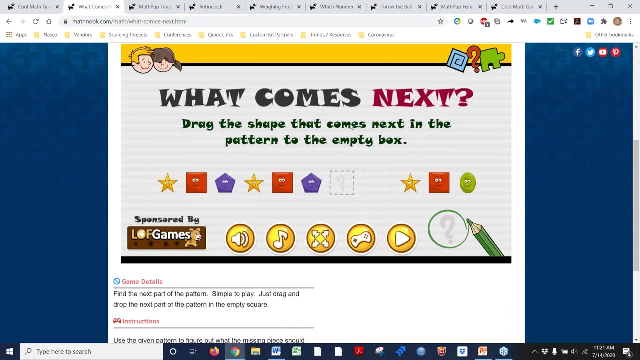 class. so that is our ladybug um game that we have there. okay, um, for first grade. um, oh sorry, I didn't want me to go back there. I like to go back to begin, just in case. so this is the other one, so we, we can start the game. um, this is based on what comes next. it's based on patterns. 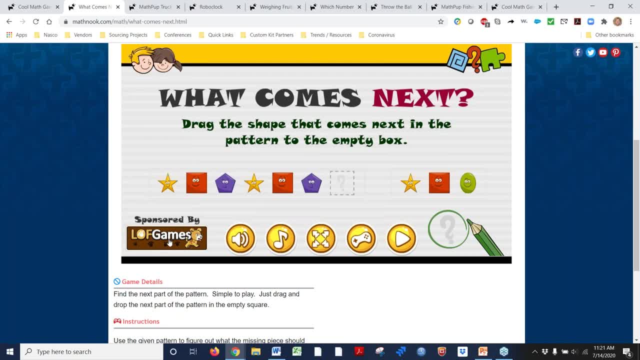 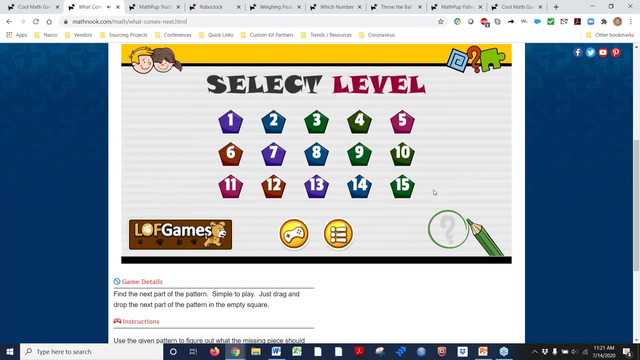 other things here is: this can take you off site. so this is sponsored by. so if you click here, it takes you off site. you can change the volume, other different aspects, so this is something be aware of. There's 15 levels. Each level gives you X amount of points, up to 60 points, And so. 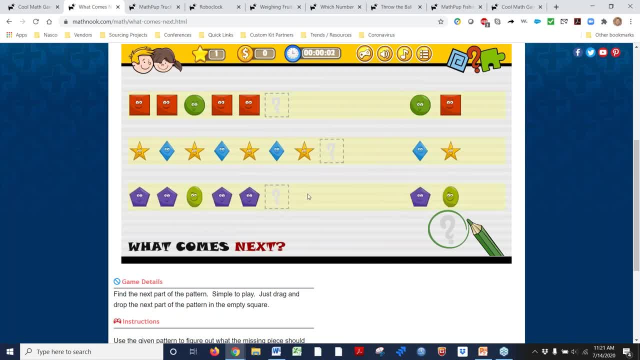 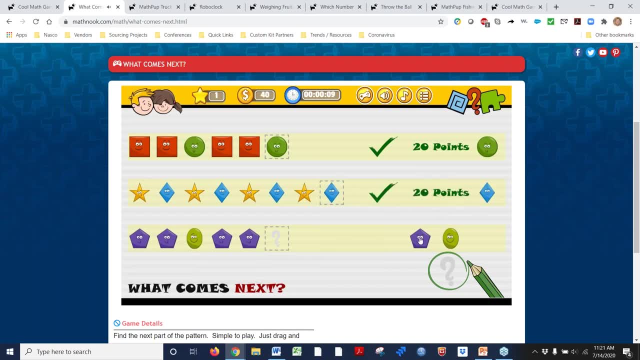 there's a total of 900 points that you can use, but it starts at the very beginning. you know what comes next, right? So different shapes, different sizes. Notice I get points for correct answers. If I were to use an incorrect answer, I lose five points. So at the very end, 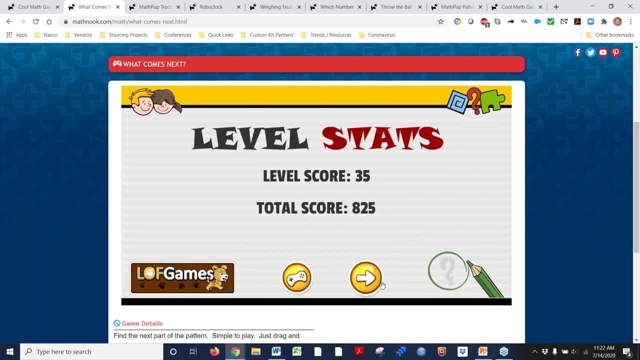 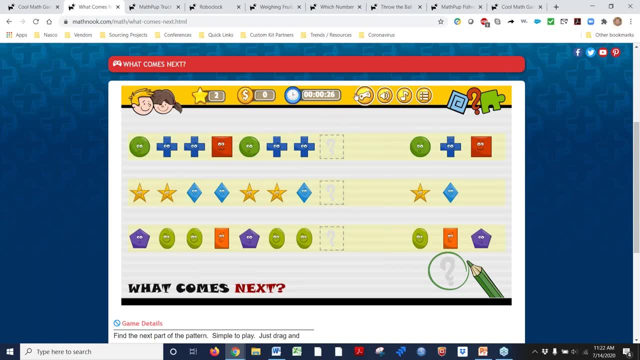 again, this could tell you total score. So I actually played this game earlier. So it's actually keeping track of all that. So that's the other thing. Once you play it, since it's free- it does keep track of everything because it's browser-based. This also keeps track of time. So 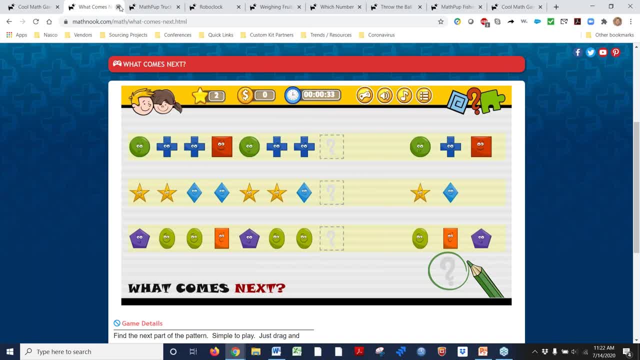 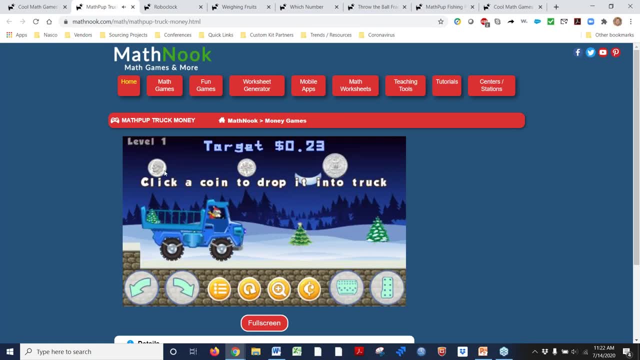 depending on how fast you level up, you can keep track of that. So that's like a first grade version Math pickup truck. This is a easy one, where you can click on coins and you get to the very. your target is 23 cents. So if I were to keep clicking here and notice that the coins are, 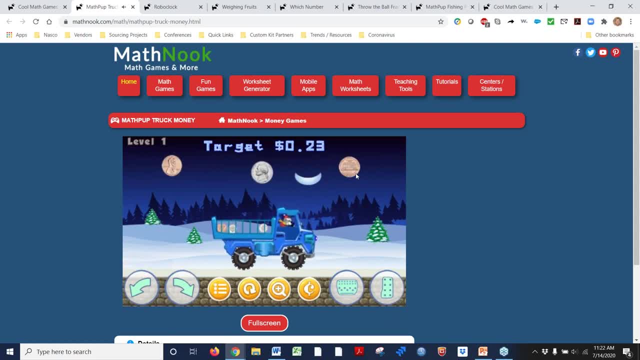 moving and they can fall out based on this. So if I go in too fast or if I'm going too slow, I don't. I can speed up, I can turn, I can make a little more. So it's a little bit more engaging. but 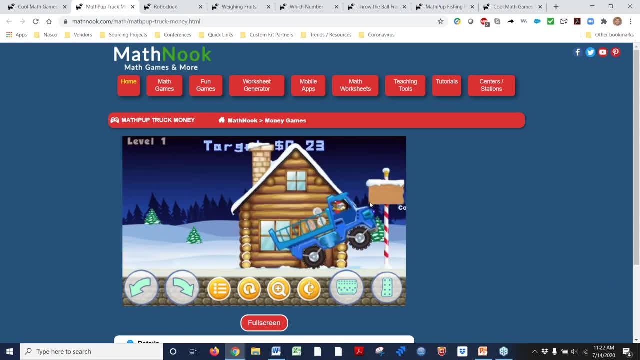 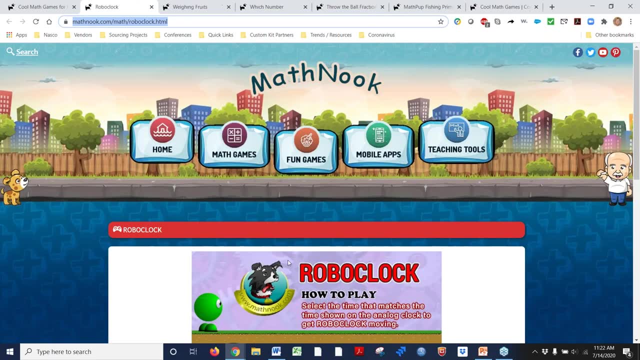 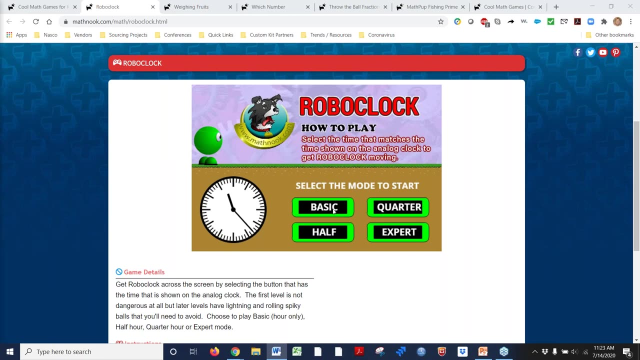 you're actually counting coins And at the very end it actually counts up all of your various coins to see if you're correct or not. So again, a nice little easy game that you can use there: Roboclock. This is teaching time, So we're getting into third grade now a little bit. So 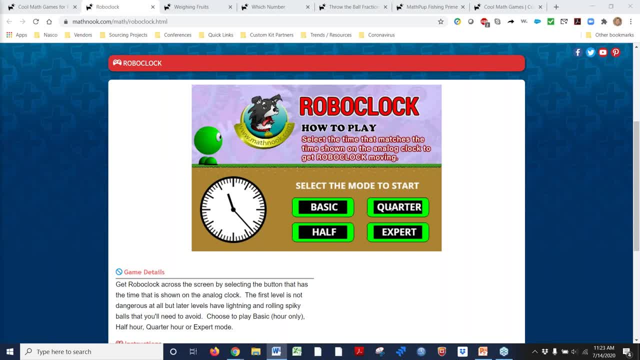 basic is based on the hour, half is using half hours, quarters, quarter two, and then expert is all of the above. So when we're looking at this, okay, what is nine o'clock here? Okay, so then we keep moving. What is this? nine o'clock, four o'clock, What is this? And you keep moving through. 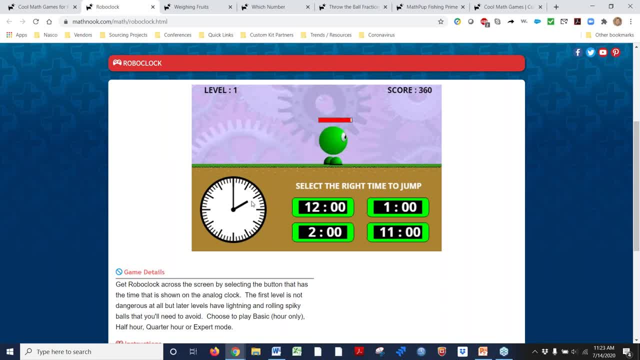 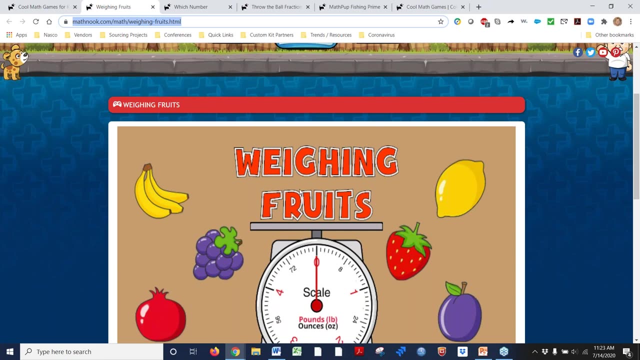 it And it will kind of switch it up over time. It's not am or pm, but it gets students start to think about and recognize different clocks to be able to move throughout this whole process. So level up, keep going and then you'll keep track of your score. A nice little easy game Here's. 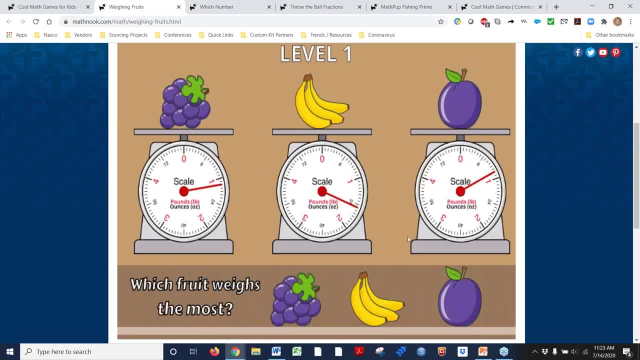 weighing fruits. You can get into like fourth grade a little bit. This is a great one because it talks about fruit recognizing this, You can say, okay, what is this So for ELL students, if you talk about that, but then also reading scales: how do we read scales and weight These? 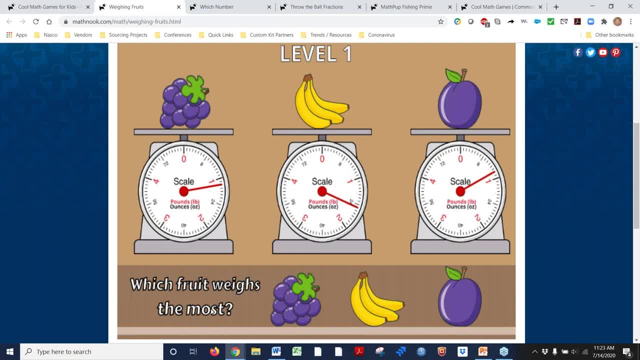 are pounds and ounces, right. So, looking at this, which fruit weighs the most? So the grape is here, the bananas here, the plums there. the grapes here, the bananas here, the plums there, the plums there. 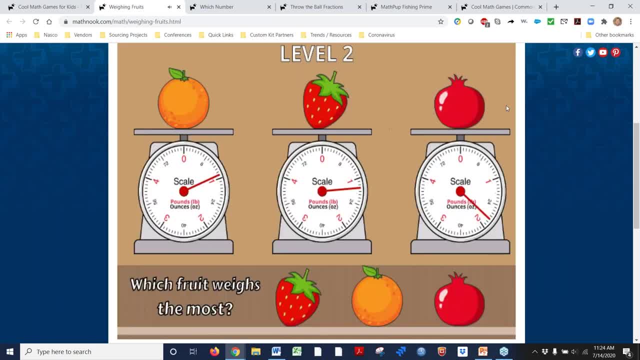 we know that the banana is the heaviest weight. Same thing here, tomato, But then as you start leveling up now we start to use multiple fruits. So if we know the strawberry weighs this much, and with the plum on it now it weighs this much, which is the heaviest, So we know that this is. 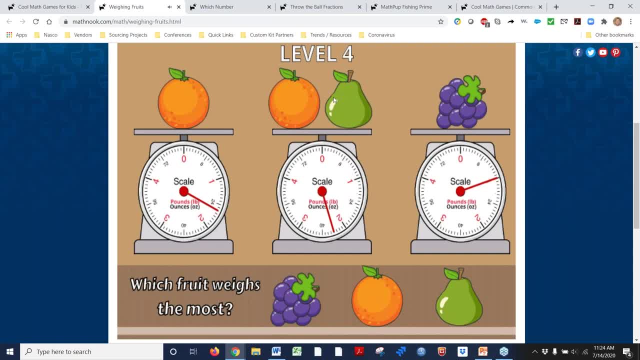 only a fraction of what an apple would weigh. So these are again getting into a little bit more complex narratives for the students to be able to solve, but it's an easy way for them to kind of use some measurements. So if you look at this, you can see that there's a number of different. 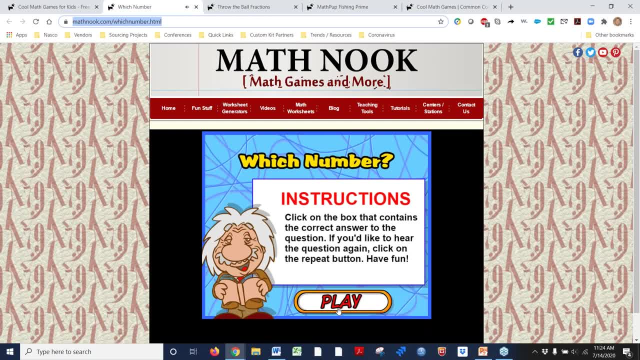 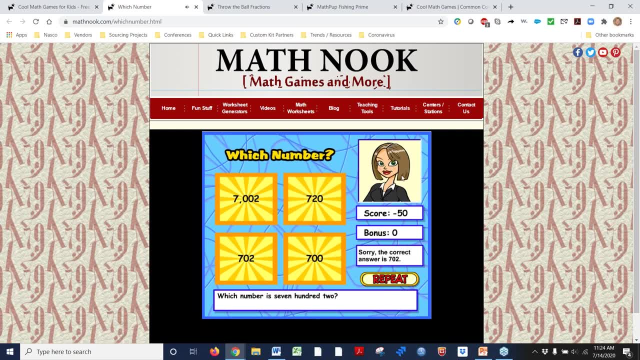 numbers. even when you look at this Again, it's actually going to give you some guidance towards reading historic environment in Google that you can actually see how that number is, ум, which number. So this game is another game that talks out loud, that says the number. 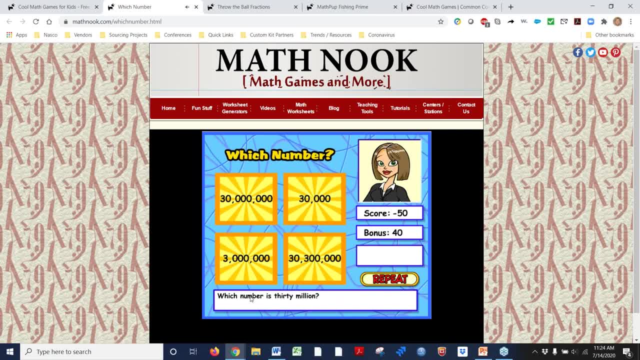 It'll tell you. sorry if it's incorrect. You can't hear the volume, but for me I can. So if you need them to repeat, number is 30 million. So it's written and it's also ready there. So, oh, hey, and then you get a bonus too for the correct answers. So again, ELL students. easy to be able to interact with each of those different stages in for differentipe. so Mona 말씀드�hat, they're not still so familiar from the prosperity ياomayan. in surprise to you, though, we all have an old on-site Tactical Impact Trip, so it's not too long. These are gonna be. 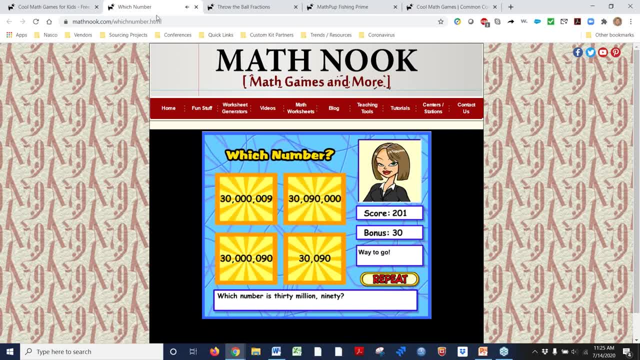 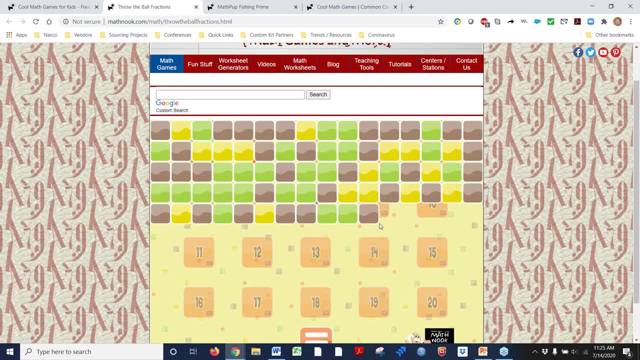 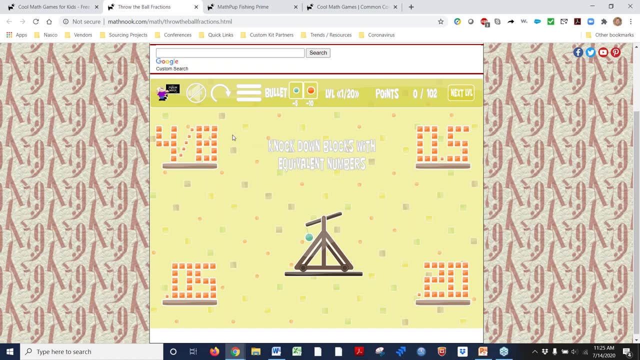 the each of those different tasks that you have, but another easy math activity. Then you have throw the ball, fractions. So this is an interesting game. I thought there's a little bit of complexity as far as skill, and then also equivalent fractions. So looking at this screen, there's two equivalent. 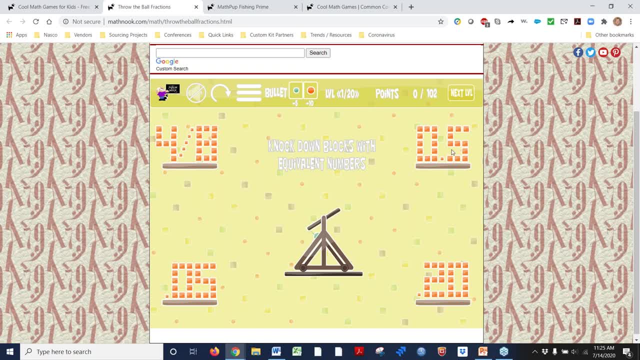 fractions that we have. We have four eighths and we had five tenths. Those are equivalent to one another. So what you want to do is knock down the block. So you hold the left clicker and then you would throw the ball to see if you can actually knock over. And I, like I said, this is something. 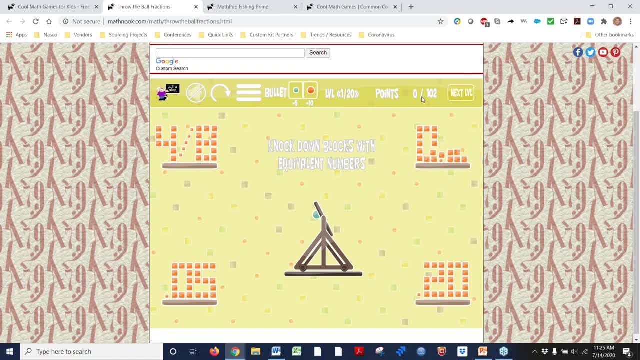 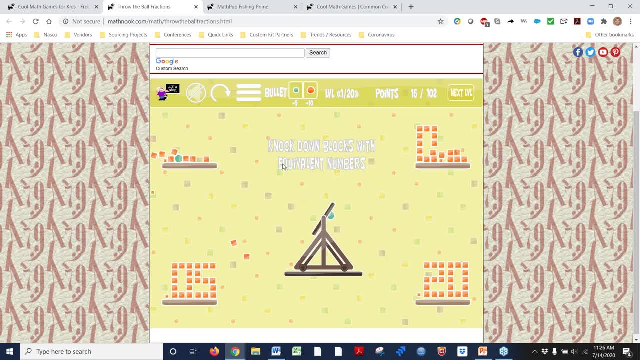 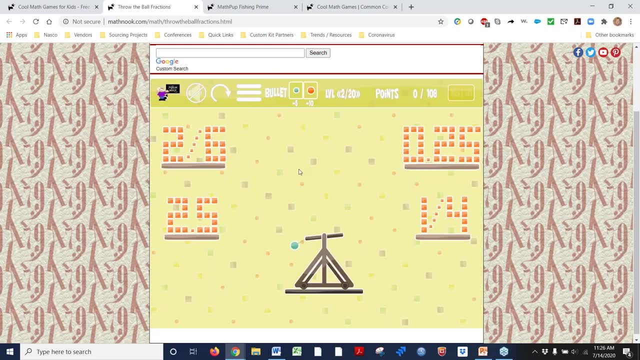 you'll notice, you'll swing over to the other side to be able to go and get all the points you need. So I am able to go to the next level. But again, recognizing equivalent fractions is something a little bit different for students to be able to use. You got prime numbers, So this is an easy. 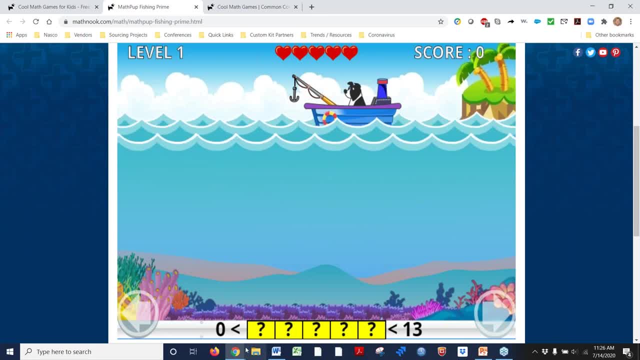 way for you to move back and forth in a boat and understand, okay, what are the different prime numbers here between zero and two? So if I lower down the hook and actually grab a fish, what numbers am I grabbing? And is it a prime number or not? Okay, Yep, So we know that's a prime. 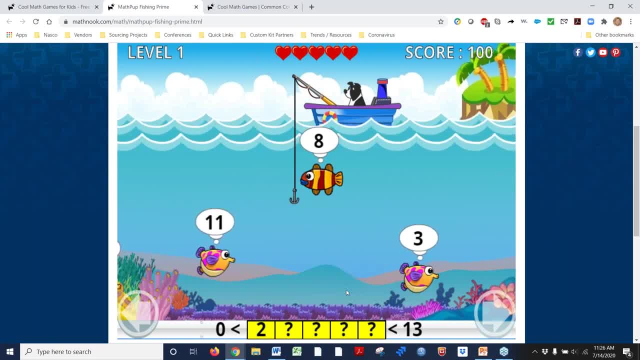 number. So what are some other prime numbers that we have? Oh well, that's a composite number, Right? So now let's look at some other numbers. Okay, It was seven prime. Yep, There you go, There's a prime number. So then we have all these different numbers here, We have a score, We have a life. 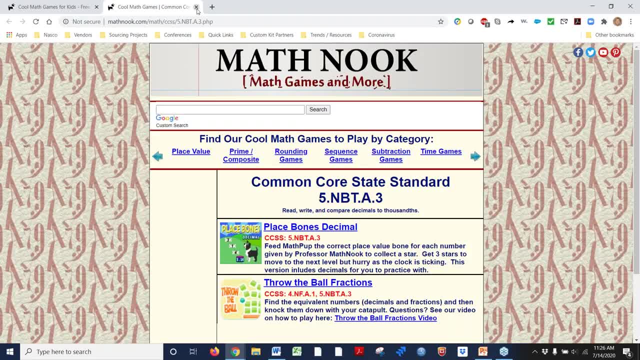 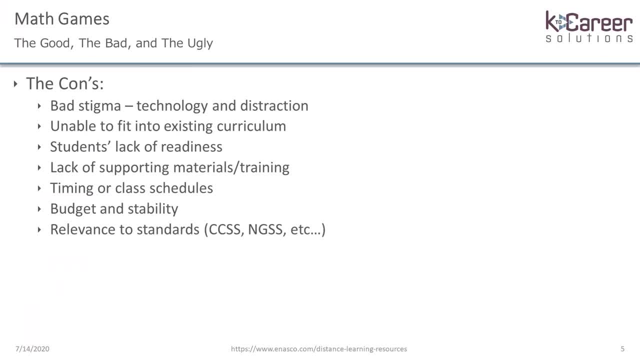 Just again another interactive game that they could be using For that, And that's essentially what math nook is. So if we're looking back on to this right here- math nook- I give you links again to all the different games that we played here. I kind of went. 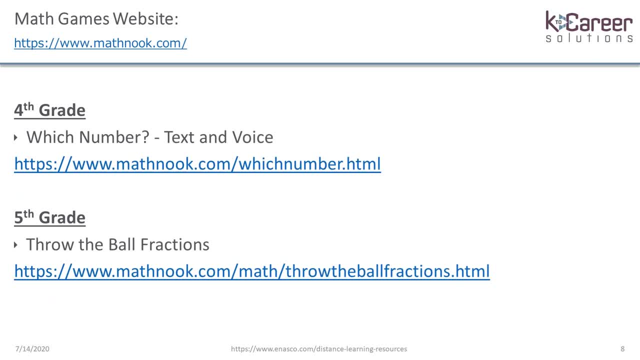 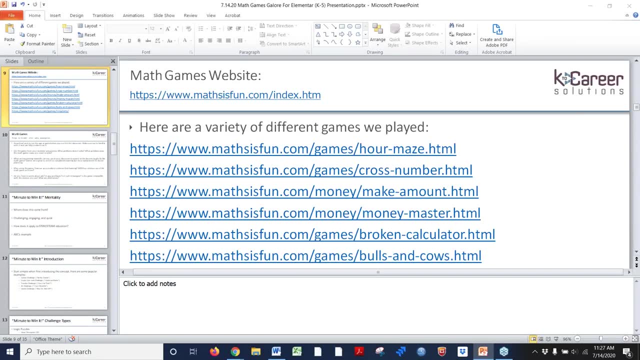 through them rather quickly, But these are ways that you can use different math games. Okay, So the next one that we're going to be able to use right now is: math is fun. This is kind of a nice I thought is like interactive puzzles. I'm a big believer in problem solving and using 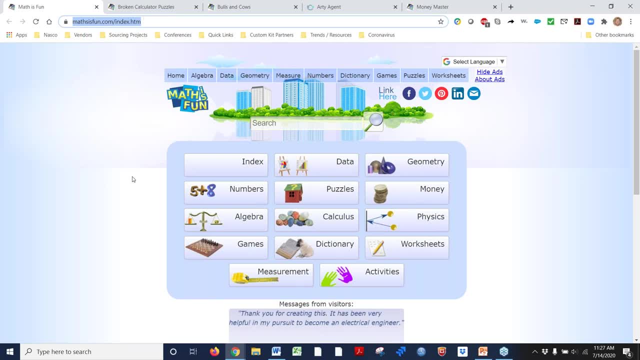 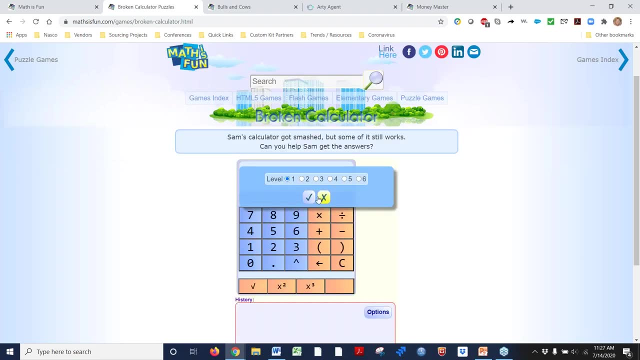 critical thinking and problem solving. So math is fun. This is the main website that you would have here, broken up into different areas. You can search the different games. So I I like this because it's a great way for students to start thinking about ways they can use calculators and how the functions. 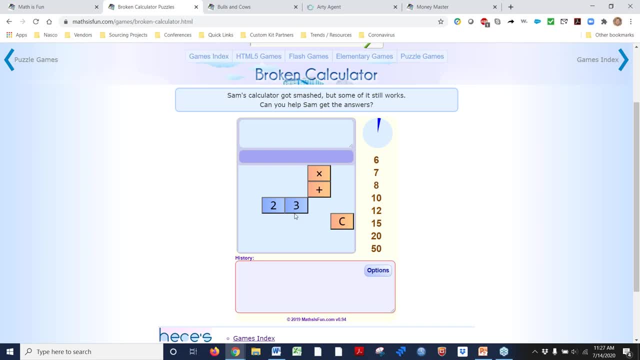 So right now, these are the only functions that we have available to assign calculator, and we have to actually make these numbers happen. So in order to do this six, well, maybe we want to do 3 plus 3.. Oh, that's six. 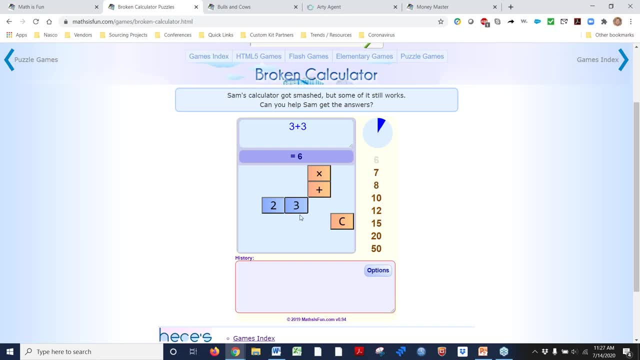 Okay, We got that And notice we're getting time during this. Okay, How do we make seven? Well, maybe we do. you know, two plus two plus three, Well, that equals 40. Well, that doesn't work. 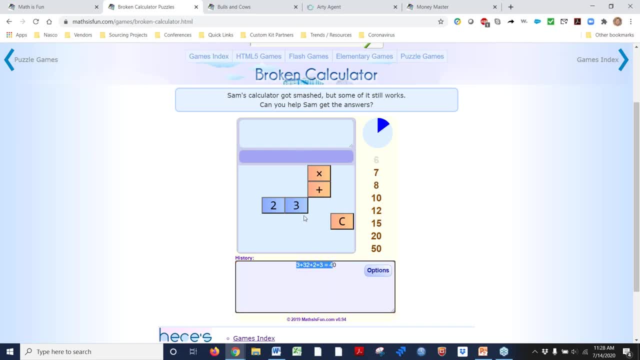 All right. So now we have to reset. So notice that this kept on from our old answer. So we have to make sure if we're resetting, how does that work? And the reason why we want to keep that in mind is because there's a way- strategies- to be able to use this. So notice, I got seven. 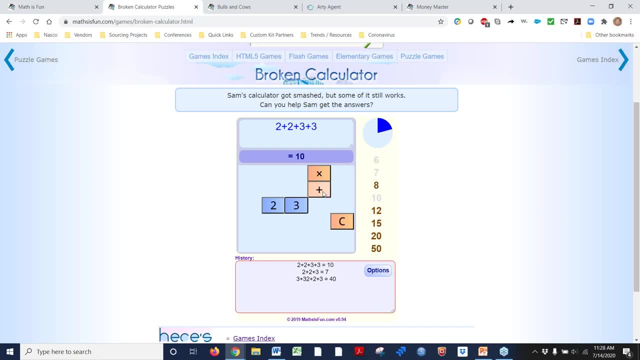 right? So if we did plus three now we got 10.. And if we did plus two, we got 12.. Then we did plus three, then we got 15.. Then if we did plus three, plus two, then we got 20.. And if we add: 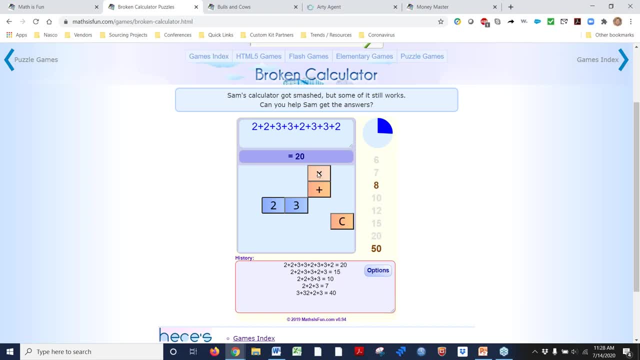 them all up. we eventually get all of these. So there's different ways And you can ask students: well, can you use multiplication to get this? If so, where? if you can use addition, how do you use that to equal these numbers? So there's a lot of different ways you can use. 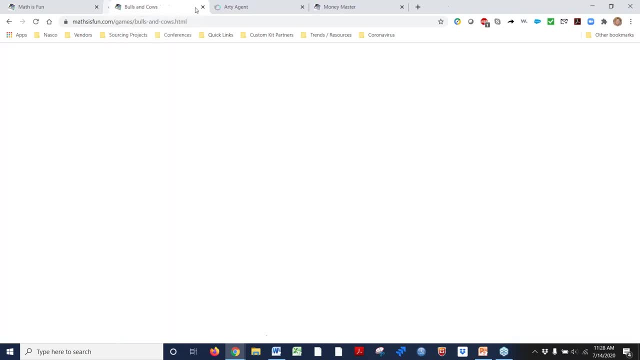 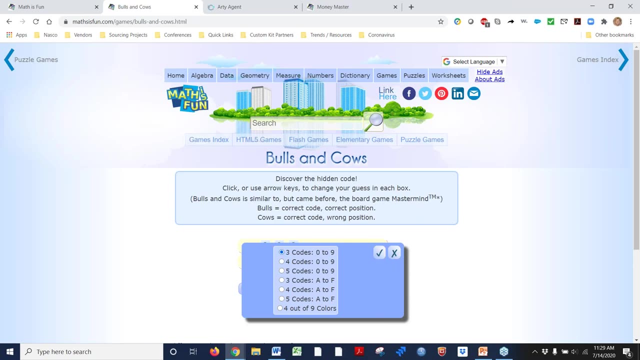 broken calculator And it's a fun way to have a little twist on a traditional calculator. So if you did plus three now, we got 10.. And if we did plus two now, we got 12.. Bulls and cows. This is a fun activity. that it's, you know, based. it just kind of came up before. 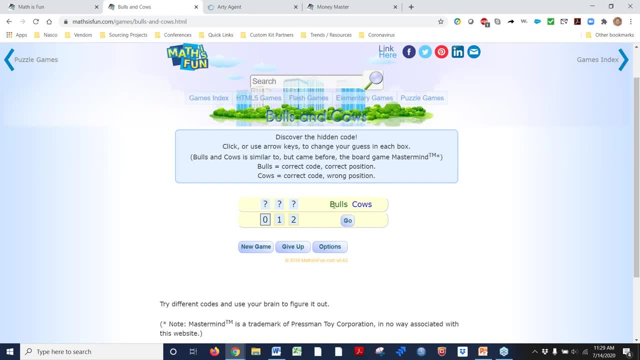 mastermind, but it's on that same principle. So right here, bulls are true, cows are false. So if I had numbers here, one, two and three, if we say go, we know one is true. So if I change this, 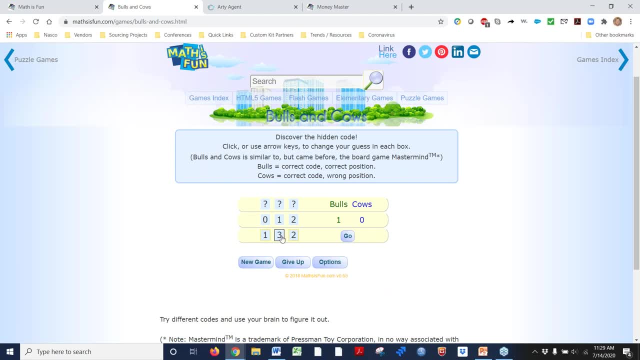 to one. I change this to three. you can have repeated numbers. We now that, know that two are false. So we know that this wasn't correct to begin with. And if we did plus two now we got five. It was one of the zero, or the one that we needed to be able to use to be able to go. So we 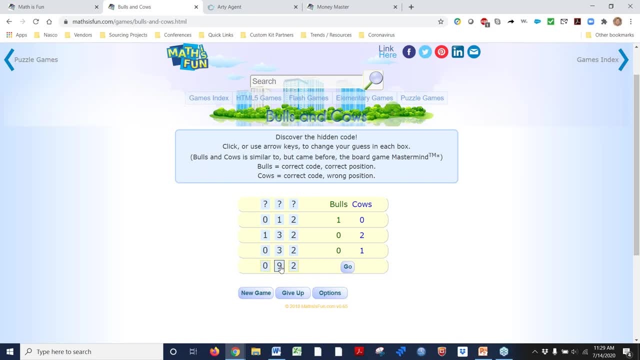 know that now that isn't correct. So we know that one, based on that information, is correct. This one and this other one are the ones that are incorrect. So if we go there now we know one one. So if we go three and four, now we know two is correct. Well, maybe let's see if this is correct. Oh, 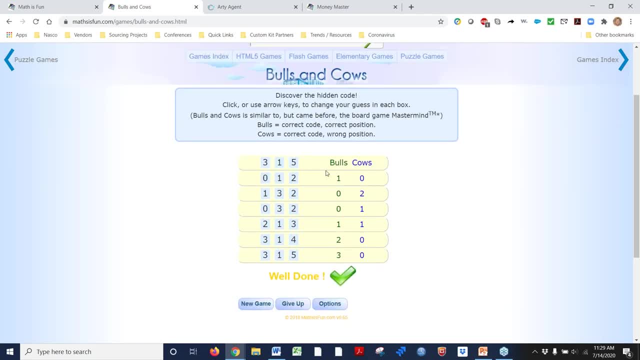 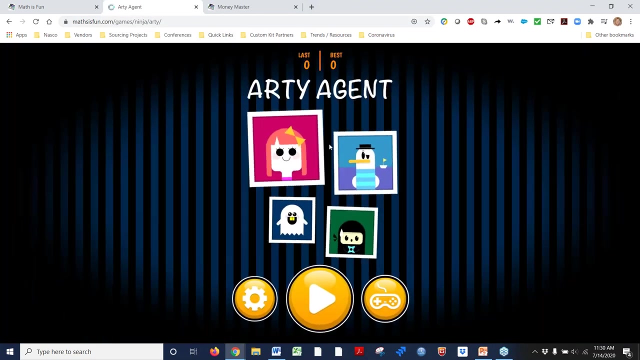 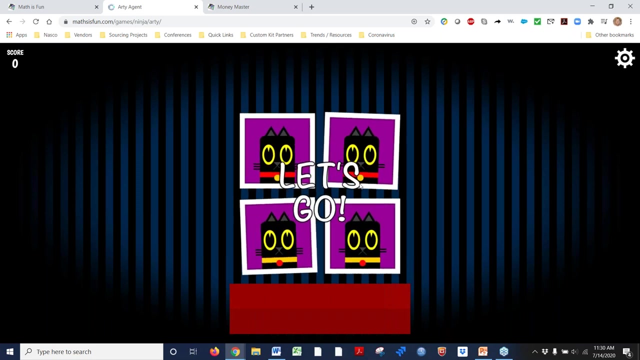 look at that Now. we did well done. So this is another easy way to be able to. what we're going to do here is we're going to go back to that natural sort here Sometimes when you need to Pf plusieurs, So there's more information to. do than you need to do. So we're going to cut a lot of time off here. You can go ahead and go to the phone and look at that, But a lot of meet. So if we want to go through the three first without less than four, just a couple of. 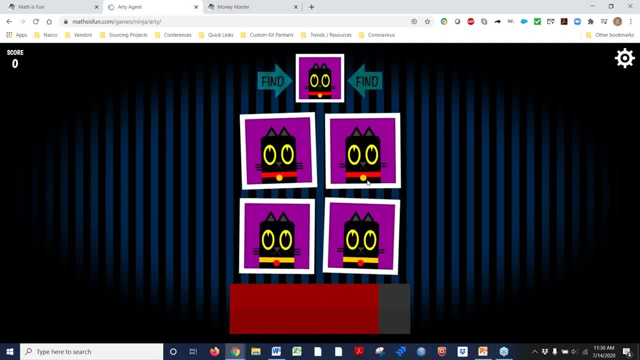 times to find the best alternative here. That's really the last thing is kind of strong with us at all. says: shift those numbers. all the want to find what is the one that looks exactly like this. so if you look, notice that these whiskers have three tags. this has two, so we know we've already eliminated two. now let's look at these. 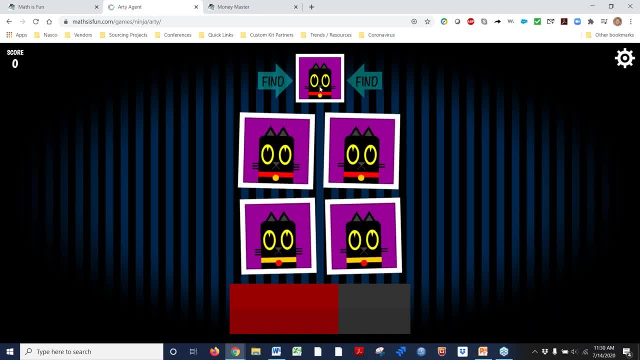 what are difference between these two? well, one's red, one's yellow. what is it? well, it's red, so we can click on there. so this is a great way for students to kind of look and focus on that, one kind of element that kind of differentiates it from the rest. now, in this case it's the eyebrows. 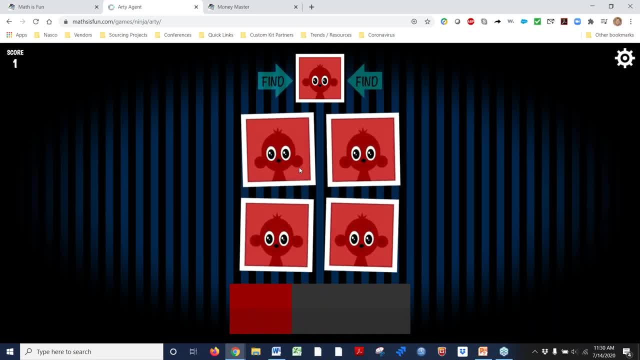 look at the eyebrows, look. so we know this is incorrect. and we also know that this is incorrect, so we know it's one of these two. so what's the difference between these two? one ears is drooping and ones is not, so we know that's correct. so this again, another way for students to start thinking. 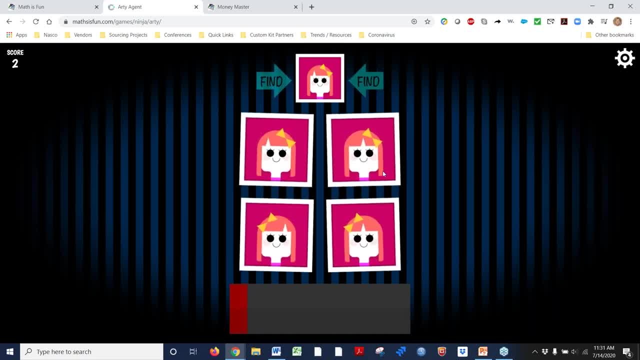 about symmetry and ways to differentiate, and then we could tie it into real world applications of forgery. how does this actually relate? in real world, there's people that actually look at these details. if you have difficulty during this time, there's people that are study this and have good eye. 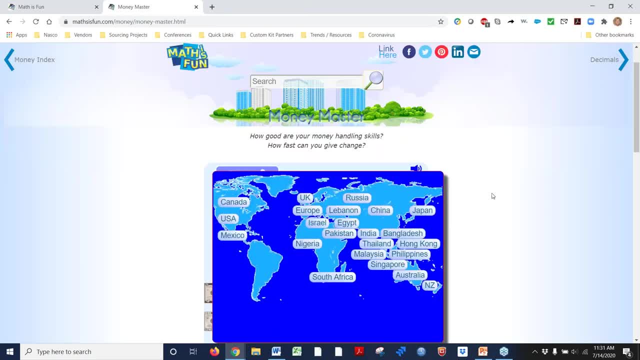 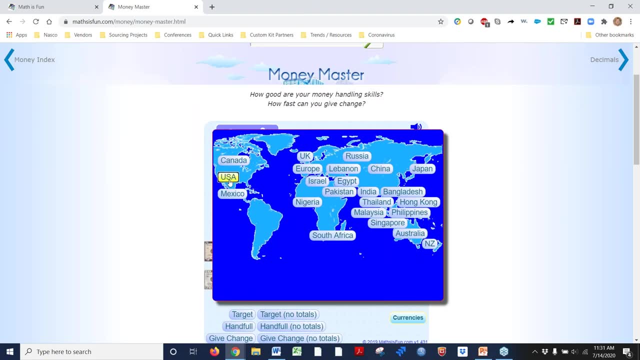 perception for that. um. another game that we have here is called money master. this is fun because i think it's a great way to be able to manipulate money in a unique way. so, for example, if we go to usa, your target change is 36. now, this is all the dollars that you can. 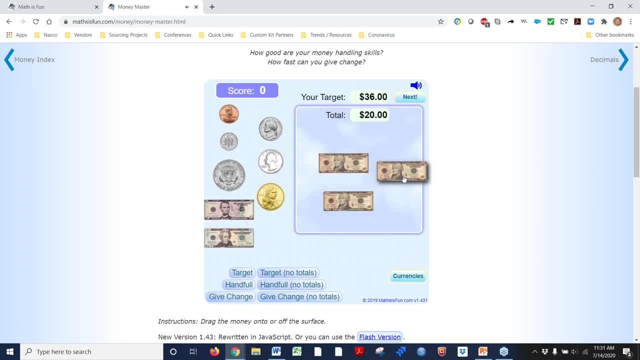 have. now you can. there's currently ways that you can add up um to this to see if we can actually get up to 36 dollars. okay, all right, so then we go to next. right, um, you can have a target with total, or you can have a target without totals, um, so so basically meaning that, as i'm going here, you can't. 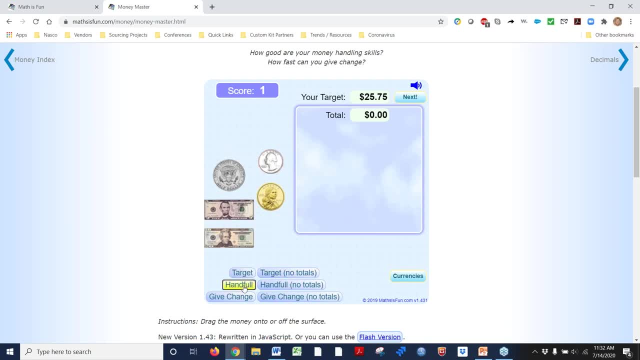 see how much this really is. so there's ways to make it more difficult. so there's handful and handful- no totals, and then if you give change, for example. so these are great ways to be able to use money master um, to be able to have this, to be able to manipulate coins, and there's also other. 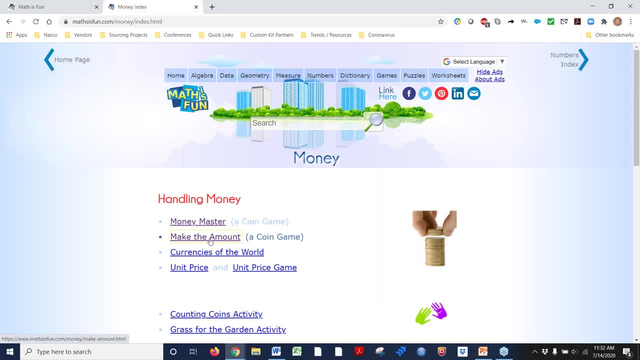 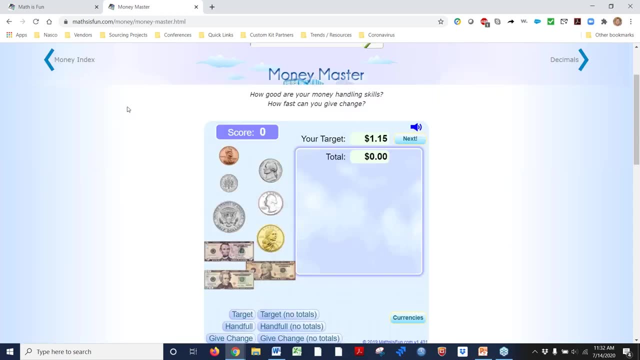 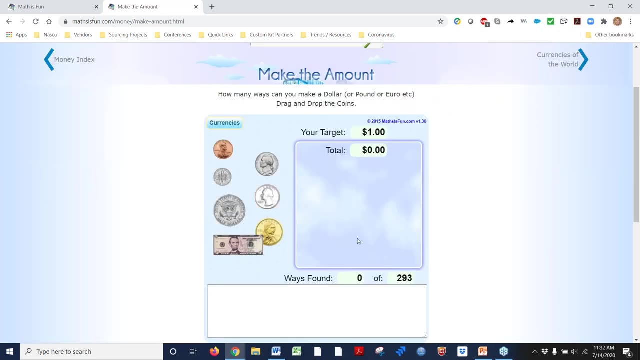 games on here, um, not just master index, um, but uh currencies of- i think it's this one that i'm looking for. uh, no, no, no, no, no, no, no, all right, okay. so this is a fun way to also think of different ways of using money. so 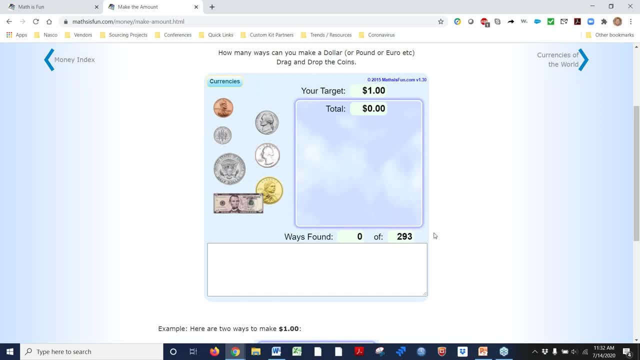 where target amount is one dollar, how many different ways can we find and make that one dollar? now, there's 293 ways um to make one dollar with the coins and the currency that we have over um. so if we looked at this, oh well, that's too much, right? so if we put this on there, yep, there's one. 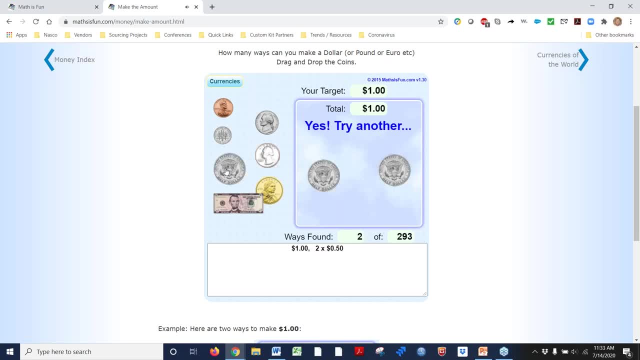 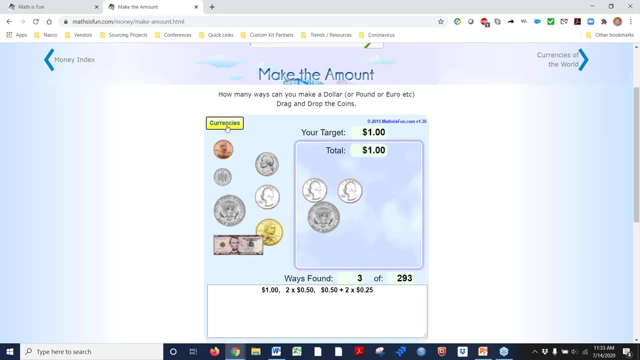 way, let's think of another way. so if we used four quarters, uh, or two half dollars, i mean, or then we use two quarters and a half dollar, that's three ways. so we can ask students to have maybe come up with like 10 ways, and then just write down all those possibilities and share those. what's also? 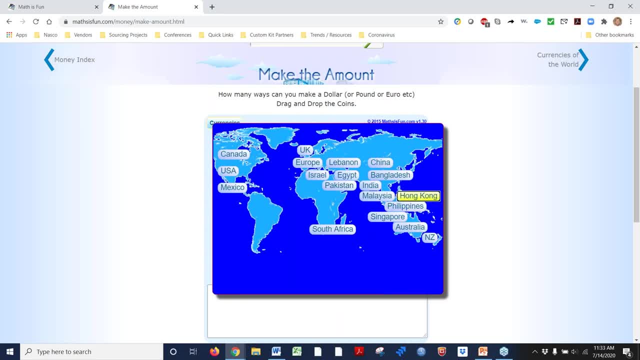 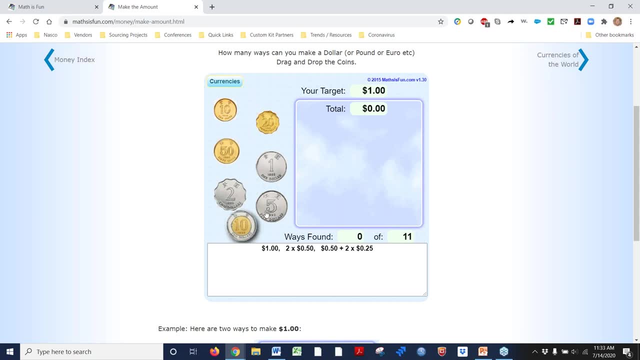 interesting, though, is we can actually have other countries currency too. so for like this one, for hong kong only has 11 ways to be able to make up one dollar, and if we look at this, oh, that's ten dollars. so, even though we don't know these currencies values, we can start to decide. oh. 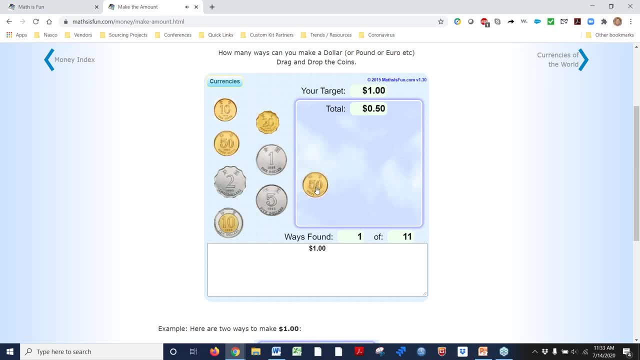 well, these are ways that we can actually start building these. so the second way would be: you know, build 50. okay, so now we use two 50s. now let's build it with just 20s and 50s, all right, so that's all the possibility there. so then we get into. okay, so now we've used all the 50s. 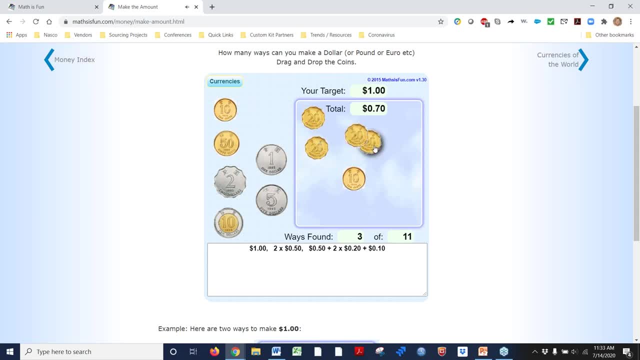 all right, so now we've used all the 50s are, so now let's substitute it with all the 20s. um, all right, okay, and then if we took off a 20, let's add a 10 and a 10 for that, okay. well then. 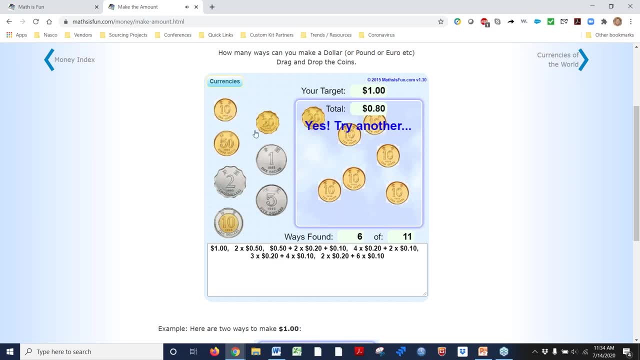 we take it off, and so you can see how i'm kind of logically thinking throughout this whole process. but this is a great way for um students to be able to work through some of these different problems, right, um? so this is not all the different strategies, so now i look i've only 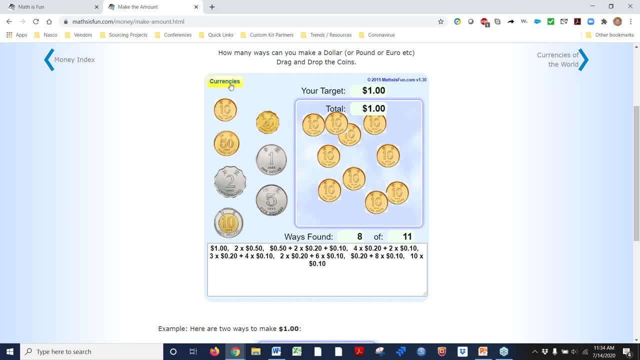 had 8 out of 11.. so where did i go? wrong, right, and then we can go back to that. so the hong kong would be a great one for students to see if they can get all of them. but then in the usa, maybe come up with maybe 10 to 20 different ways or depending on the 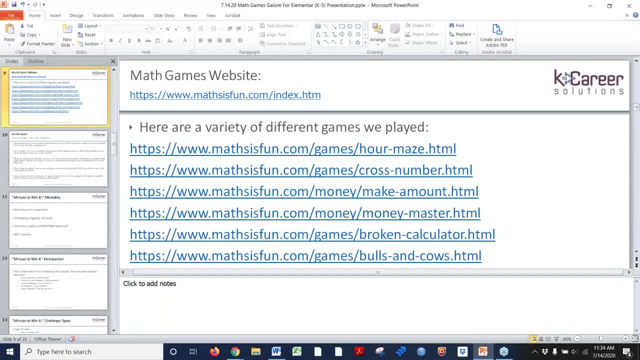 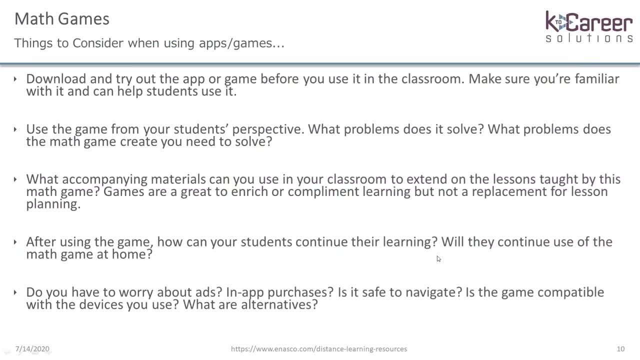 level of your students to be able to use that. so again, math games are great ways to be able to use, and here's a couple of some different links that you can use for that. so, when you're using them, things to consider. you want to download and try to use an app or 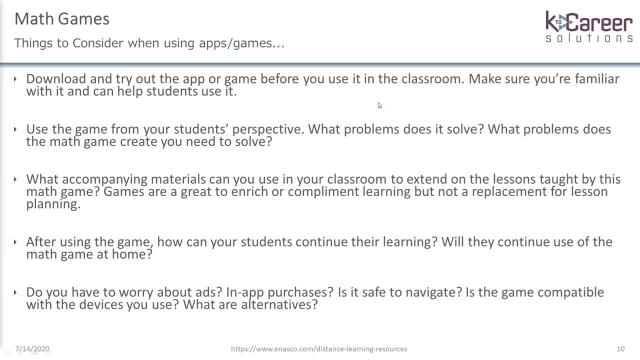 game before using the classroom, just to make sure you're familiar with it. You want to take it from your students' perspective to see what they see. you know what kind of problem it solves. what's the things they kind of create when you need to solve what accompanying materials can? 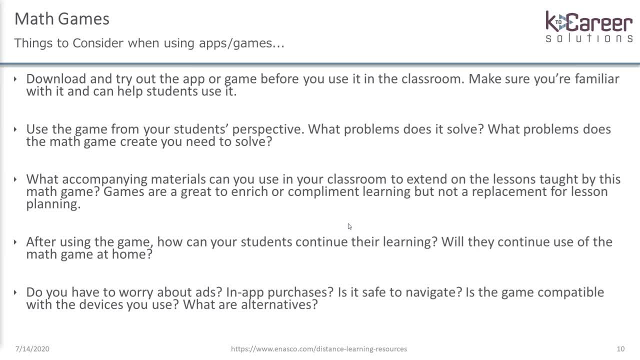 you use in the classroom to extend on the lessons taught by this math game. Games are great to enrich or complement learning, but remember it's not to replace the lesson. And then, after using the game, you know how can your students continue learning, Whether they could continue to use the game at. 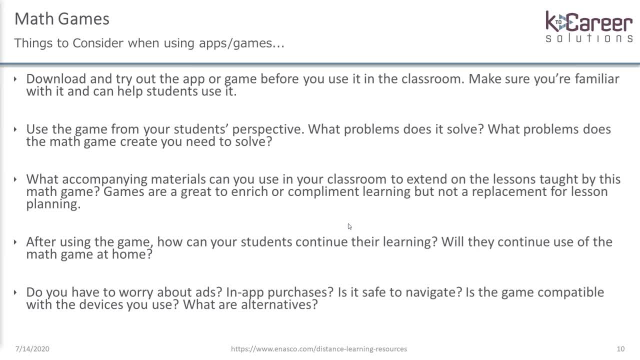 home. is it pretty repetitive? Is it going to be able to, you know, be able to use over and over again? So, and then the last thing is: do you have to worry about ads in-app purchases? Is it safe? 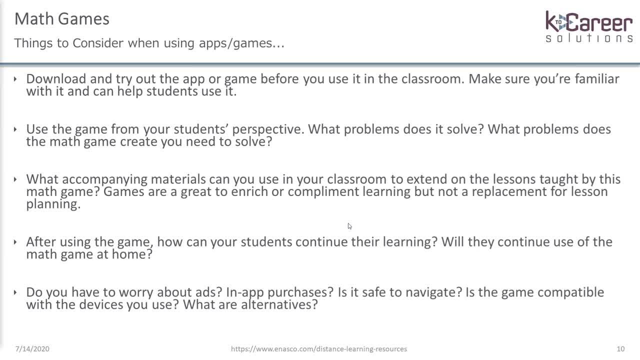 to navigate? Is the game compatible with the devices you use? What are alternatives? So the sites that I gave you, some of them do have ads. Some of them are hard to navigate. So, although you can give them the link, students can get out of the link really easily and start navigating. 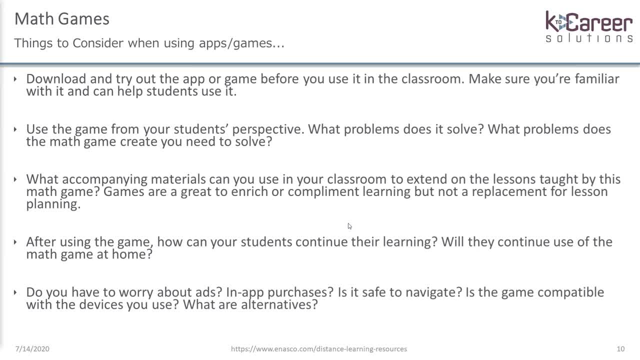 all over the place, right? So you want to really make sure that students if you're using something that you understand. there are limitations to sometimes using free resources, But these are again great ways that you can use different games and apps throughout. 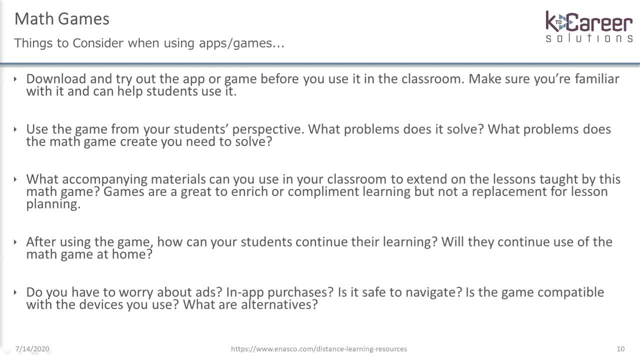 these And these are more of guidelines that get you thinking about what's important When you ask yourself these kind of questions when trying out new games for your classroom. it can help you assess whether games or apps are a good fit for your classroom needs and if the app will continue. 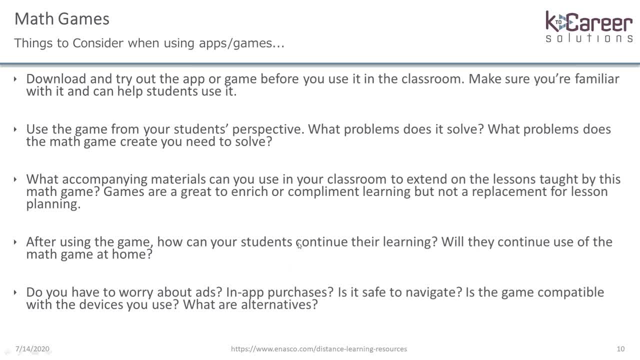 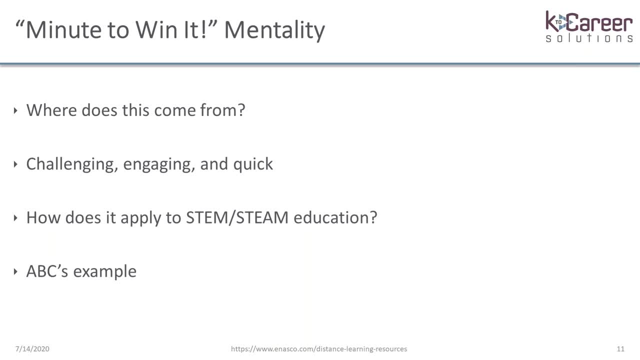 or contribute to your class learning environment. So let's jump on to the next one. So I'm going to try to get into catch up on time. I think I kind of went a little bit too fast or too slow on those last ones. But again, I wanted to kind of give you an idea of an array of low-level, all the way to fifth grade- different games that you can use. 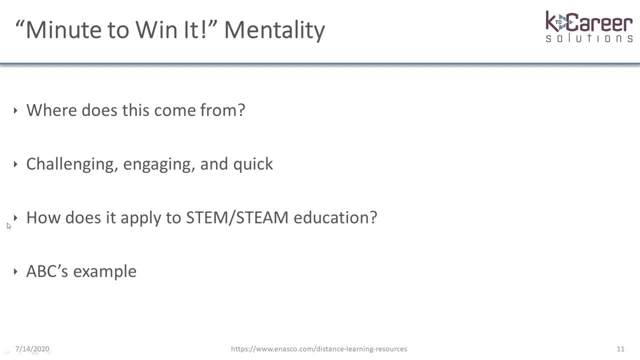 All right, so Minute to Win It strategy. This is based on the popular game show that took off in the early 2000s. It aired live in the US in 2010 on NBC. But what you may not know is that this is a spin-off of Every Second Counts back in the 80s. The idea is that you know someone, or a couple is. 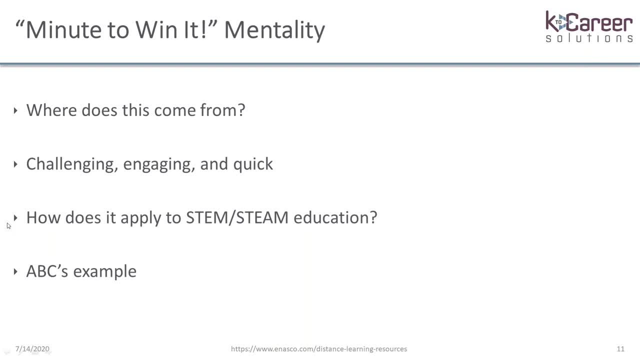 trying to get a game to complete a task in a minute. They would do so many rounds and then they would win money. You know it was very popular, So getting students to participate or get excited can be difficult. You know this game-like approach gets students interested, even for those that are just watching. It gets students thinking: you know, Hey, can I do that, Can I try that? And they can test the skills of students and it could be a physical challenge or a mental challenge or both, and it could be scaled up or down depending on the level of students. The best part is is that it's quick and you can fit it in your already over-the-top. 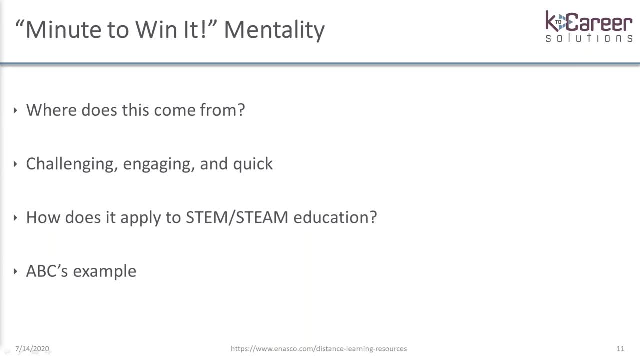 overcrowded schedule, so for one. it forces students to use skills they wouldn't normally use. oftentimes we're focusing on content knowledge, but students aren't always graded on communication, their collaboration skills or how they problem solve, Etc. this changes that, because you can have students. 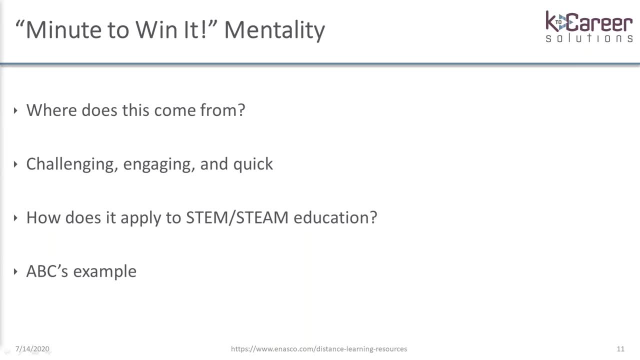 work together as pairs or groups, and students naturally use their engineer design cycle and the best part is that you can tie it to the challenges content. so one of the examples that they give is the ABCs, so the, for example, everybody can do the ABCs, you know, beginning to end, you know. 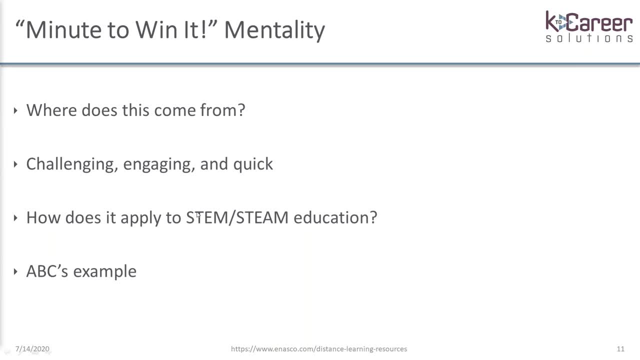 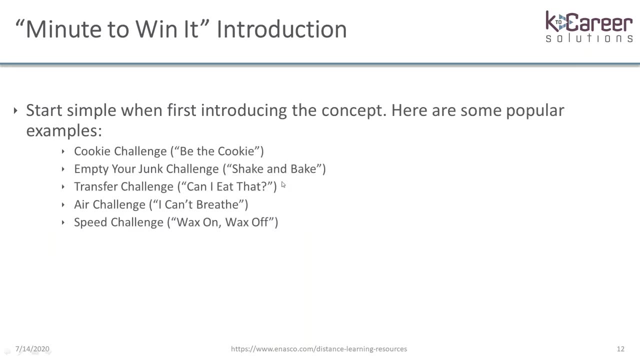 ABCD, EFG. but can they do it backwards in a minute, right? so that's the easy way to get students start to really think about it. normally I would test you guys, but for time's sake I'm not going to do that today because I got some other tests I want you to do. um, this is some introduction activities. 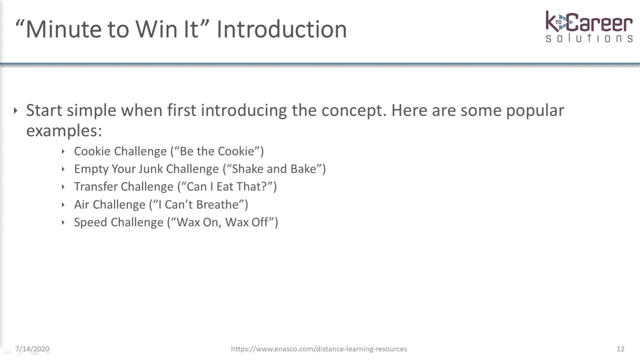 that you can use with this concept. you know you have the cookie challenge, um, this is where you put the cookie on your forehead and then, without touching it, you have to use the face muscles and move your face or body to move the cookie into your mouth from your forehead. so this is a 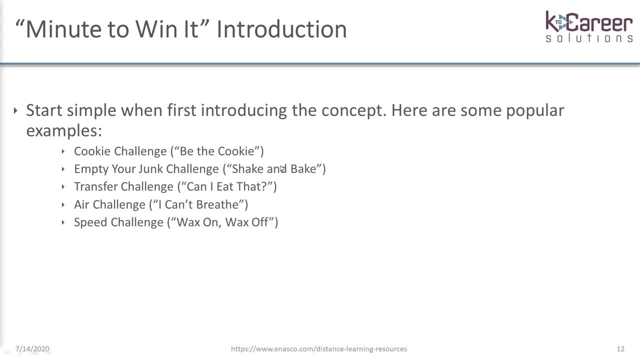 fun and interactive empty your junk challenge. so shake and bake, I like to call it so- basically tying, um, you know, a tissue box to the back around your waist and the box is actually behind you and you have items in your tissue box and you have to kind of shake and groove to get all the objects. 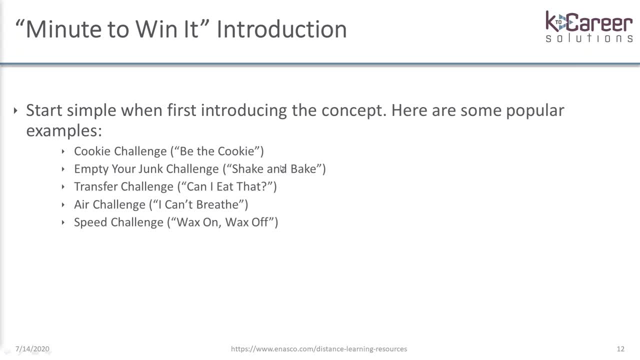 out of your tissue box. it's a fun, interactive thing and it gets students really engaged with that transfer challenge. so you can use a straw and you can move um things. I call it. can you eat this? so like using Smarties or some food that won't go up in a straw and then you've got to move them over to a plate and can you do that? 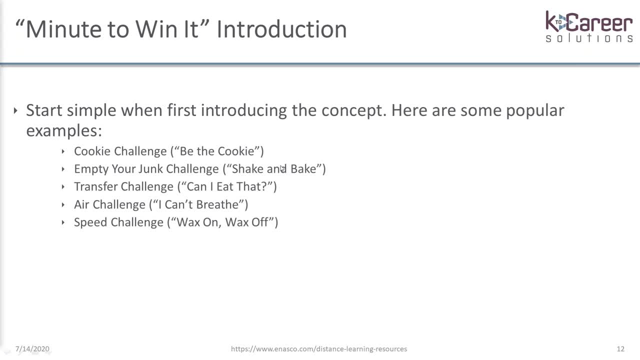 in a minute. air challenge. I can't breathe, so using a balloon. can you keep the balloon in the air with just breathing out loud? uh, just using your breath from one side to the other? so this is a fun challenge: um speed challenge, wax and walks up. I think it's kind of fun because this is seeing if. 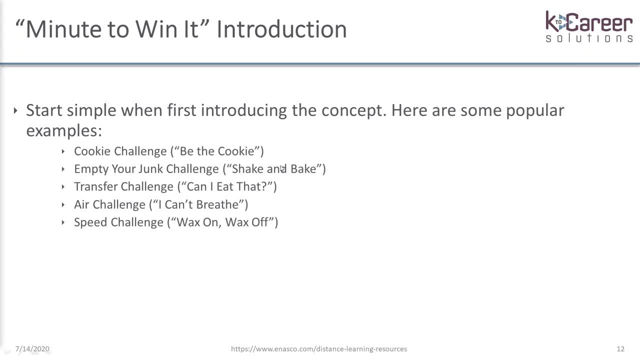 a student can use one arm behind their back, usually their non-dominant hand, and then using only their dominant hand to pull one tissue out at a time of a box and see if they can empty the whole tissue box in that one minute time and you can do spin-offs right. so this is- this is more of a warm. 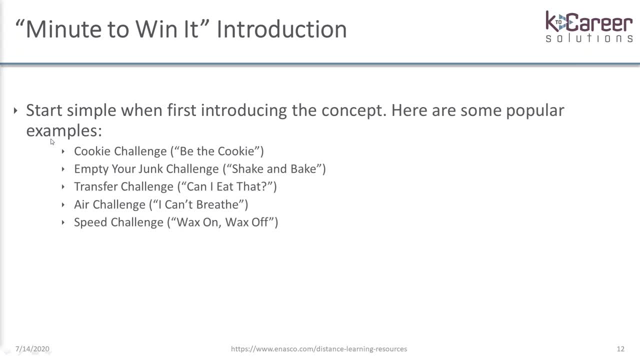 activities for the philosophy. you can alter these activities. for example, you could change the transfer game into using even and odd numbers. students could pick up, you know, numbers on laminated cards and drop them off on even numbers on a plate to your right, and then maybe odd. 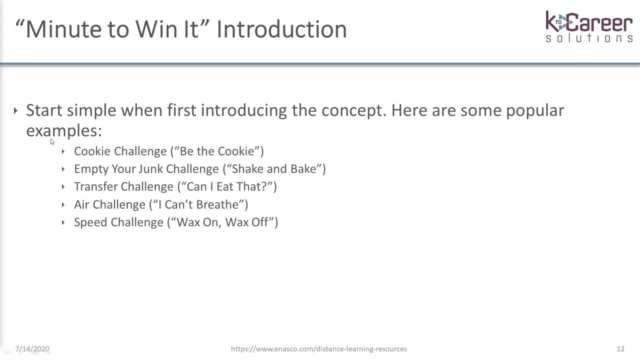 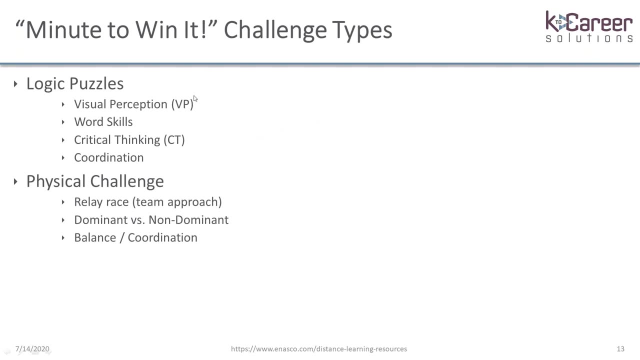 numbers on a plate to your left, same tactics, just changing this sounds looking related to math food, um. so this is that's. those are some great things, and there's different challenge types: visual perception, um, word skills, critical thinking, coordination under logical puzzles- and then there's also physical challenges where you're actually, you know, doing a relay race or change checking. 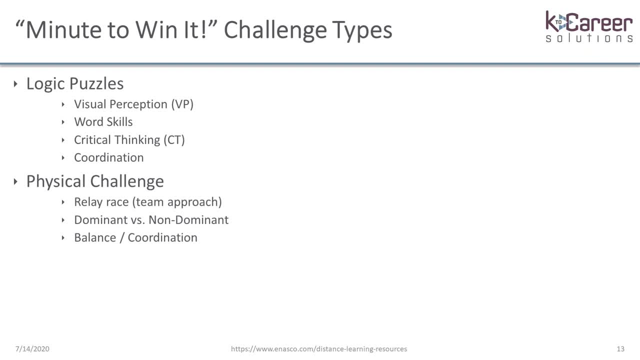 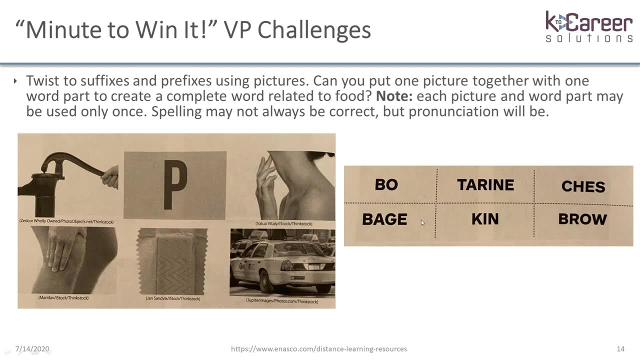 your dominant versus your non-dominant, um, senses like your hand, your eyes, and also balance and coordination. so we're going to go into some of these. so this is a twist on suffixes and prefixes using pictures. um, you know, can you put one picture on to the left with the one, um, uh, complete word on the right and each picture? 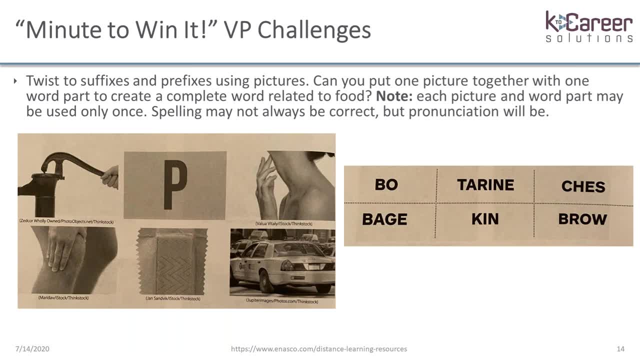 and word part may be only used once, so spelling may not always be correct, but pronunciation will be. so I'm going to wait for about 30 seconds here and see if you guys can come up with some of the different answers. all right, and usually you would say, hey, you got 10 more seconds, Etc. so, um, but with sake of time, I'm 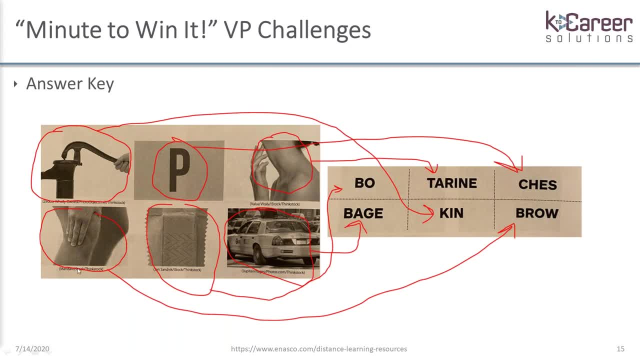 going to kind of give you the answer key here. so just to some things. you can see. you know you can see pumpkin, um. you can see the P with peaches- um, you know you can see, um, uh, you can see the nectarines. brownie is probably one of the hardest gumbo cabbage and 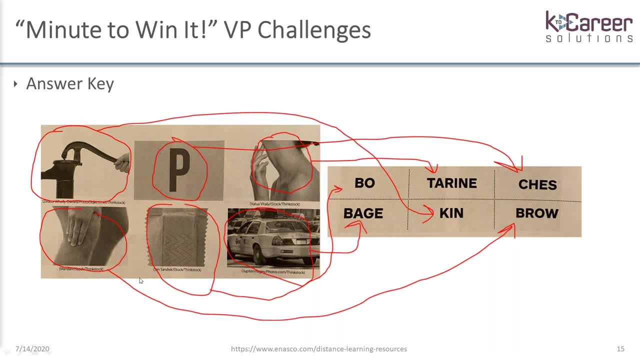 there's other variations that you can use as well. um, you know, you can use pictures of landmarks, familiar areas or vocabulary. change the time limit? um, you know, so it's, it's okay, you know. and so, again, this is a way for students to maybe, you know, critically think about something that. 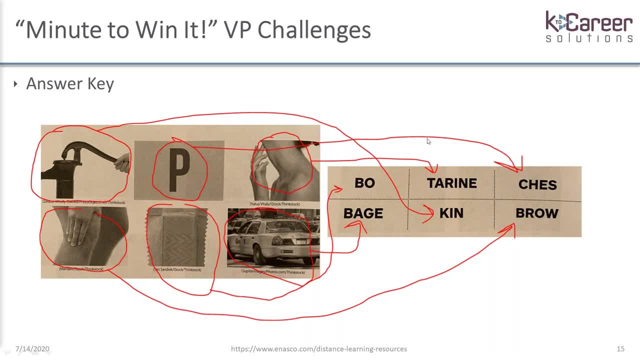 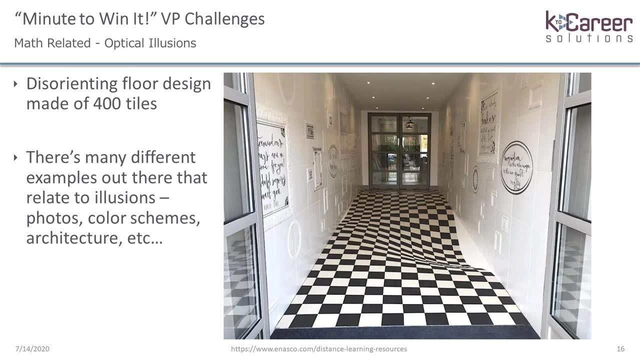 they haven't done before, to kind of get some visual perception skills um, done, um and then you also have math related visual perceptions, right? so this is a disoriented floor design made with 400 tiles. optical illusions are a great way um to be getting students thinking. 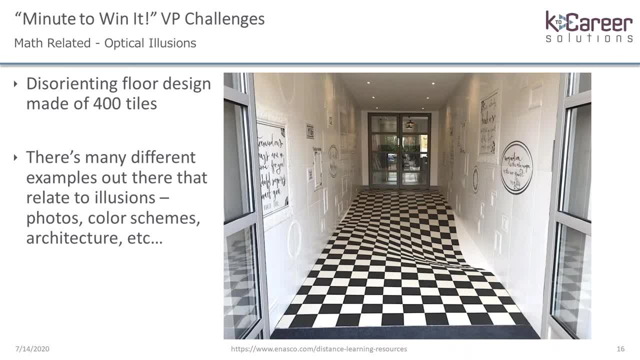 about these challenges using photos, color schemes, architecture, Etc. so this is again that one of those illusions. that floor isn't dipping down, it is flat, but is the optical illusion effect that we have. that's kind of really cool. um, also, look at the circles to the right. are there? are? 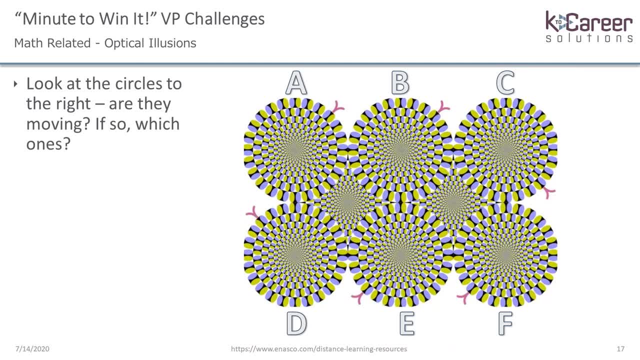 they moving? if so, which ones? I'll kind of give you about 10 seconds to kind of look and kind of see what do you think? all right, we'll see if anybody has some answers, um, to see if they think: is it a, is it B, C, D, E? 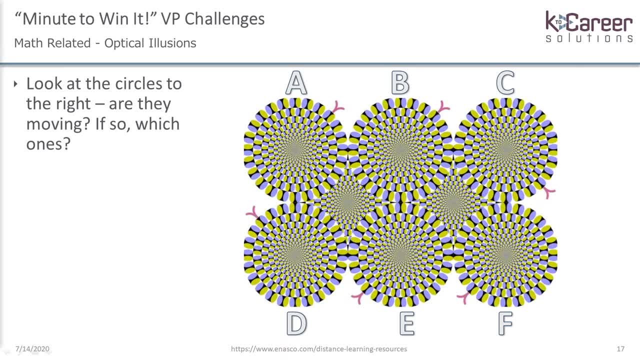 F, any combinations, all of them. I kind of want to see what you think. all right, so we got, uh, Crystal thinks they aren't moving, Carly thinks they're not moving. um, all of them are moving. Patricia, um, and, and no, this is, this is very common um, there's a lot. 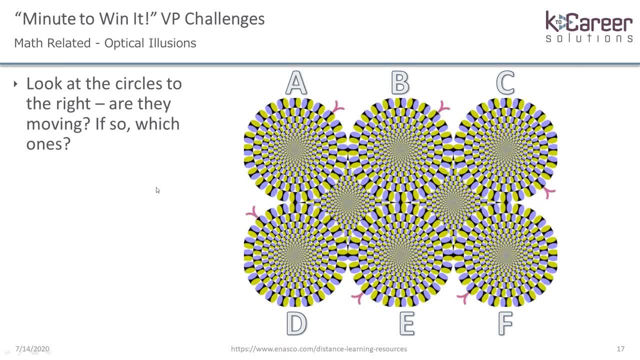 of mixed answers, usually um, and the reason being is: because there there's a perception here, so the answer is actually none of them. and no, this isn't a gif, um, you know. so this is. the image was inspired by the famous illusion rotating snakes, created by a Japanese psychologist and professor. so it is example of a peripheral drift illusion where the 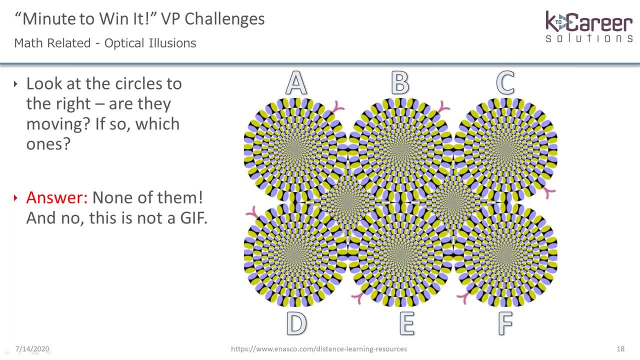 still image appears as if it is moving, despite the swirling um and twirling that you think. you see, this is actually a stagnant image. the human brain kind of processes information in a very basic way. as we move our eyes from light left to right, we pick up visual cues both directly and in a 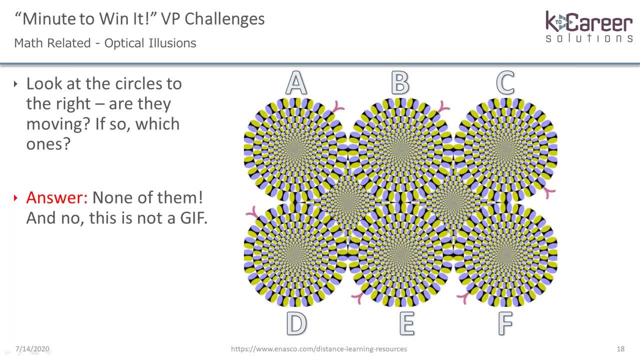 peripheral vision that our brain then processes it kind of piece by piece, not continuously. so, and because our brains process high contrast elements- like you know, black on white- faster than low contrast ones like black on gray, that lapse in mental read time is ultimately what causes the apparent motion. so when you stare at one part of the photo without moving or blinking, 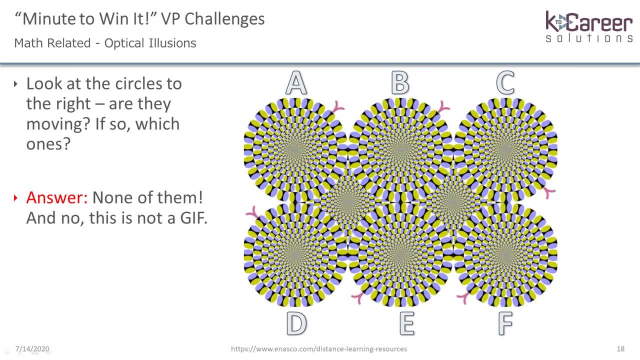 your eyes there shouldn't be any motion. and it's kind of hard to do because when we tend to look at our peripherals, um, but that we look through our peripherals. but you know, that's a little fun activity that you can use as students, and I also like doing this activity. 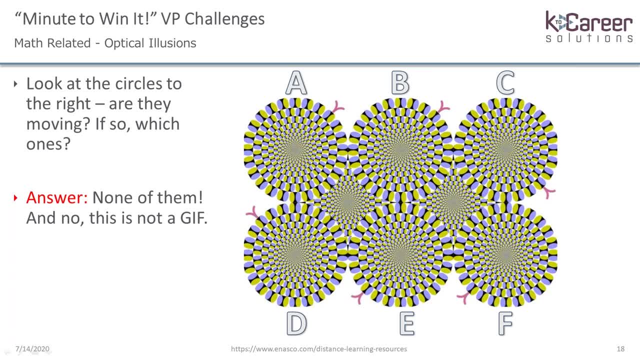 because it shows how math is related to science. a lot of people still believe math and science is separate, but they are actually one in the same reason is because math is the language of science. it's it's how we explain any science phenomenon or the world around us. for example, gravity is visible. 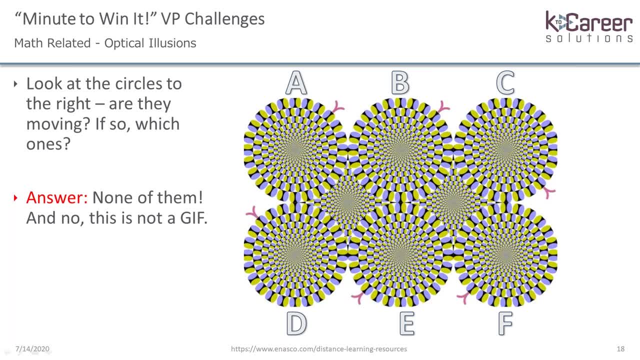 and easy for students to kind of witness newest law, but it's much more different to explain it mathematically. when you're teaching math, you're also inadvertently teaching science, and it's just that people don't always realize it or think of it that way. so this is something to think about, um when you're using, but that's a great activity. 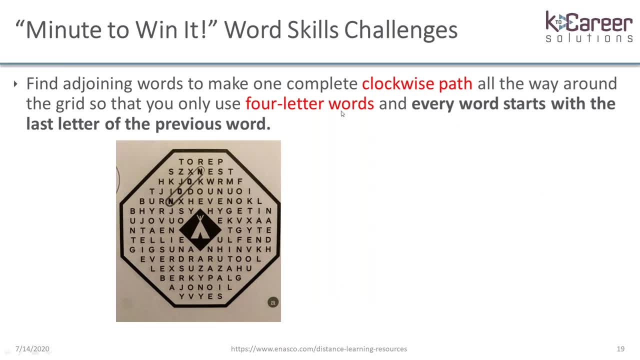 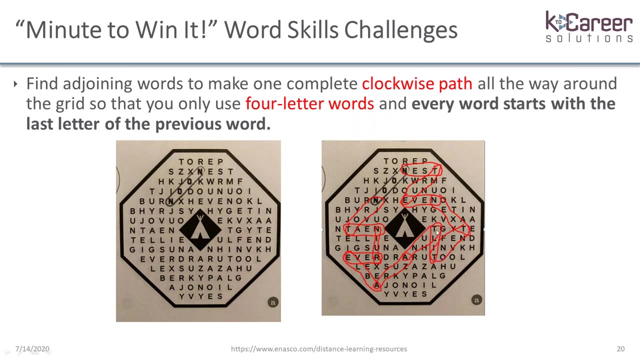 that you can use also world skill, word skill, challenges. this is a unique way or shift that you can use vocabulary for math. so basically we're taking here and we're actually coming up with a path of words that you can use. so nest, turn, even next tent, tilt, uh, tuna, Aurora, and then you 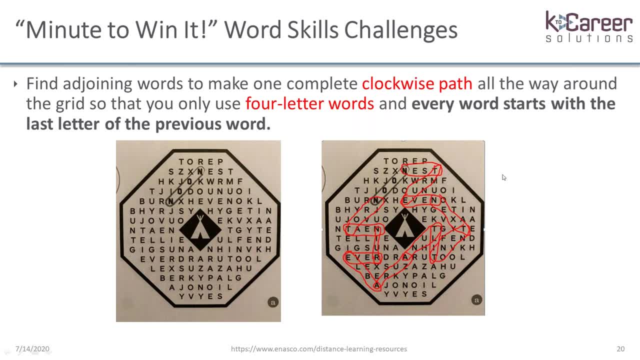 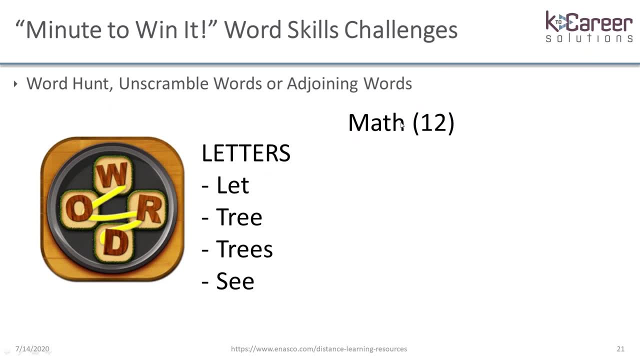 can build all the way around. so this is a nice little puzzle that you can also use. but I have some different variations of that as well. um word hunt, unscrabble words, so letters, so like math. you can actually unscramble math and create actually 12 words. um, I'm, I'm, I, and just to prove it, I'm. 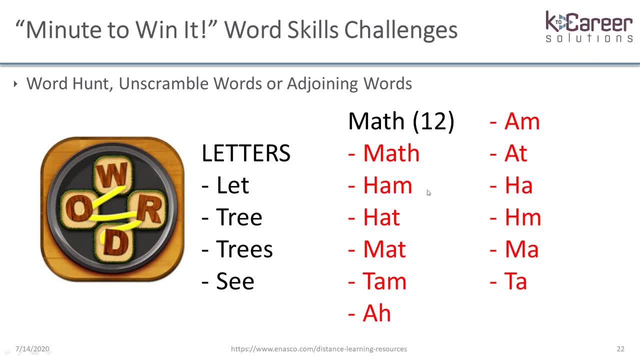 going to show it to you. so these are all the different 12 words that you'd be able to use. and yes, Tam and ta are words. um, you know, Tam is like a tight-fitting Scottish cap and ta is thanks. we get questions about: hey, are those actual words? yes, and there, are recognized by the Scrabble too. 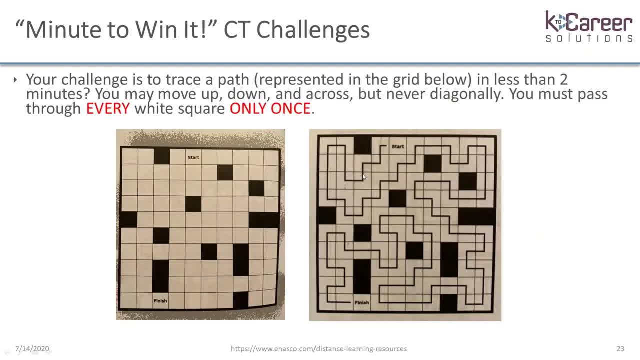 so just something to be aware of. uh, fun little activities that you can do. um, this is another challenge, that this coordination challenge. are different challenge type? um classic, you know: start in one spot, you go only through one square once and you have to complete the challenge you. 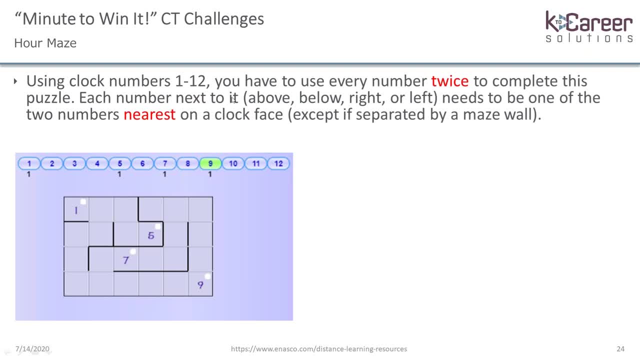 can do this with a kind of type of math um. so this is like using clock numbers one to 12. you have to use it for every number twice. to complete this puzzle, each number next square point above below, right or left, and needs to be one of the two numbers nearest on. 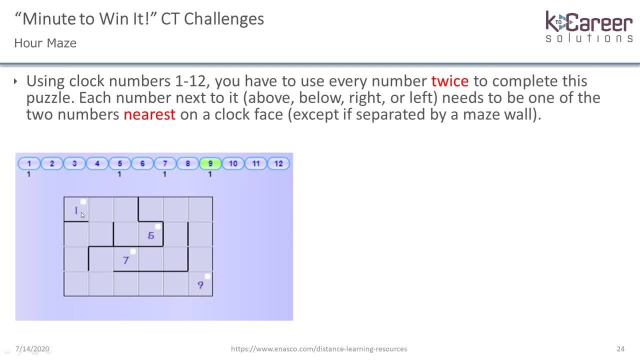 the clock face, except to separate by a May's wall. so, for example, one needs to be next to two, five needs to be next to four or or two, or you can't be anything else. five could be next to four or six, seven could be next to six or eight, and nine could be next to eight or ten. so you would go through. 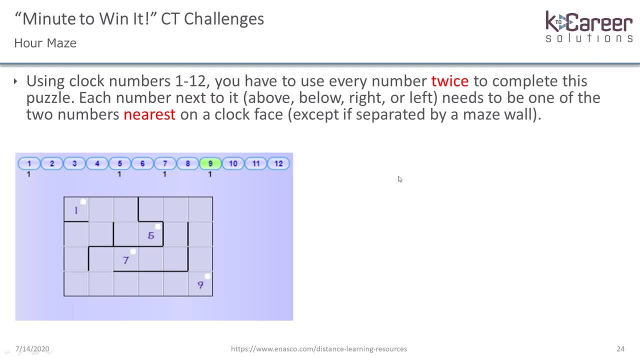 this and try to figure out if you can solve this. normally I would allow you to do this, but for time sake, unfortunately I can't don't have enough time. so this kind of gives you the puzzle to kind of think about if you want to use that activity as well, and this is something 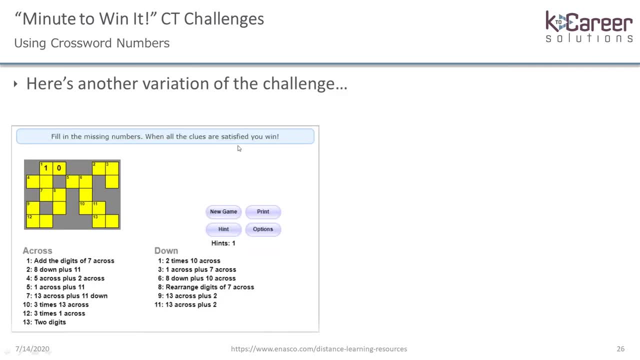 that's also tied to math is fun. here's another minute to win it, challenge that you can do here. i gave you a hint. so using crossword numbers, right. so one across is add the digits of seven across. so you know that if you add the digits of seven across, it should equal ten and we'd be able 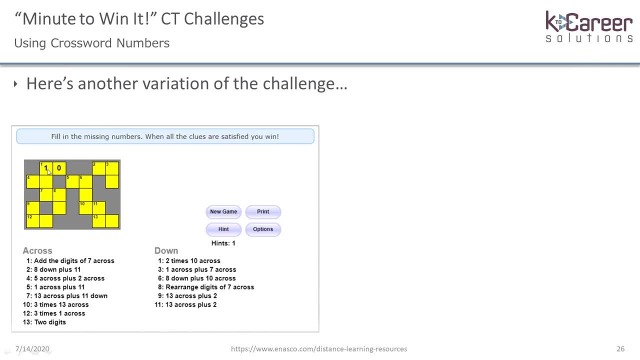 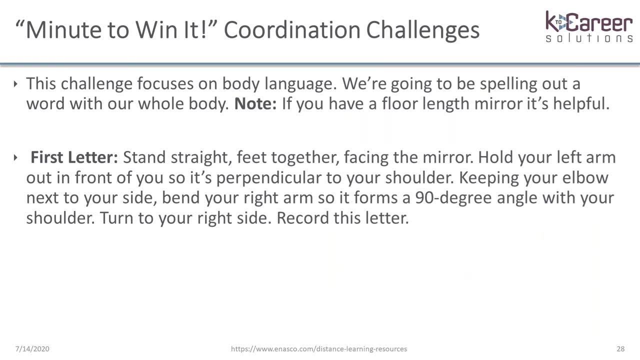 to go through this process step by step. once i gave you this hint, you can use this challenge if you want, but i did provide the answer as well. i won't show you exactly right now, so if you later you want to go back and try it, you can coordination challenges also. so this is using body language, so 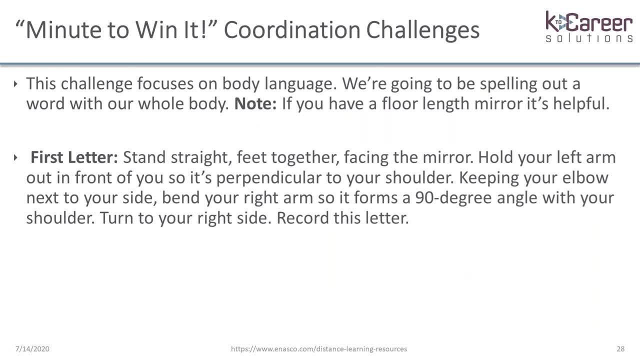 body language could be an also great coordination challenge, because you can start talking about symmetry, angles, degrees, etc. so this challenge focus on body language. we're spelling out a word with the whole body. um, if you have a floor length mirror, it is helpful for this specific one. so 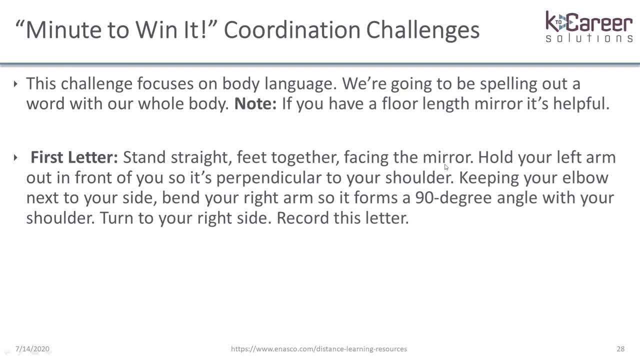 the first letter that you're going to make is basically standing straight feet together facing the mirror. hold your left arm out in front of you so it's perpendicular to your shoulder, keeping your elbow next to your side. bend your arm so it forms a 90 degree angle. 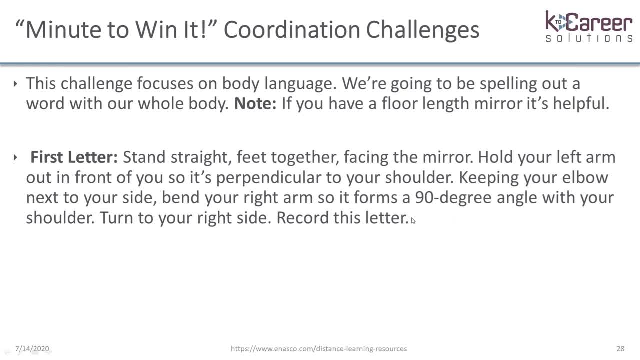 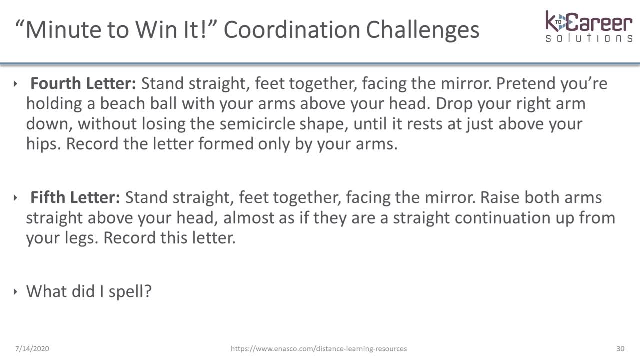 with your shoulders and turn to your right side and record this letter and eventually you would use the second letter, third letter, fourth letter, fifth letter. i'm going through this quickly again because again i want to be able to cover everything and then you'd say, okay, what letter? 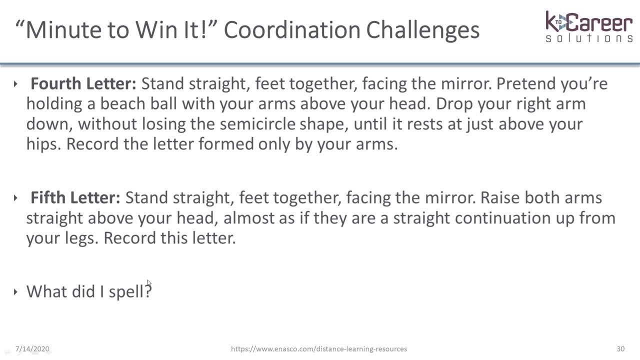 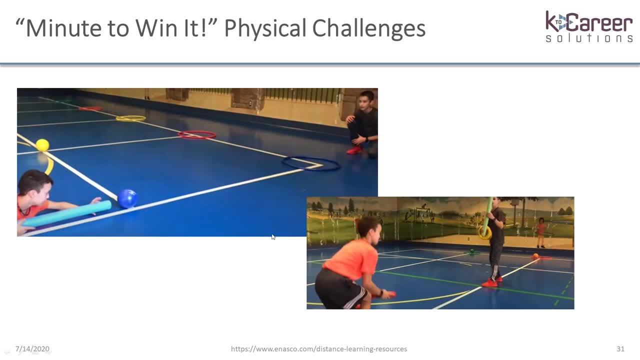 did you spell um and then i'll let you do that activity, um, but the letter that you or the word that you should spell is fresh, so i'll see if you can figure that out on yourself. so another physical. so we just did mental challenges um, this is physical challenges. so these are ways. 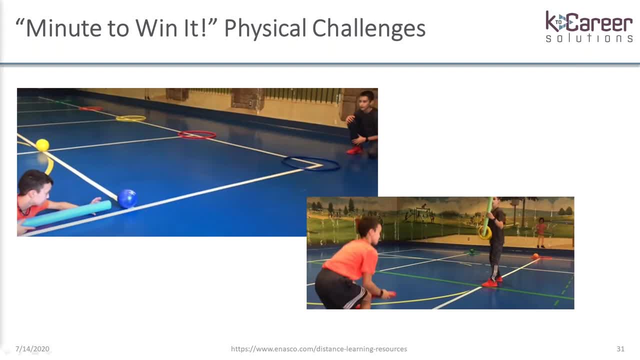 that you can, strategies that you can use with students. um, this is just one example: using, like swim noodle, hula hoops, you know, softball- and balls, rings, etc. and they're basically creating pool, right, and so for every ball that he hits in there into the ring, he gets 10 points for every. 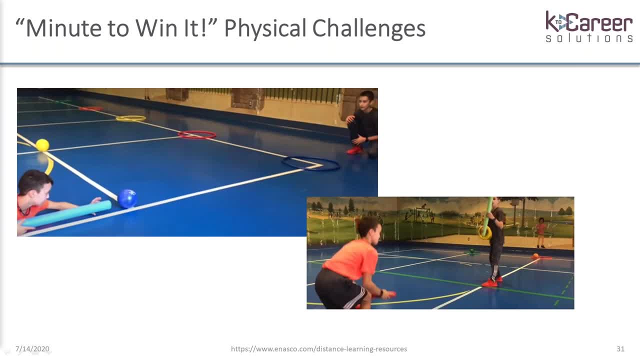 one he misses, he loses points. this is a minute to win it. challenge and you can keep track of the point system. is that it can be included in math or you can do variations of physical challenges, like if you want to throw rings. um, that's more of like a skills challenge that you can. same concept. 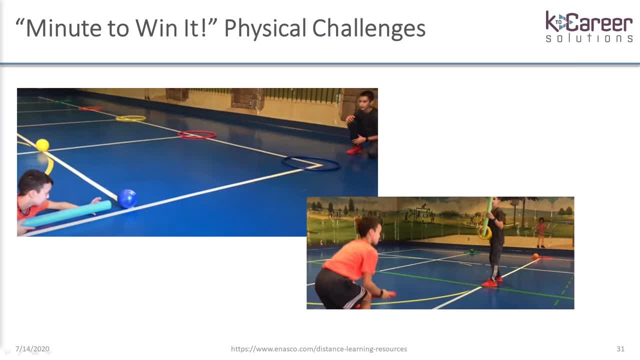 from a certain distance. have the students measure out feet? well, um, maybe they don't have a measuring yardstick. well, how are you going to measure out five feet? well, you have feet right on your foot. um, maybe you can use your shoe size to figure that out. so there's different ways for students. 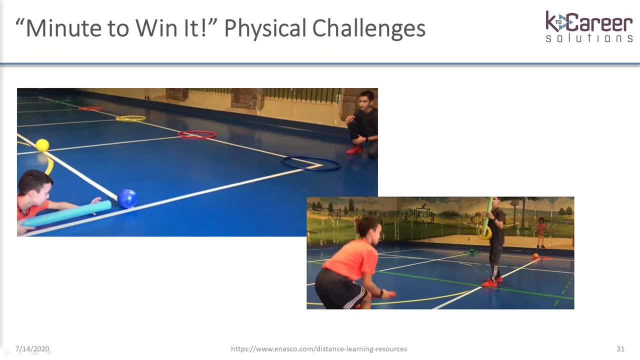 to kind of think about those kind of distance and creating those distances. and you can also use, like hopscotch, variation, um, you know decimals, place values and then just giving them task cards to say, hey, you have this only touch, you know equivalent fractions. or you know, um, you know reduction, uh, reduced fractions. 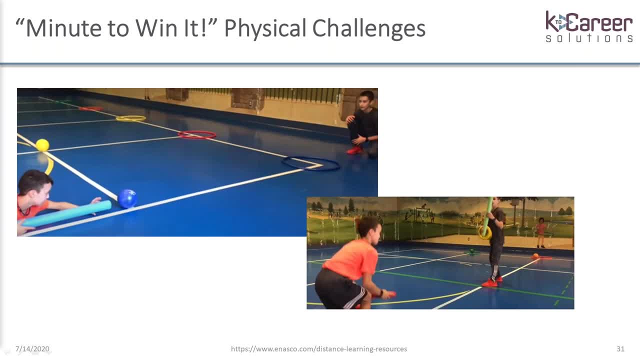 etc. um. and then there's also statistics that you can use: um, throughout these different physical challenges, you know dominant versus non-dominant senses, so your left versus your right hand, um, or your foot, um, your eyes, things like that, and stuff like that, you know. so that's, that's a. 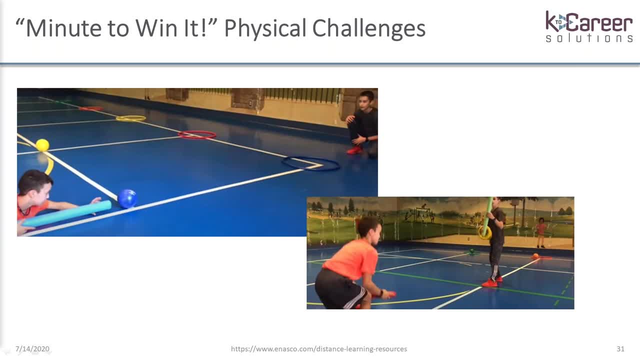 things like that. and, statistically, what does your classroom have in as far as like dominance? um, and this could be a physical challenge- that this the students can do at home even, and then they can record that and send that information, and then you have a group of students or a whole class. 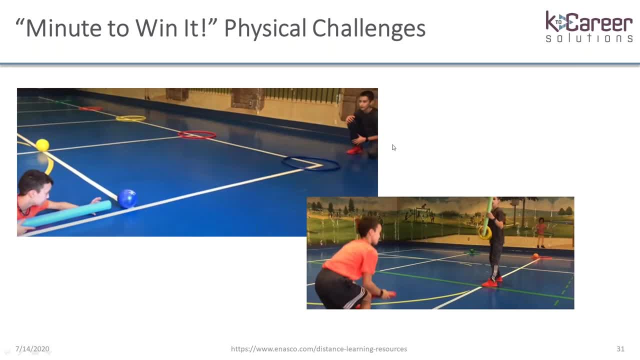 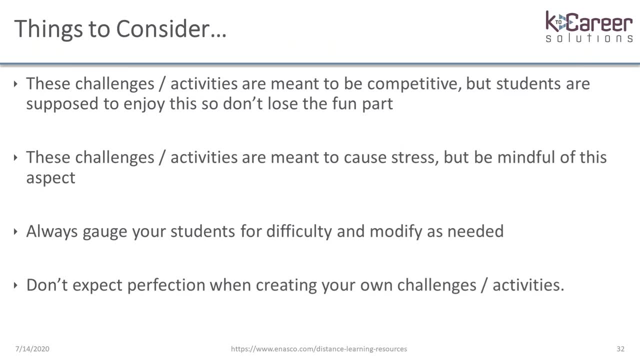 with all statistics that you can do. so, all kinds of different minute to win it, challenges that you can do with your students, things that different consider, um, i definitely have those out there. um, i think that they're pretty self-explanatory. uh, one things i definitely want to make sure to. 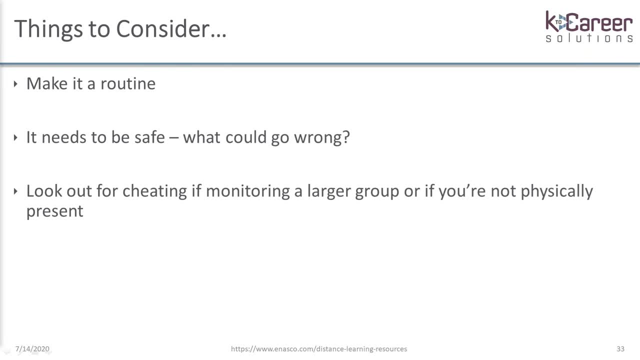 focus on is that um. i always encourage safety um, and then look out for cheating if monitoring large group, if you're not physically present. so if you do anything online like scramble words and things like that, students might look to cheat um, and then you don't want. 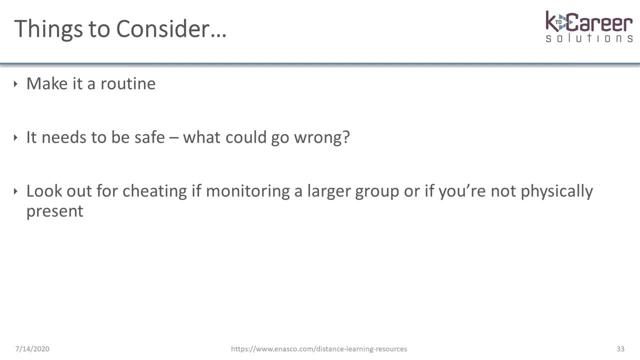 to let the competitive edge take over, right? this is fun and it's supposed to be engaging, but you don't want it to ruin the things for other students as well, so that's so. that's what I've kind of done for you today is kind of create a variety of different challenges and 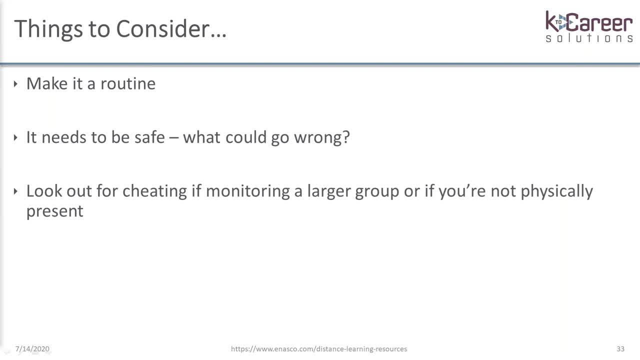 activities that are meant to be, you know, kind of done within one to three minutes, and you can change the variety of this now, that being said, you can certainly make these activities longer, shorter, that's fine, but the idea is that you want to create quick, intense and engaging activities. 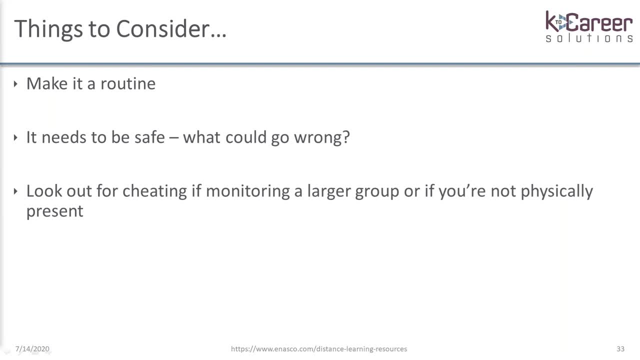 to make your students really focus for a short time span, and whenever I build these exercises, I focus on two elements: the time limit and the difficulty. they both are weighted equally whenever I'm trying to determine the outcome that I want to achieve. the other thing is great about the 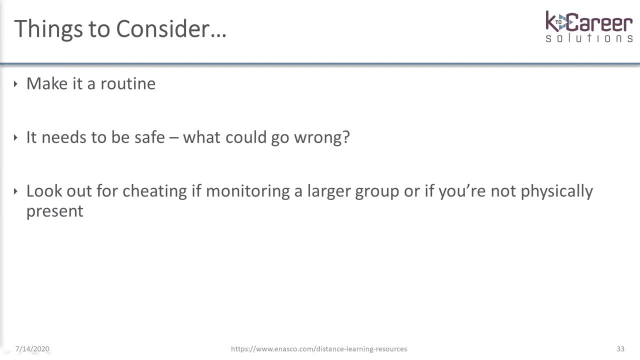 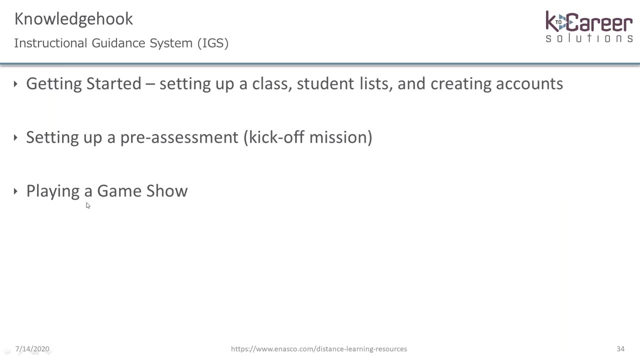 minute to win mentality is that it can be used and they can be adapted to other subjects, not just math, as you can see. so, being elementary teachers, you can use this mentality and kind of transition to other subjects as well. and then the last thing that we're going to be covering is knowledge hook. 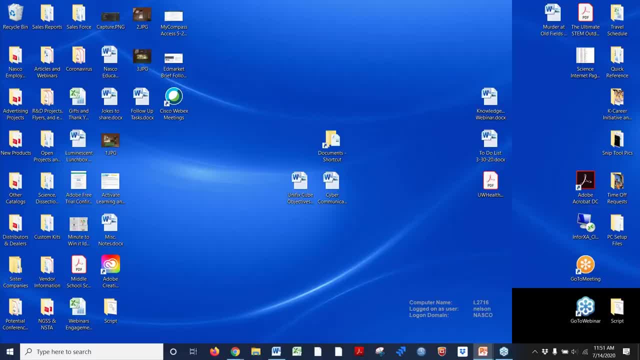 and this is a great and this is a NASCO specific tool that we're going to be kind of focusing on, and I just want to give you a little bit of an overview of what we're going to be focusing on, and I just want to give you a little bit of an overview of what we're going to be focusing on. 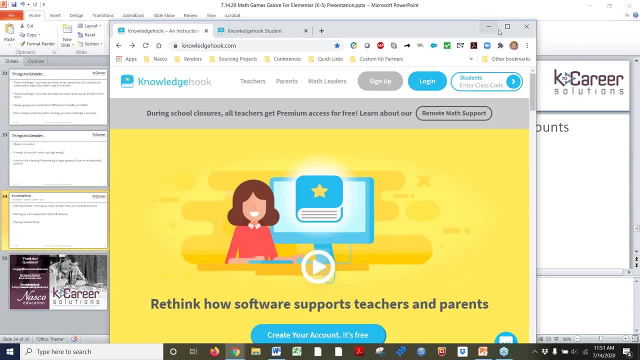 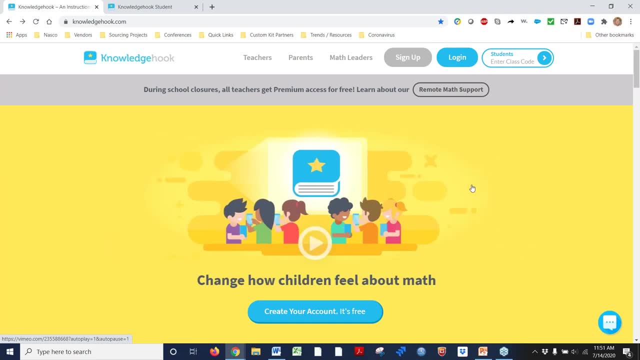 wanted to do it because, again, it is free to access. right now it is tailored for grades 3 to 12, but this is an easy way for you to get engaged with students and it has game applications built right into it and you can use it for a lower grade level. so now, typically you would sign up, but what? 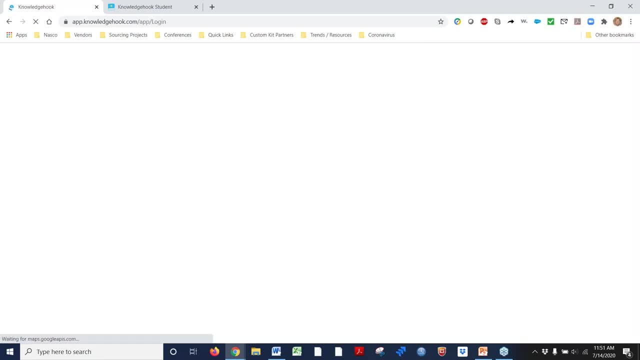 I'm going to do is I'm going to log in as my teacher, so you can kind of give an idea of what it is. and the nice thing is, when you log in, you can sign in with google, so you don't have to sign in right away. to make it very easy for you to log in, you can sign in with google, so you don't have 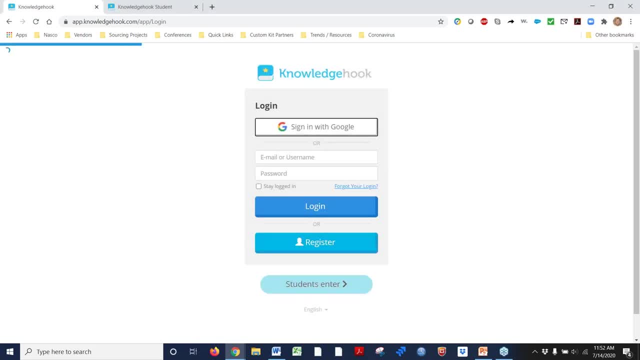 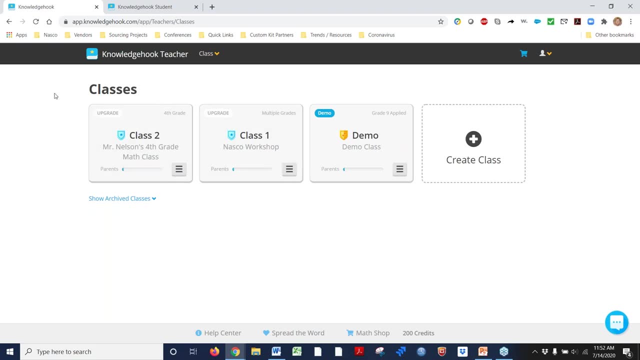 to sign in right away to make it very convenient um to be able to sign in um into your classroom. so what I'm going to do is I'm going to actually have you guys participate with me um right now. so there's going to be um all we have here. so I'm going to have Nelson's class here and what I want. 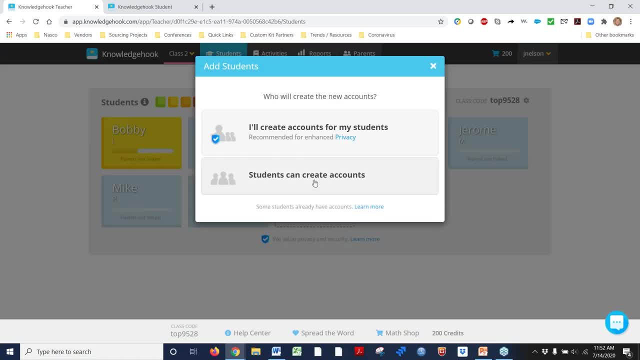 you to do is you're going to sign in with me, and students could create their own account, so I'm going to quickly have you sign in. what you're going to do is you're going to go to this website. you're going to use this code. 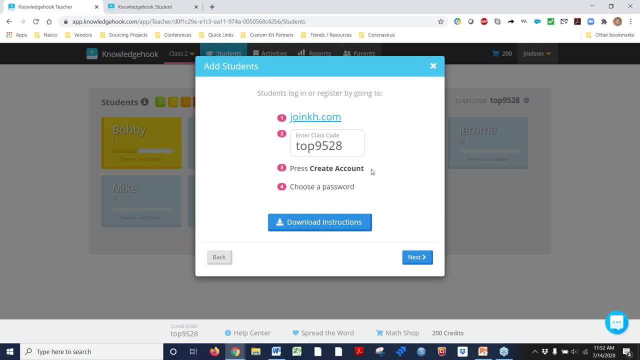 and then you're going to press create accounts and then so, when you create accounts, um, you choose a password very easy, like 123, abc, something very convenient. this isn't going to be something that you're going to be tested on or anything like that, but this is just to quickly. 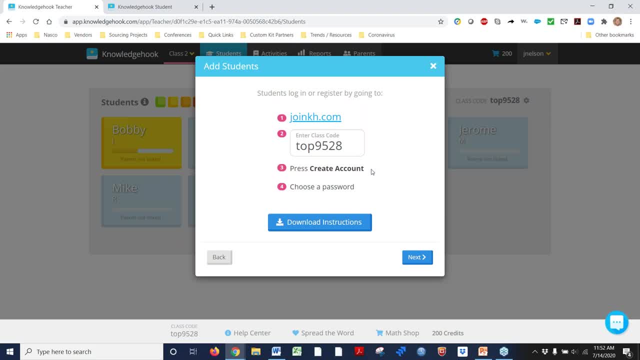 get you engaged with something that I can show you how that students would be able to use this content, um. so again, joinkhcom, use this code, top 9528, create your account, choose your password- um- and then um. we'll get this this going here. so what I'll do is I will. 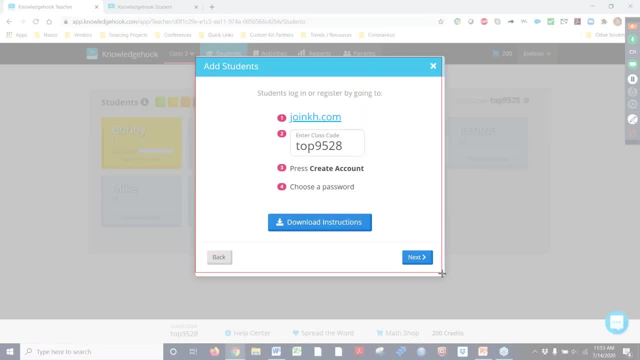 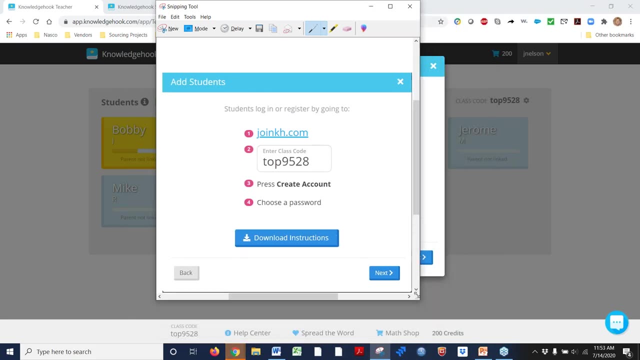 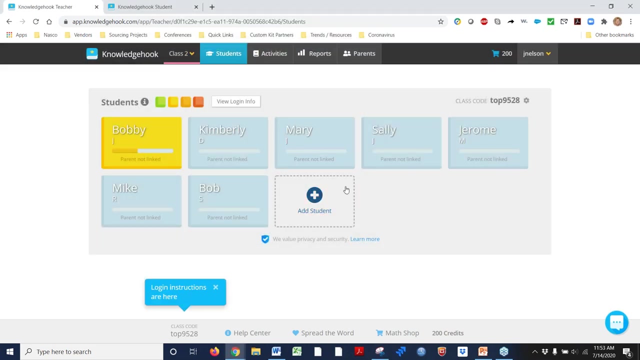 basically use this little clip here to make sure that this is still on the screen and accessible um and. but I want to make sure to keep the progress, keep going um throughout this whole thing here. so what I'm going to do is I'm going to hit next and I'm going to see the students. 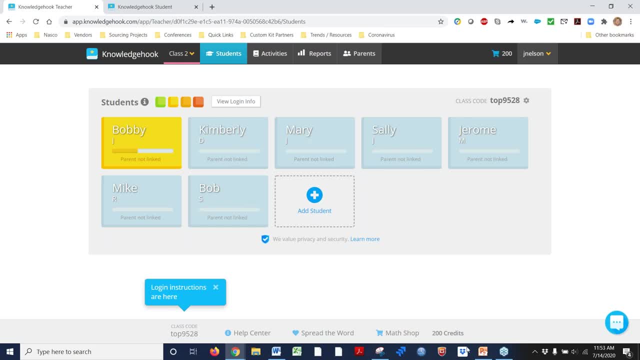 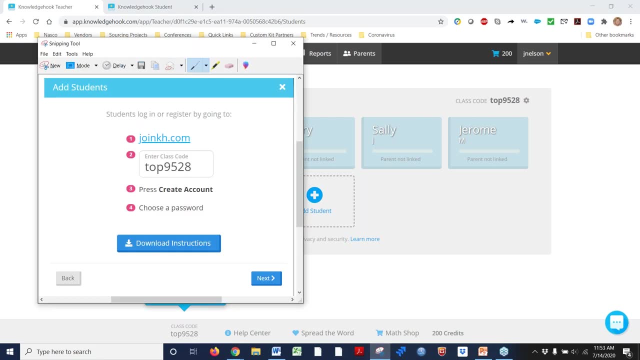 you're going to see people kind of log in as you're kind of creating an account, the next thing I'll do is I'm going to make sure that this is actually close enough. um, so, if you guys are using it here, you're going to hit access to uh, as I mentioned, 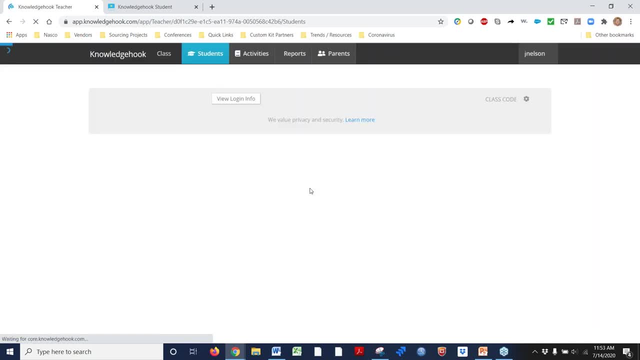 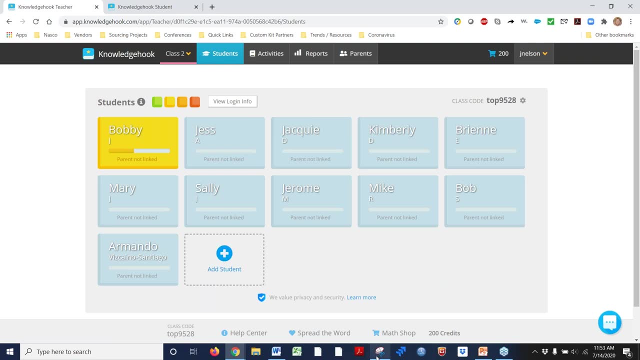 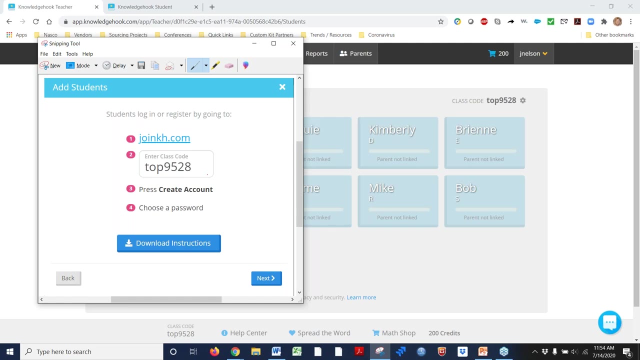 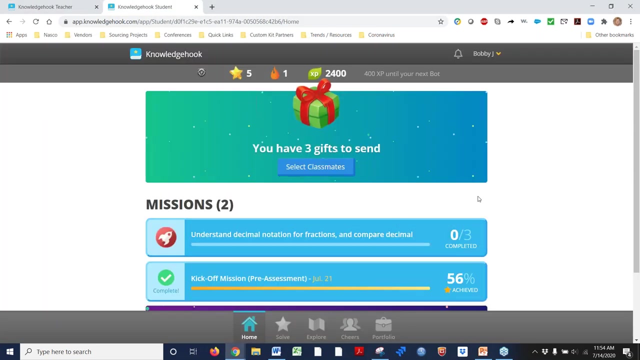 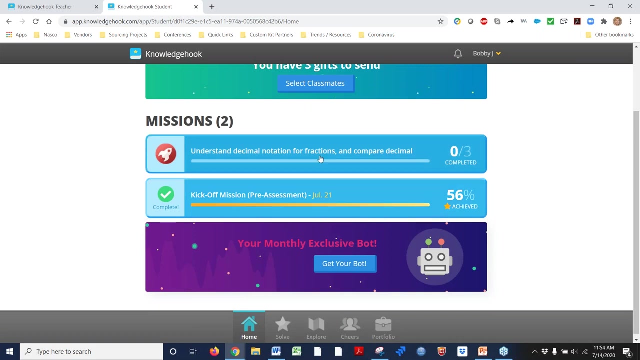 to create in the chat um. here you can see that I'm creating an account And then what I'm going to do is what you should see is something similar to this. Now I have experience here. I want you to click on the kickoff pre assessment lesson. There should be two lessons in there. 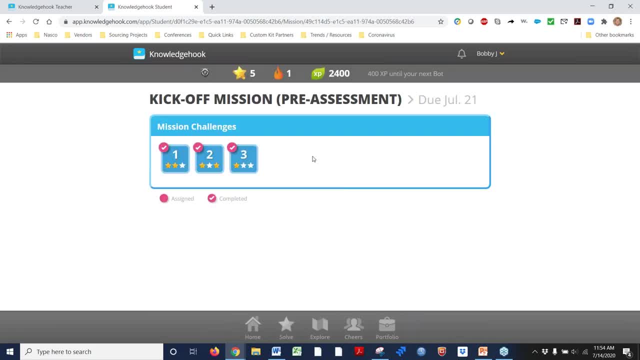 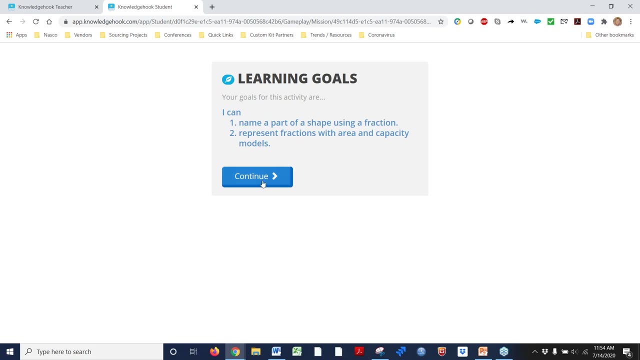 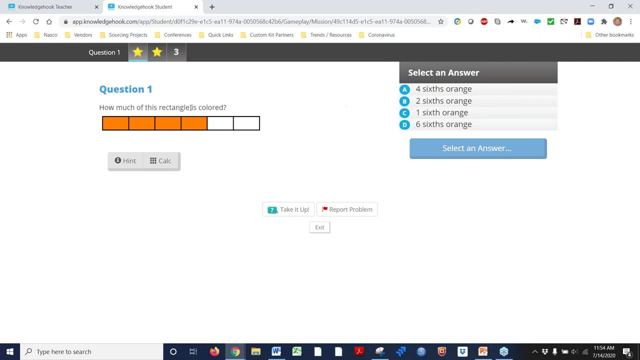 This one is going to kind of give you an idea that this is a way to work with students, to strategize on where they're at At first. this is your pre assessment, to say, okay, if students are needed to learn, this is the learning goals that we're going to be able to do, and you can go through this process right now with me to, or you're on your own pace. So how much of this rectangle is colored? so we have 1234 out of 64 out of there is. 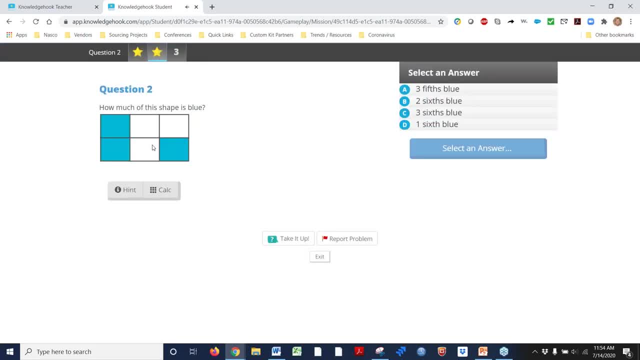 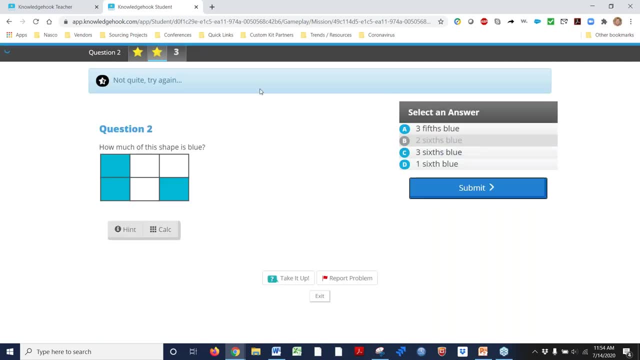 And then we'll say, oh yes, this is correct. okay, we try again. Now if, for instance, we were to struggle with anything, how much is the shape? is blue? Maybe we said it was two out of there. Well, no, not quite, try again. 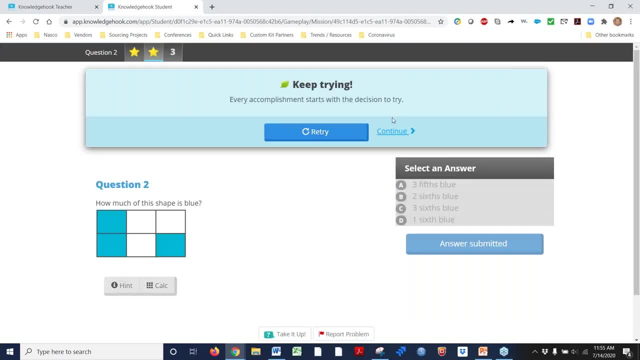 What if one of a blue? You know what: Keep trying. every accomplishment starts with a decision to try. so we want to get students to think that just because you got the wrong answer Does mean you give up. You can keep retrying over and over again, and that's. that's part of the process of learning is through failure as well, so you can either continue on or you can retry the same different one when you hit retry. 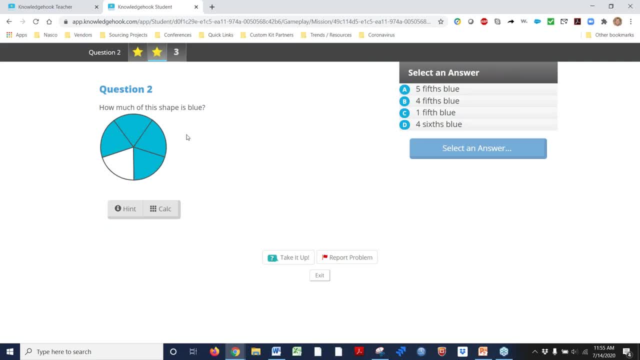 Now it's going to switch your question up, so it's a great way for you to kind of see how this actually keeps students honest and that they're not going to be using the same thing over and over again. Another thing is that you can report a problem. if you're having difficulty seeing this, There's hints that you can use to be able to work through this problem. 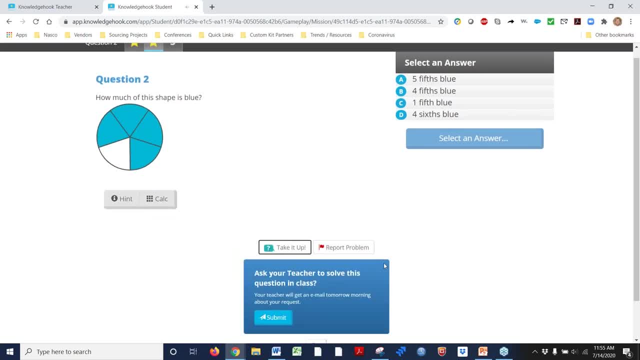 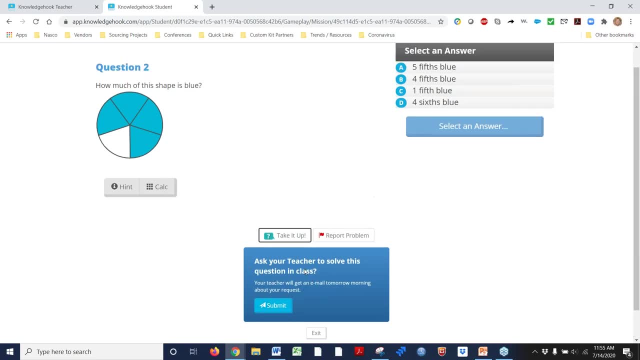 There's calculators and then there's also take it up. This allows you to ask the question to the teacher, saying, Hey, I'm really having trouble this. can we, you know, answer this as a class? this, specifically, it kind of gets students to really take ownership of their learning, to be able to work through this answer. 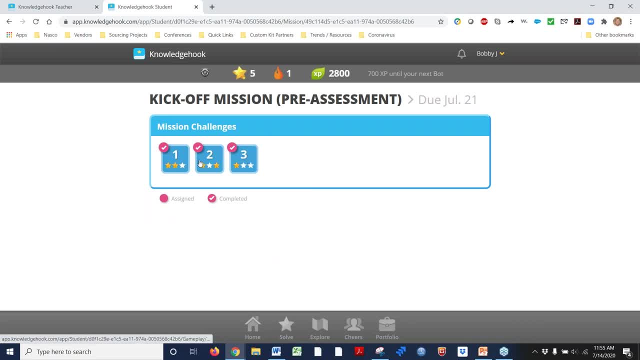 So if you want to exit, you can go back out As you gain and answer different questions. So if you want to exit, you can go back out As you gain and answer different questions. You're going to notice that you're starting to get stars and some of these other different power ups, so it has a game like mentality that you're gaining experience to level up. 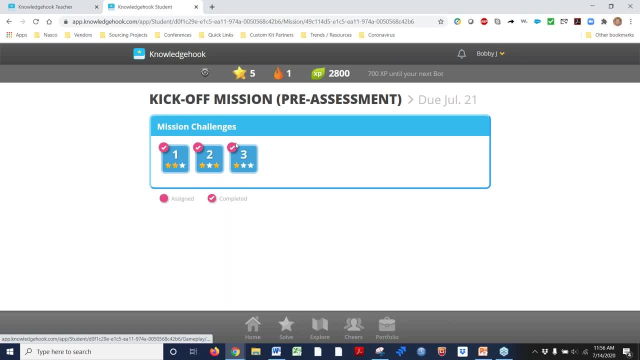 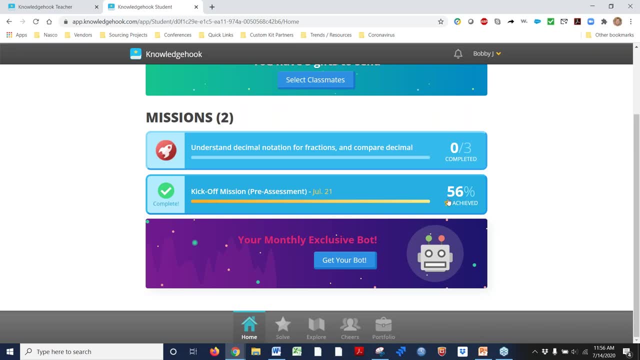 So it has that easy and how, and so when you're all done, You can actually go back to your very beginning page And you can see how much you actually achieved of this. There's also different things that you can get exclusive, but there's also different activities that I can add as well. 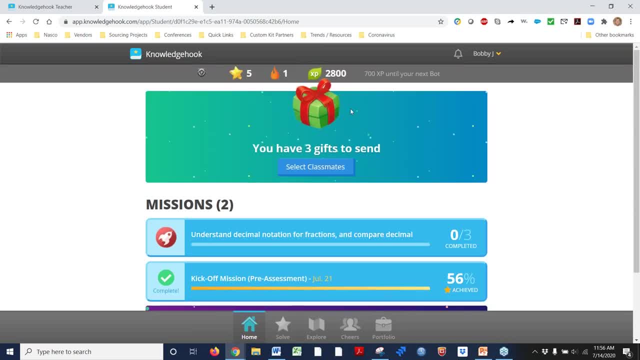 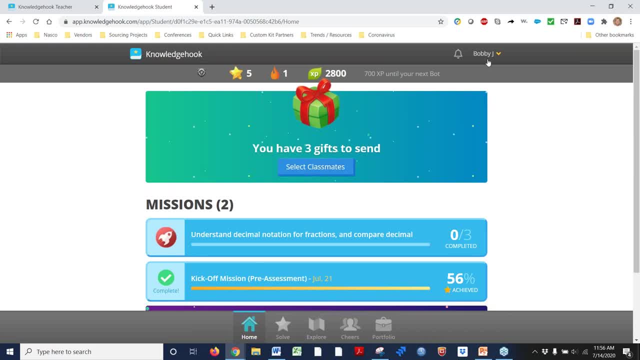 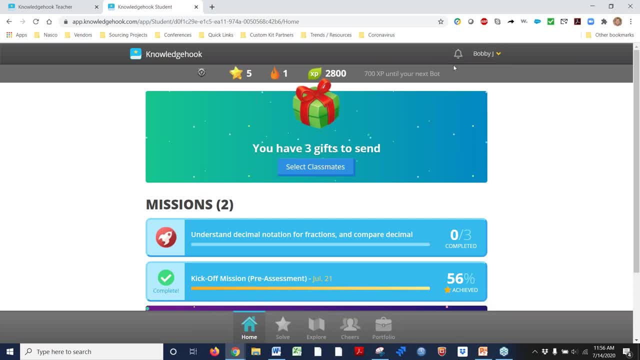 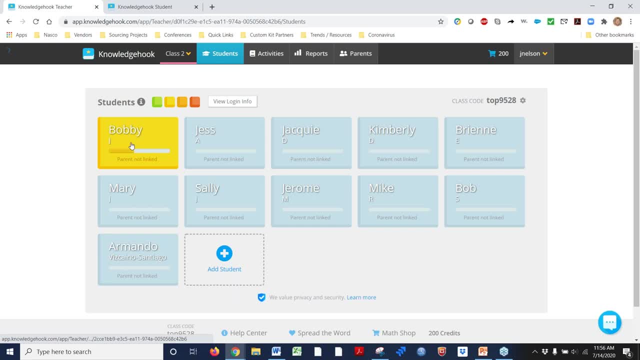 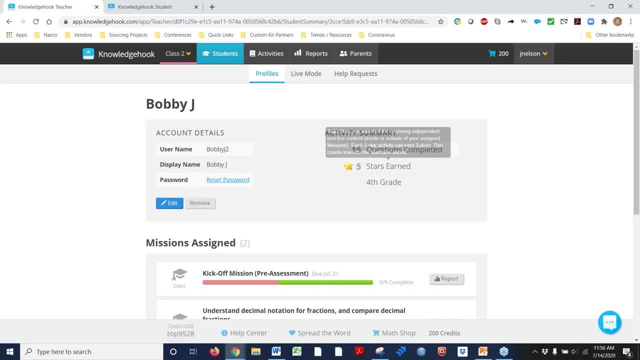 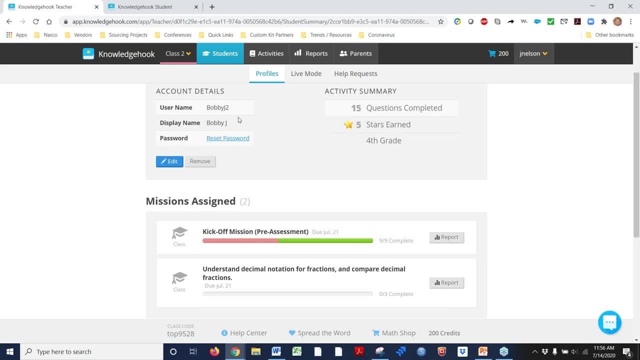 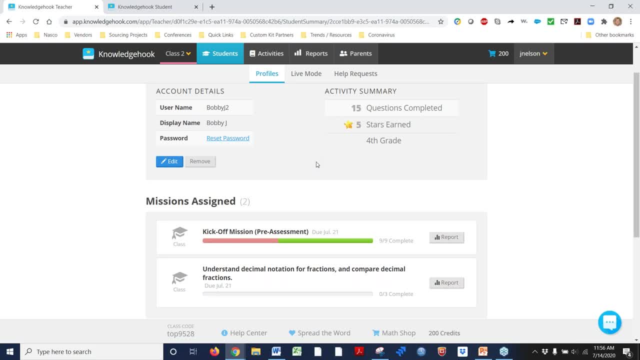 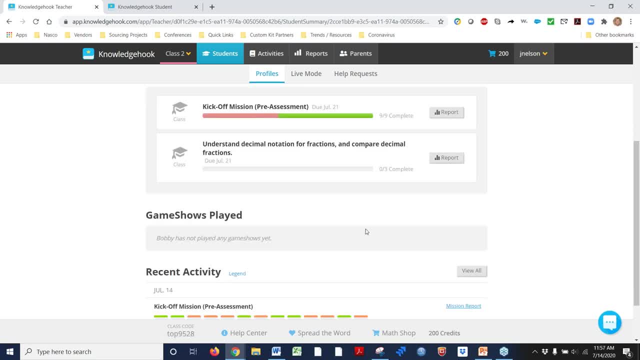 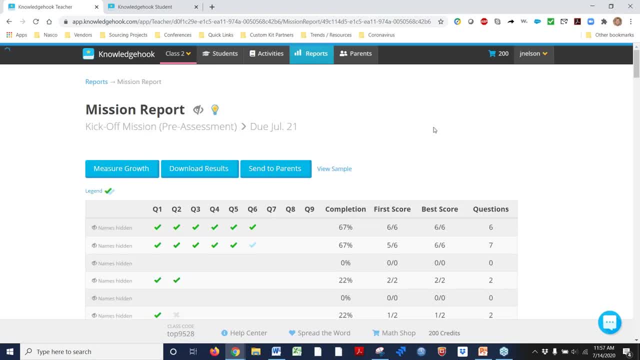 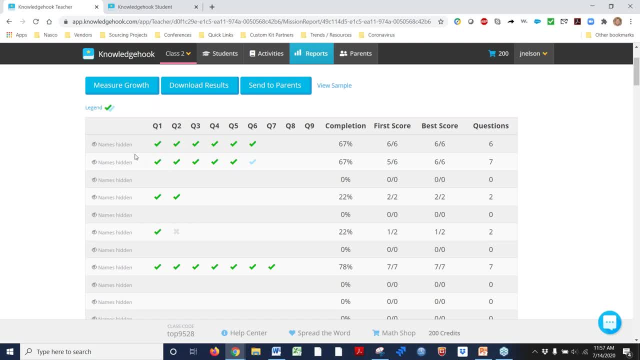 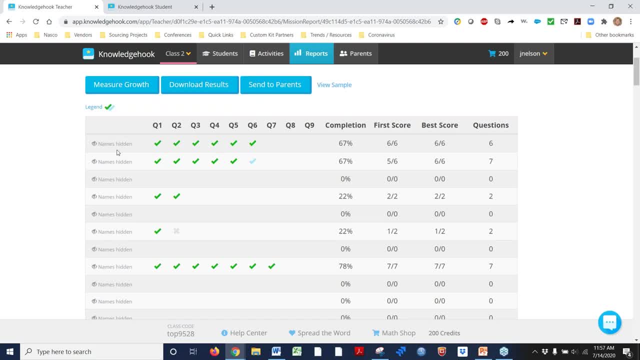 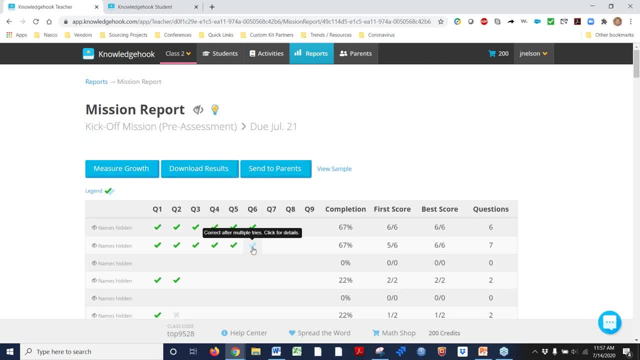 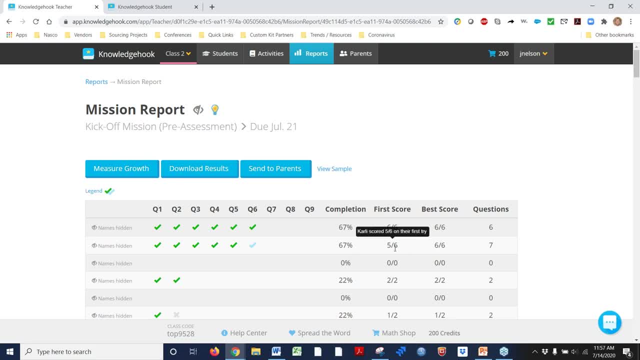 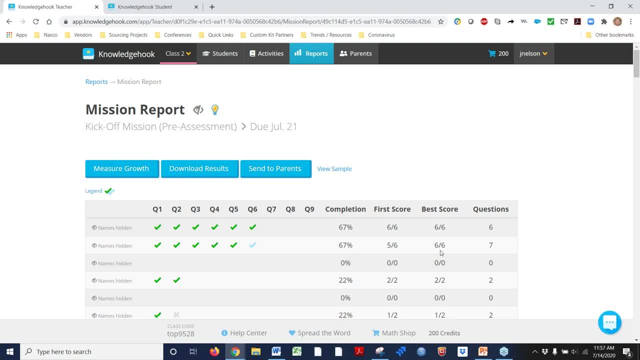 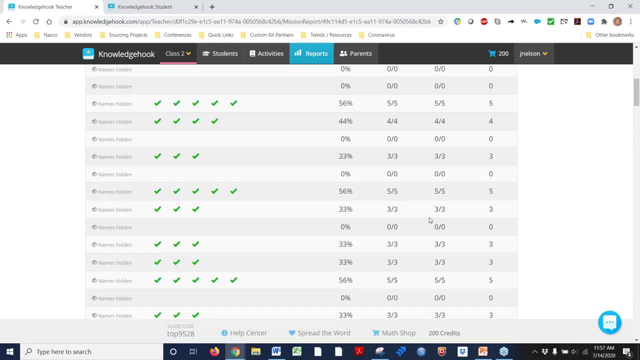 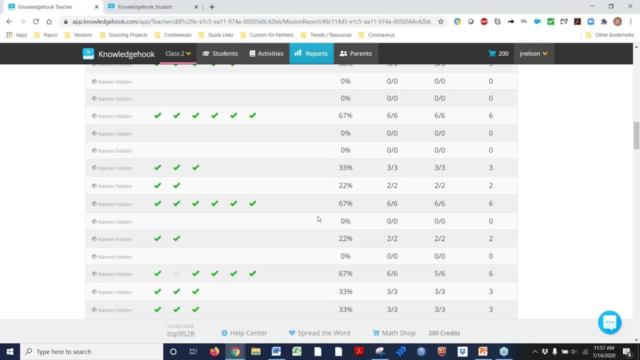 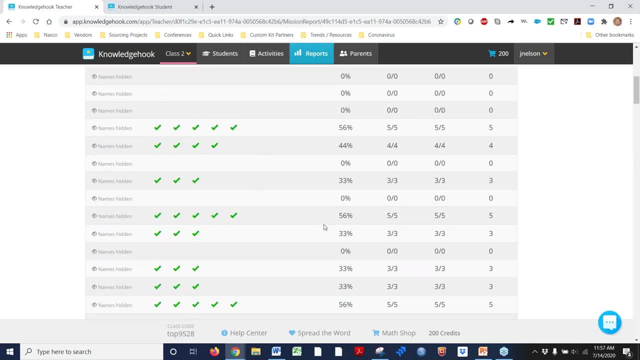 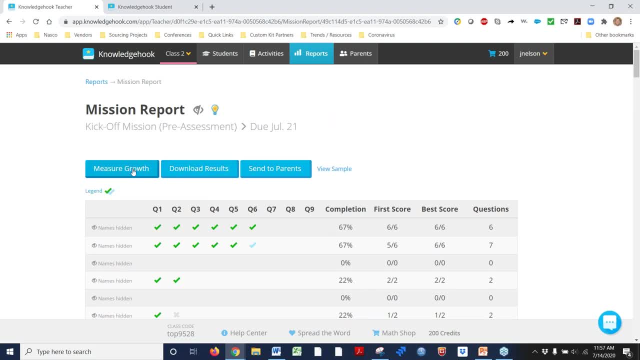 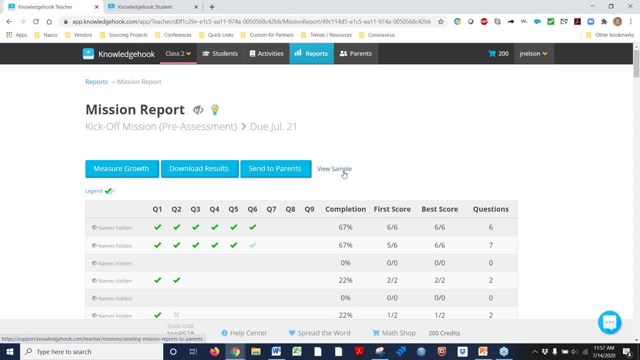 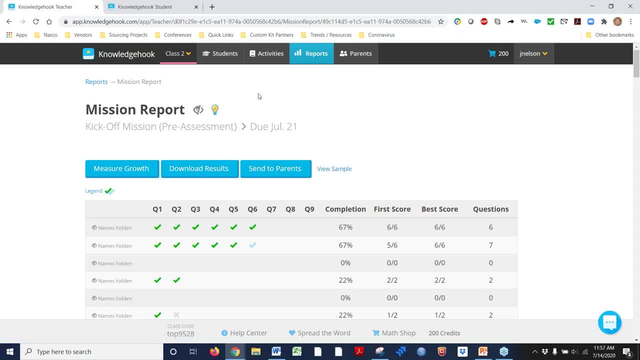 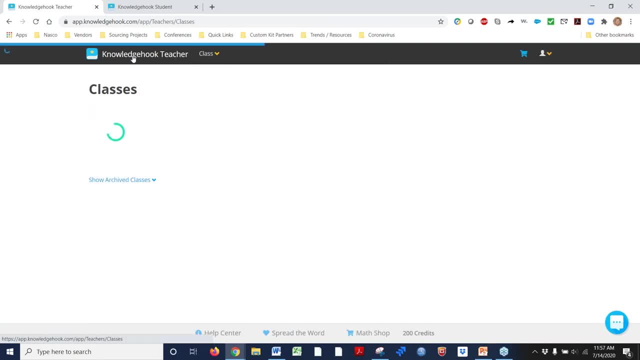 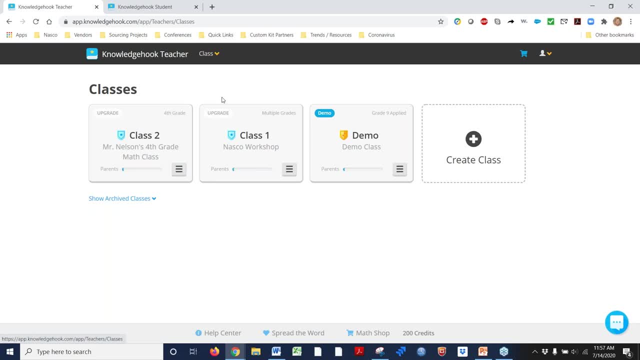 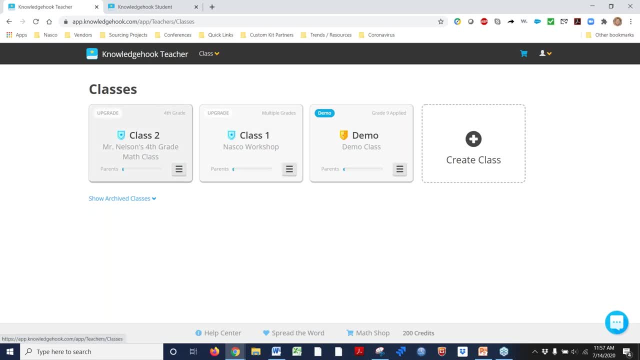 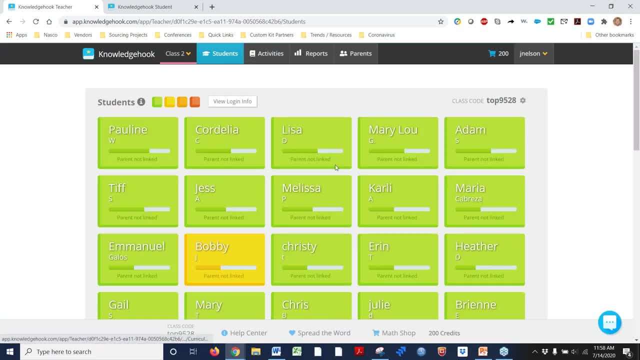 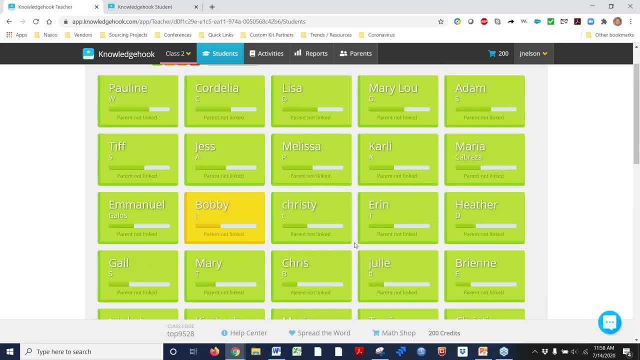 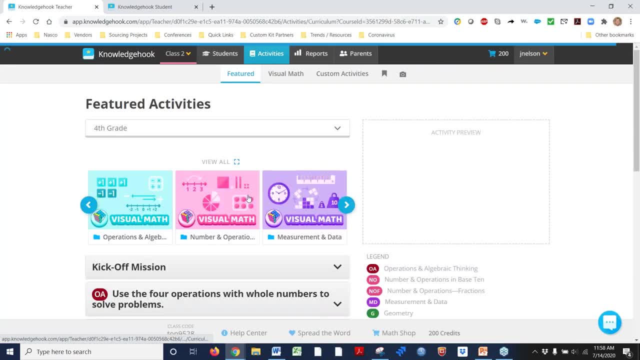 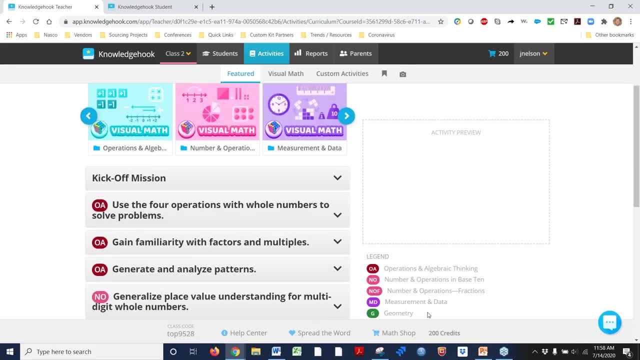 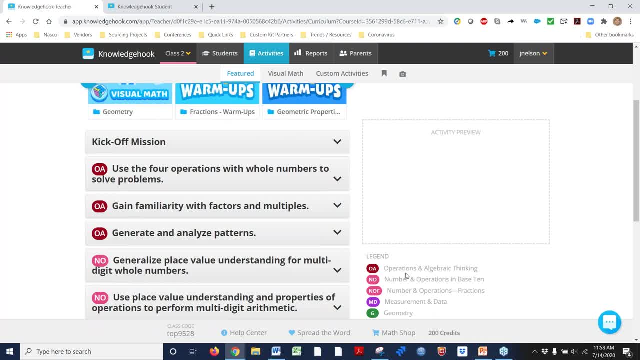 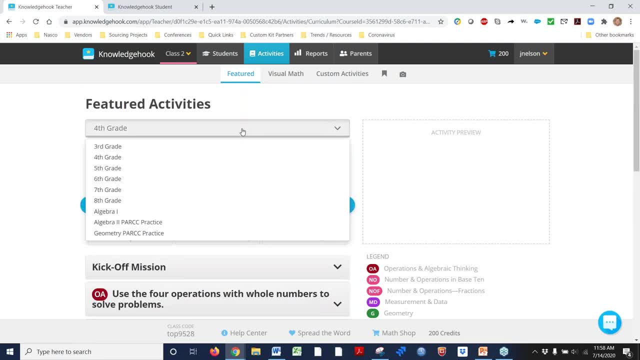 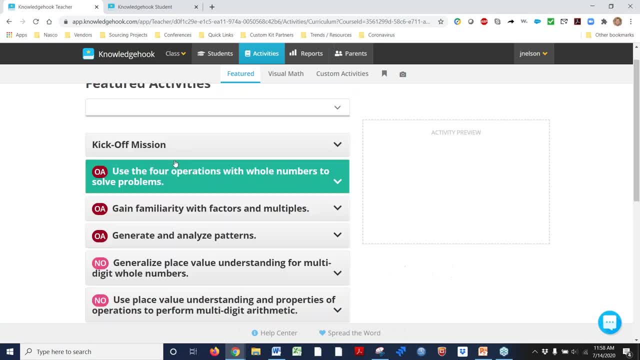 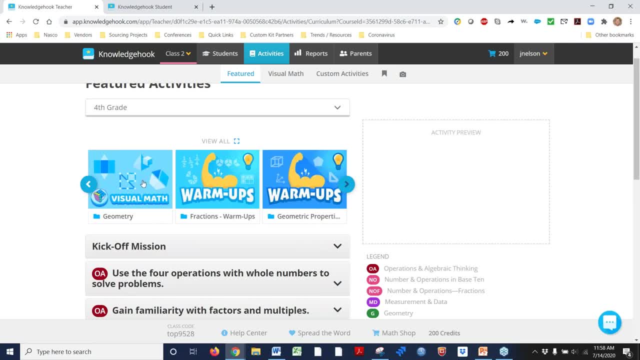 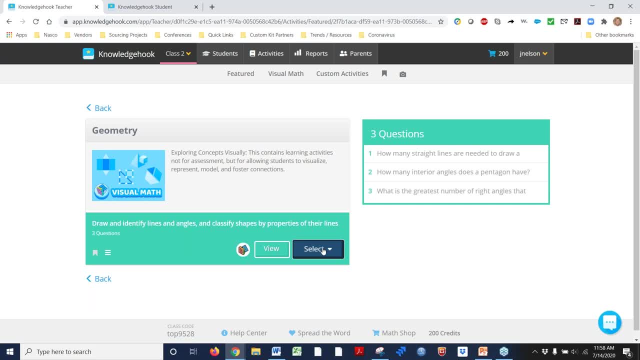 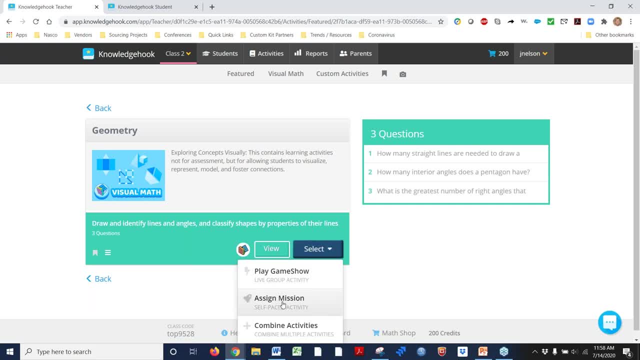 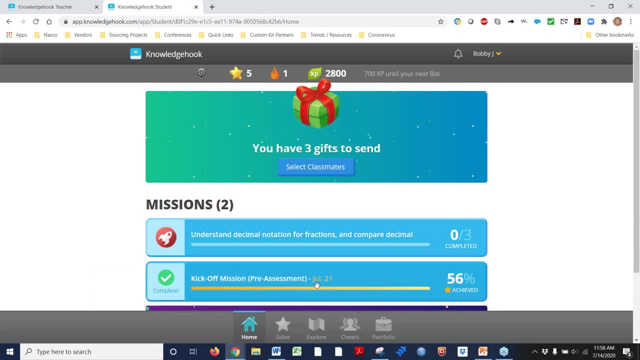 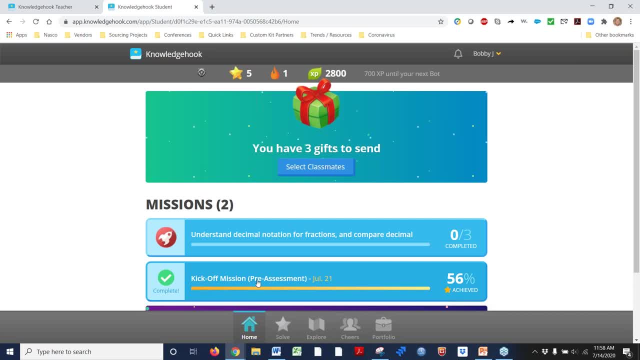 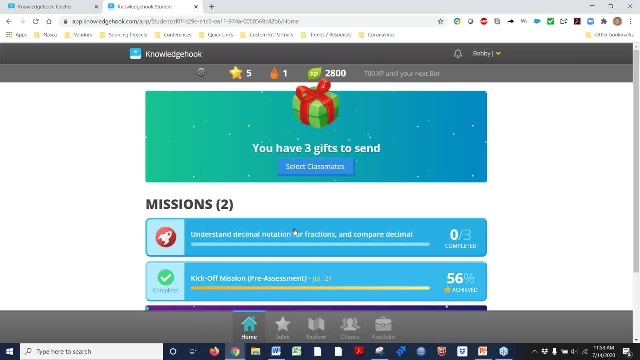 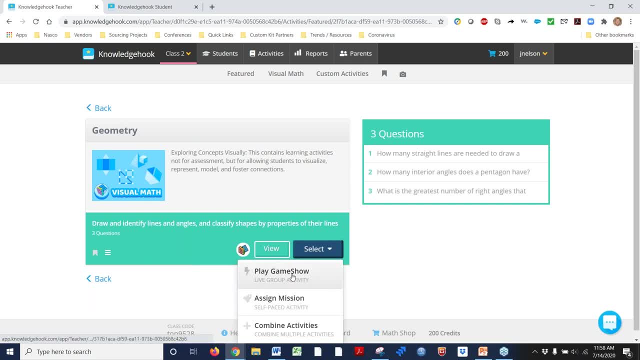 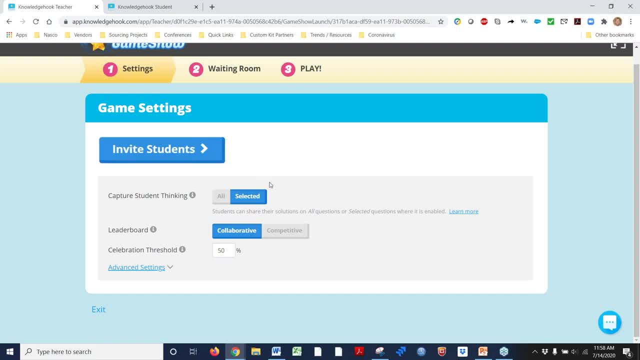 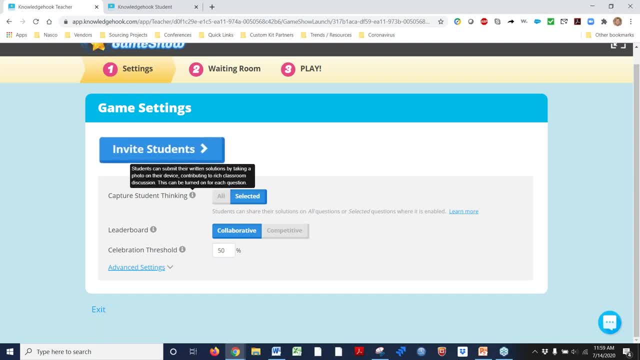 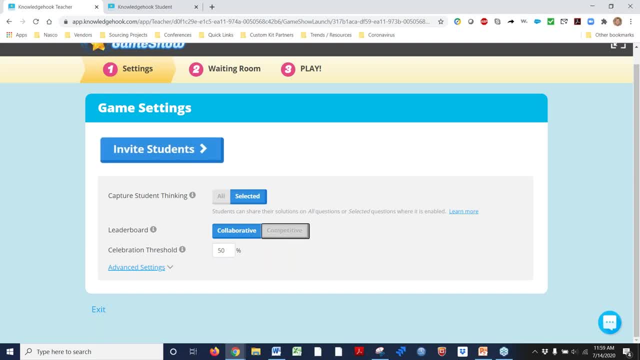 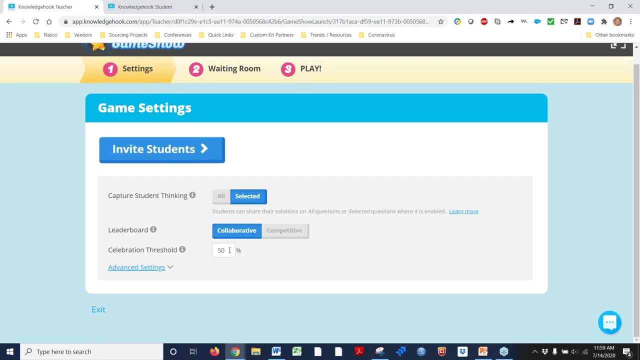 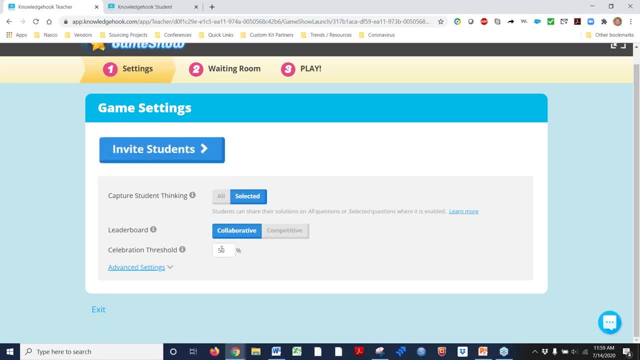 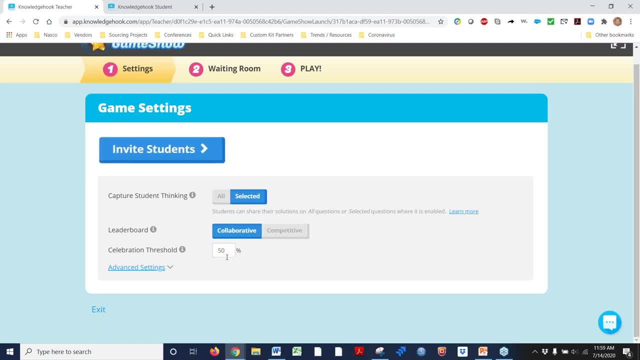 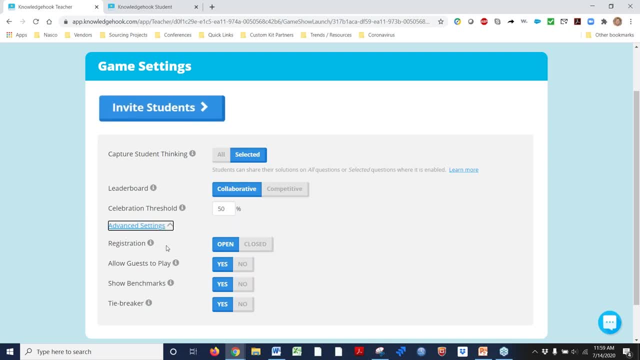 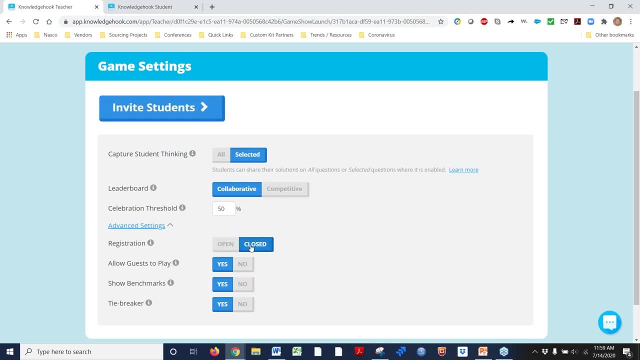 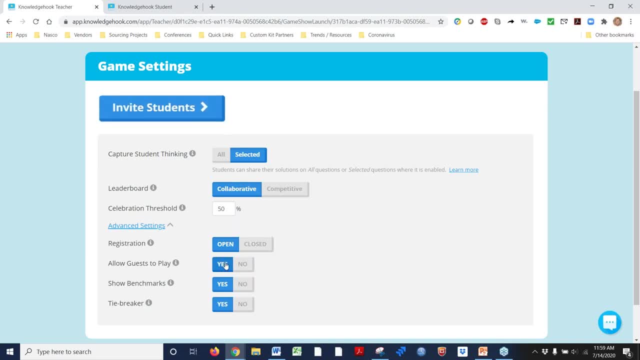 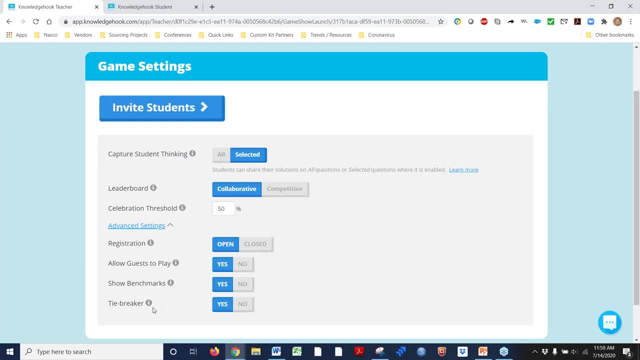 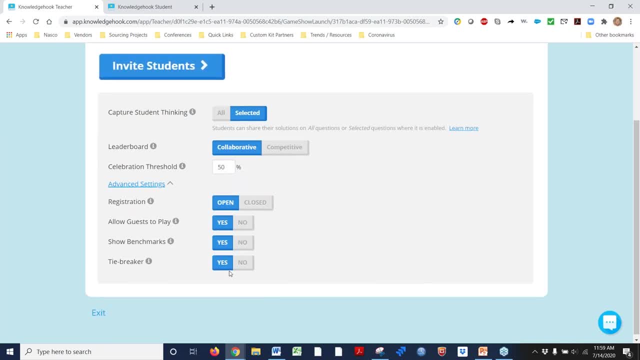 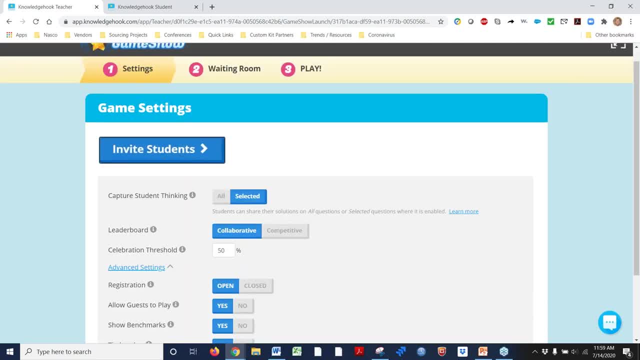 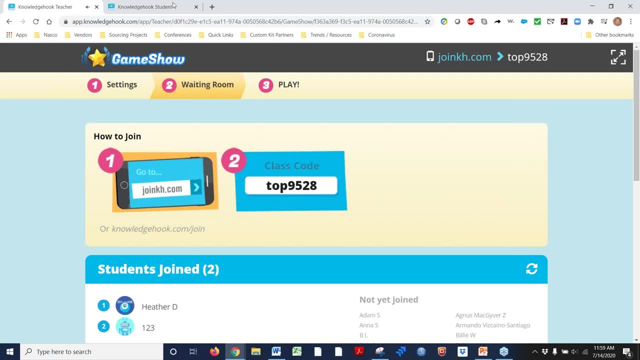 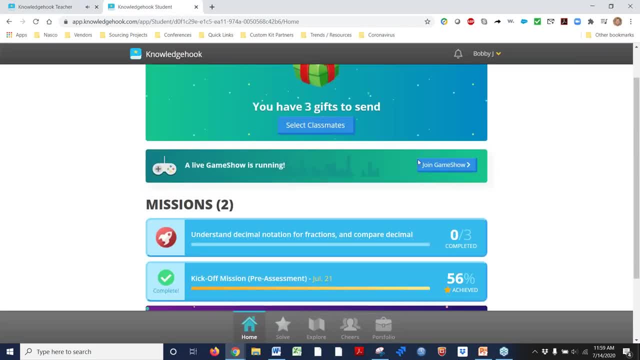 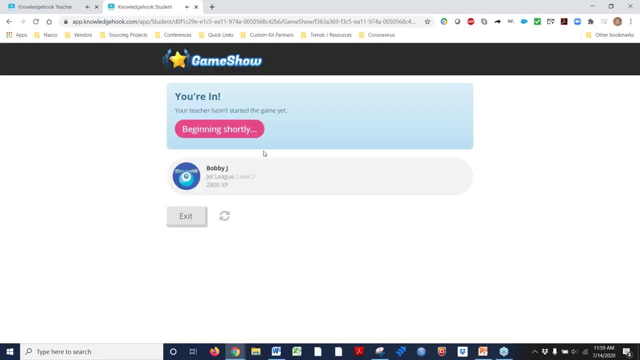 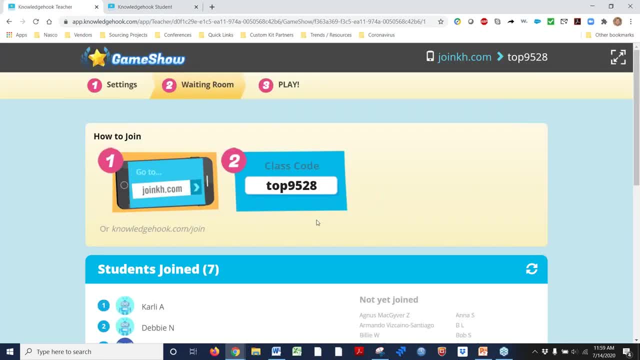 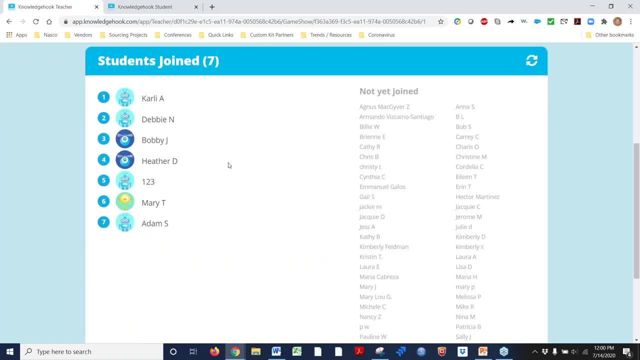 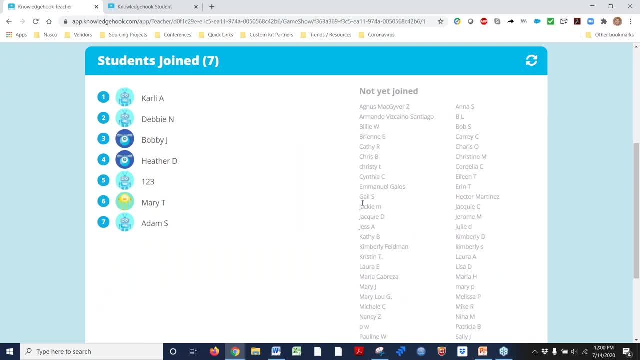 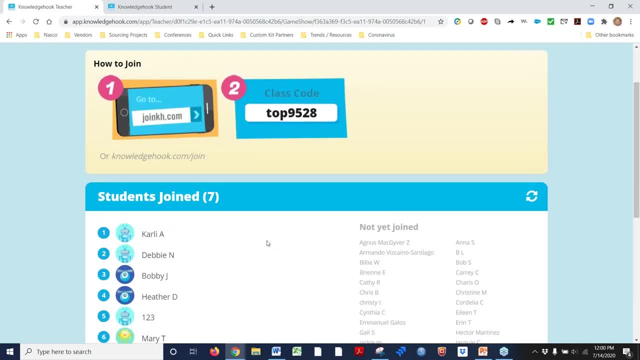 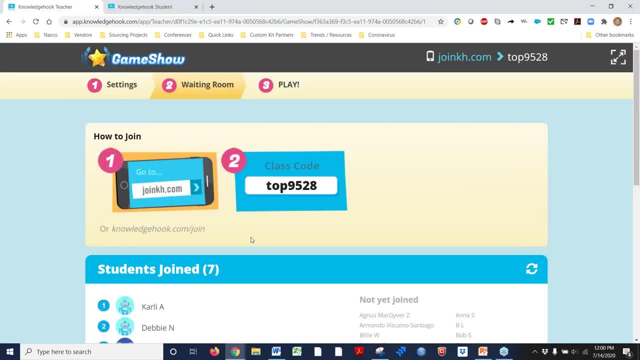 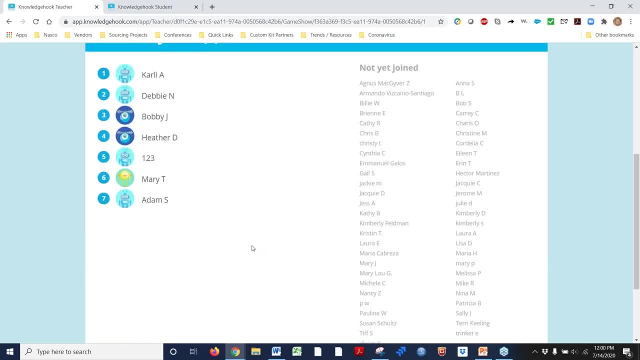 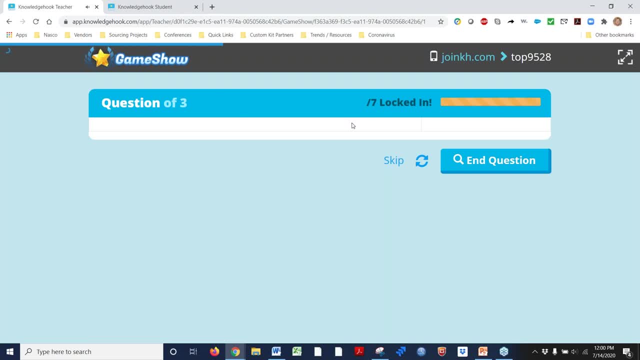 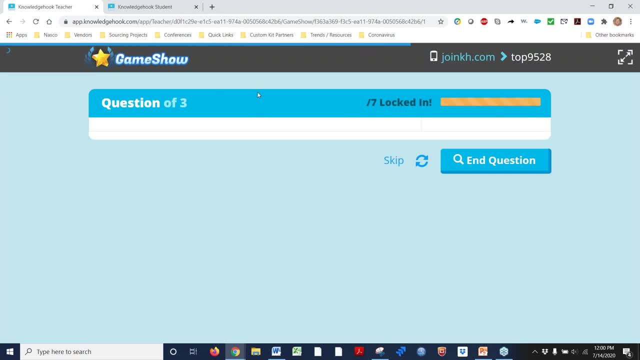 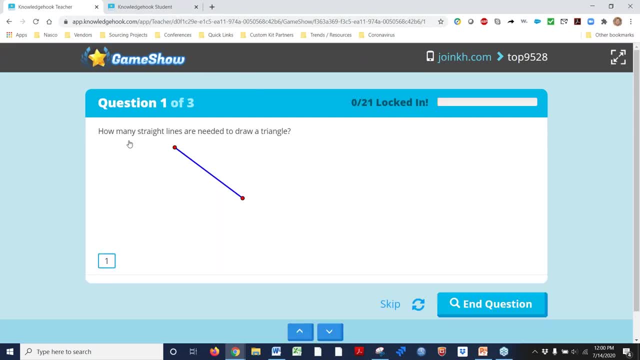 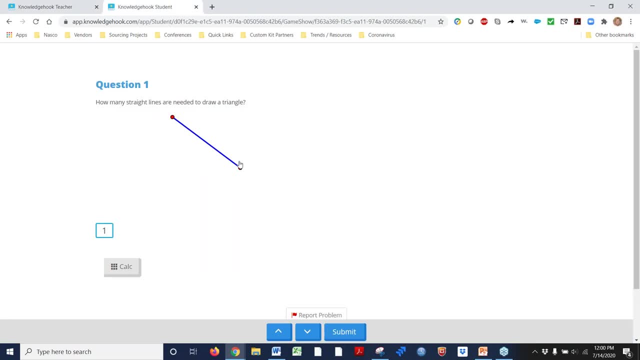 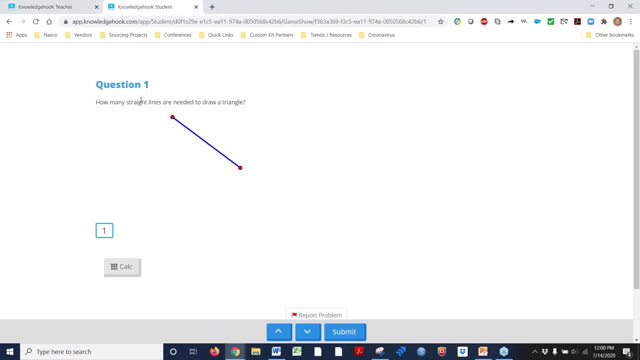 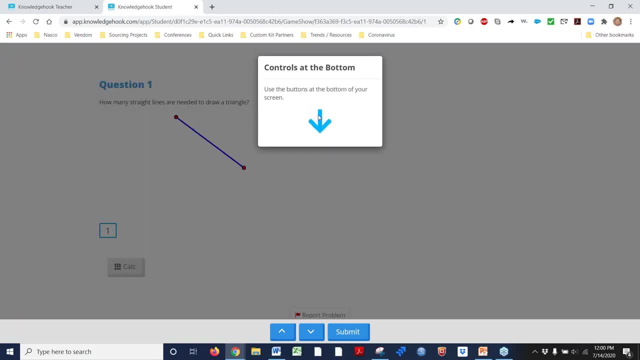 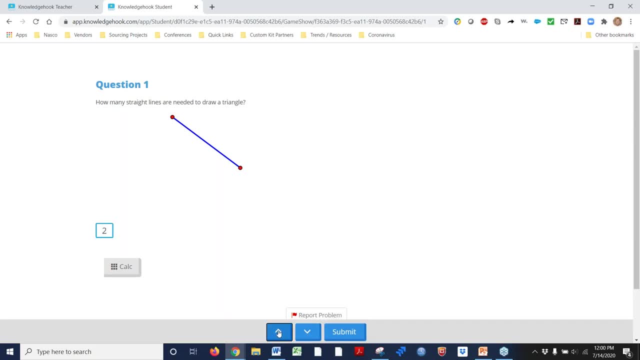 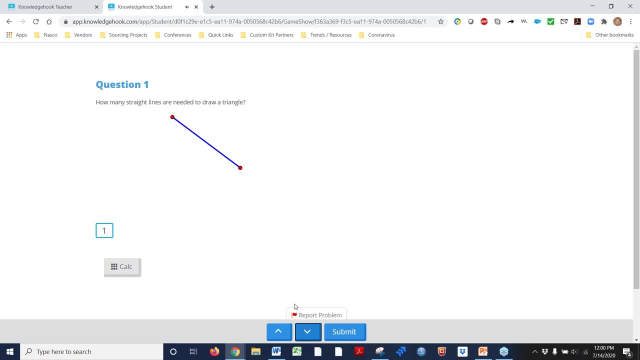 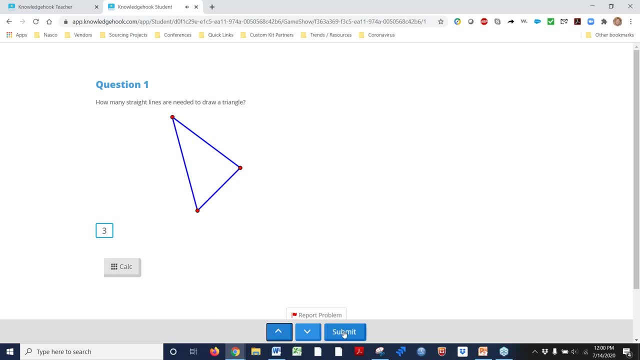 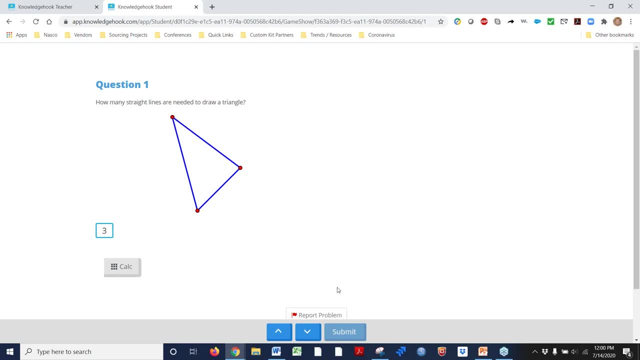 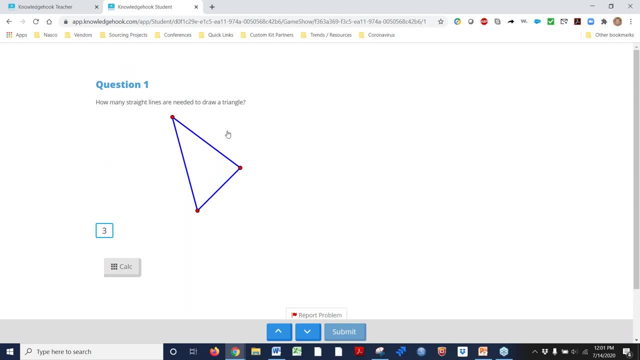 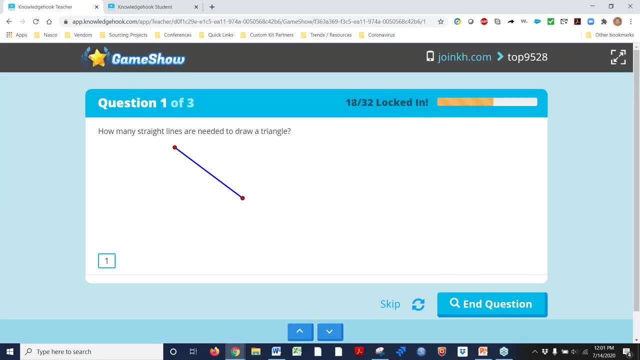 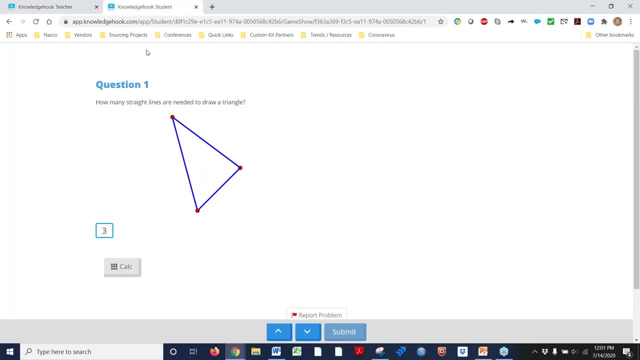 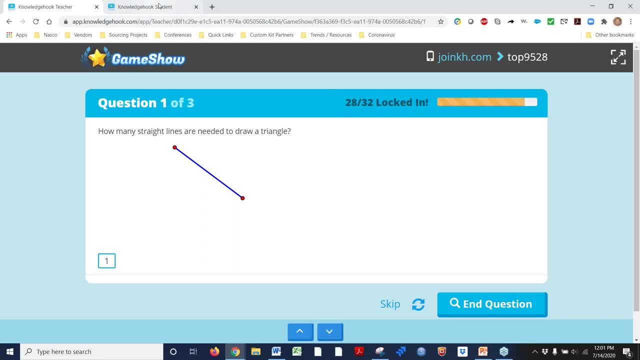 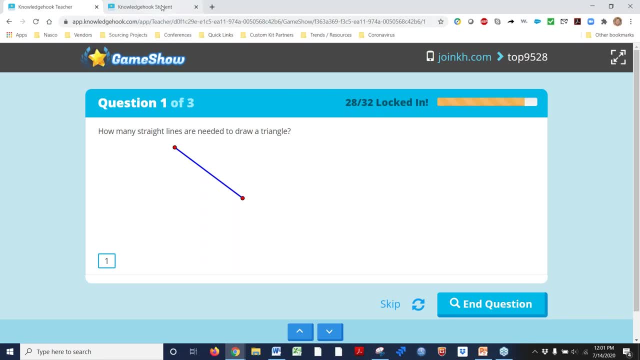 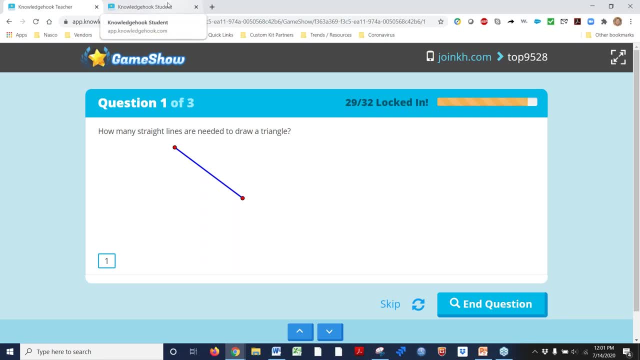 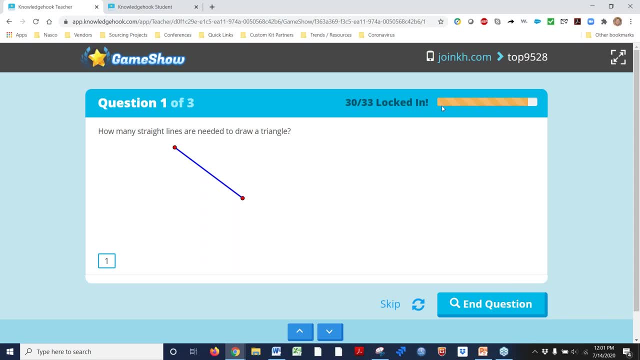 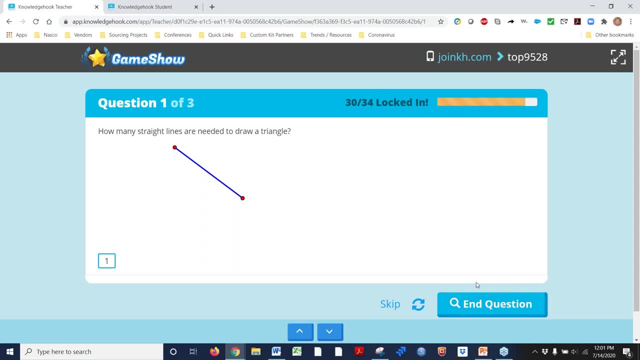 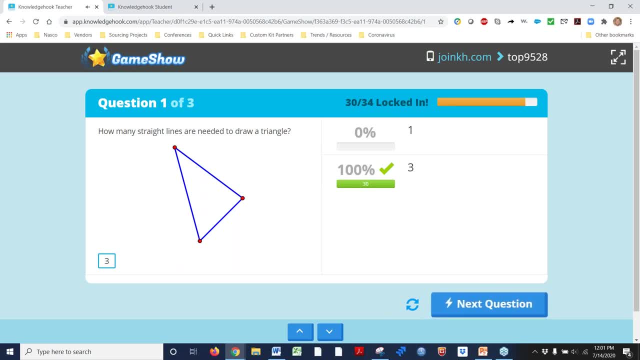 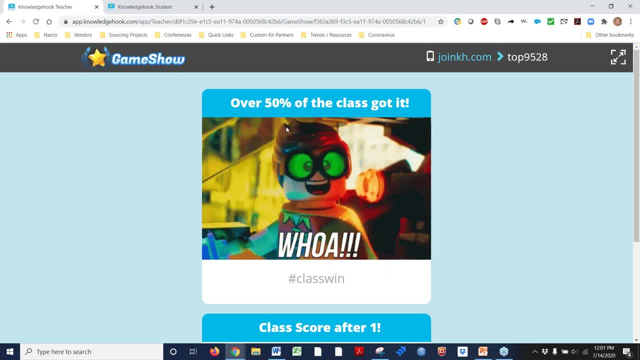 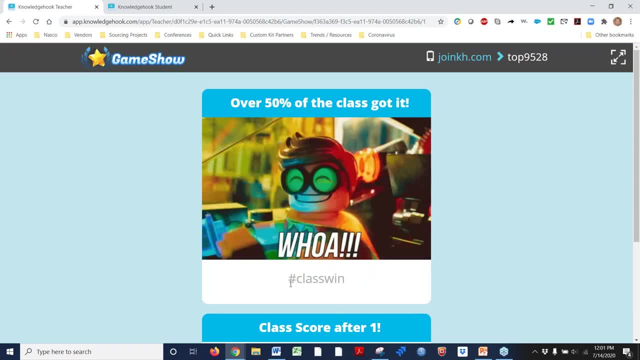 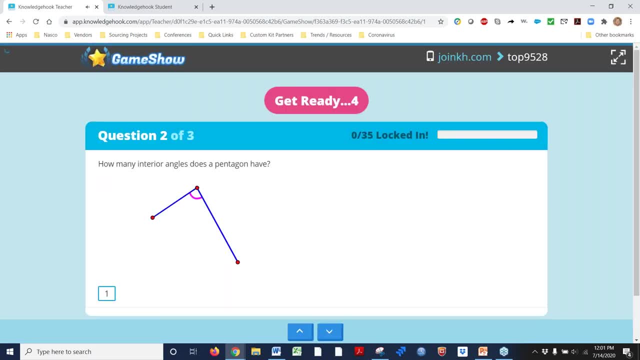 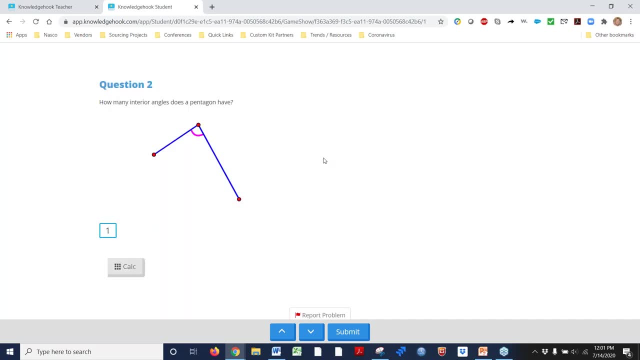 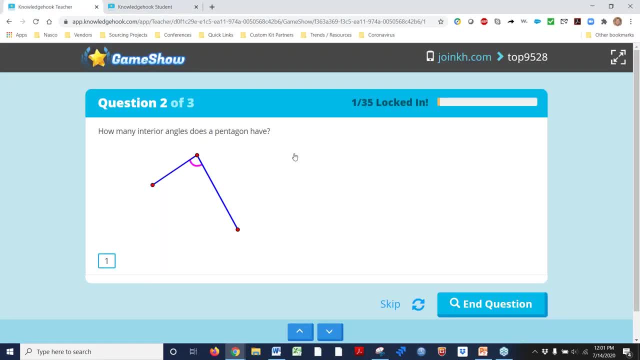 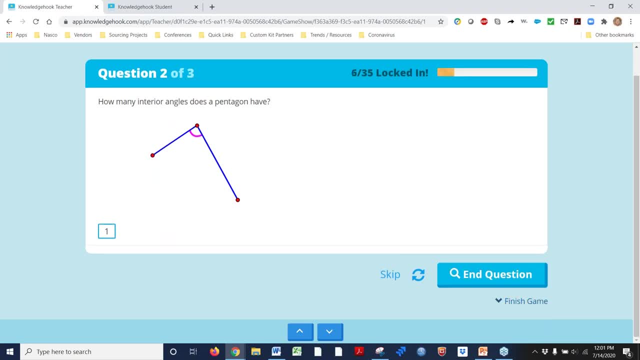 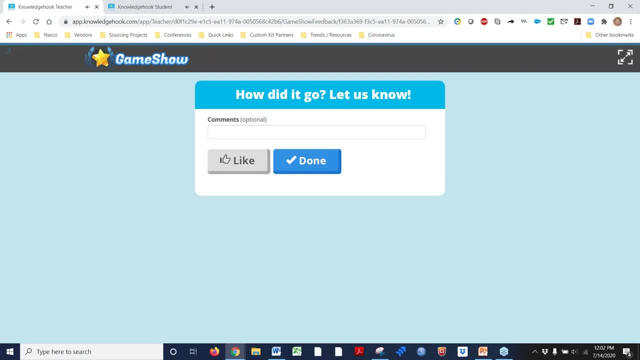 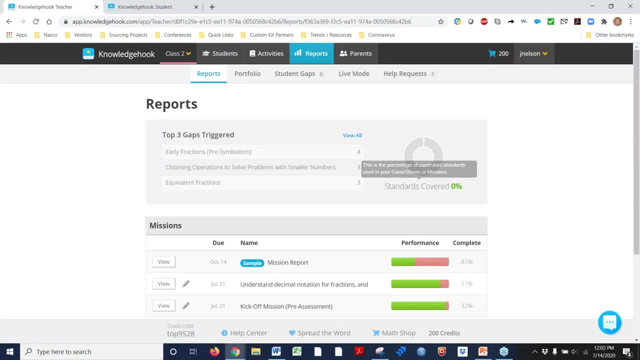 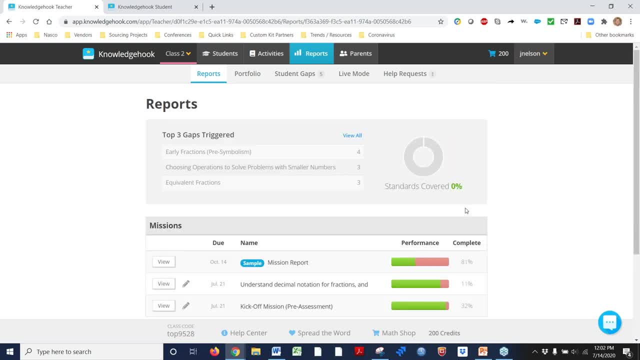 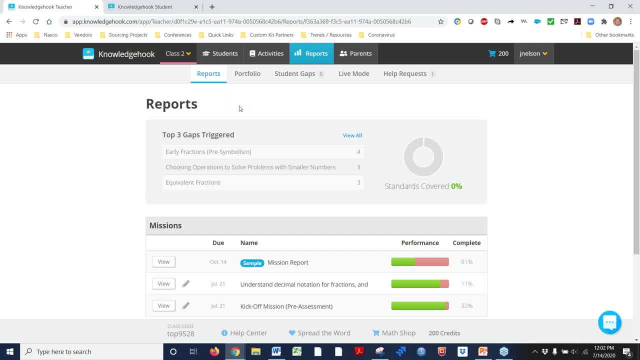 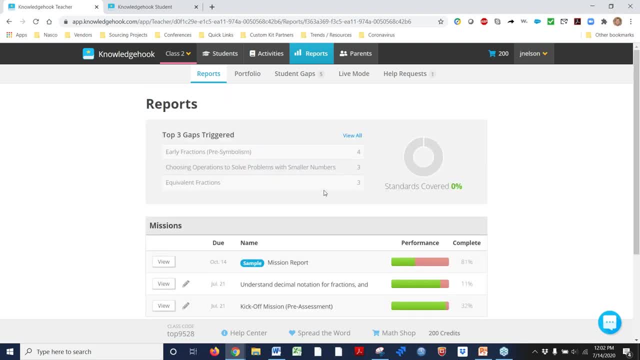 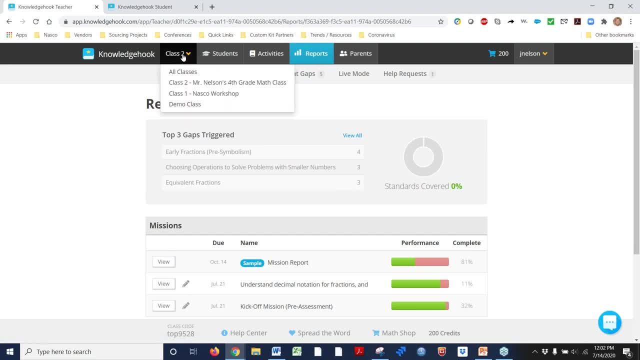 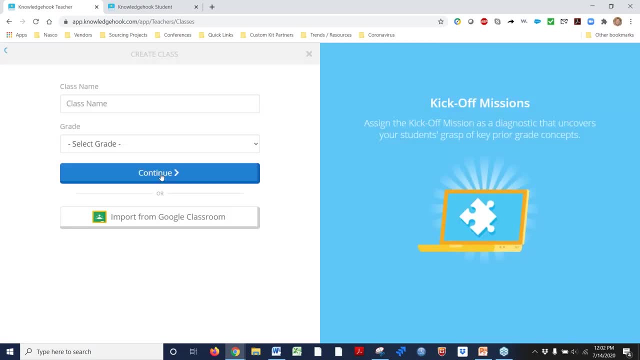 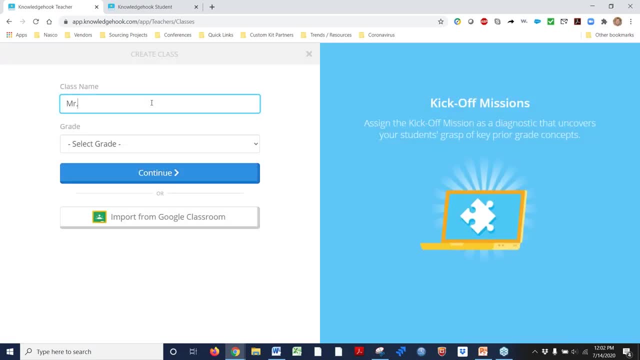 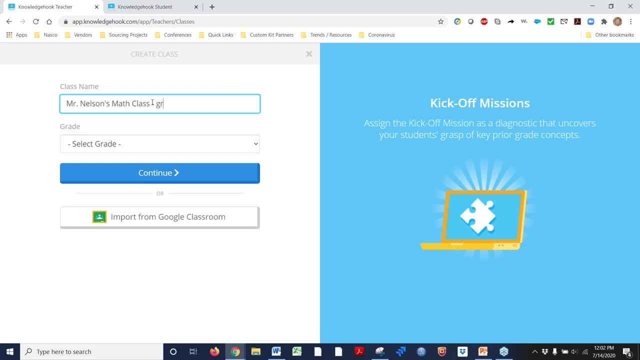 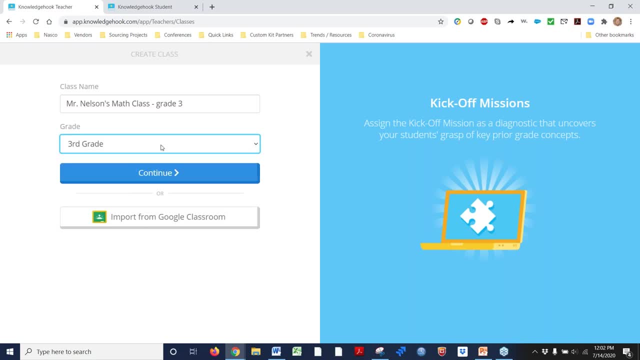 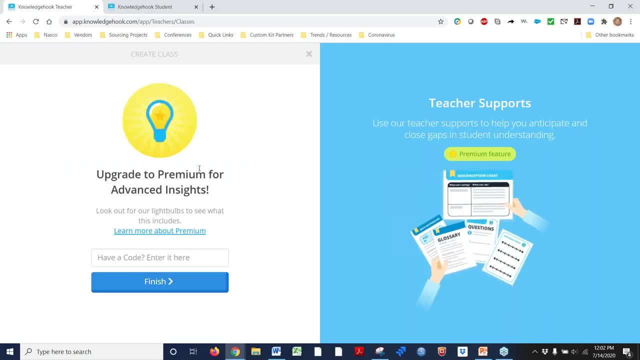 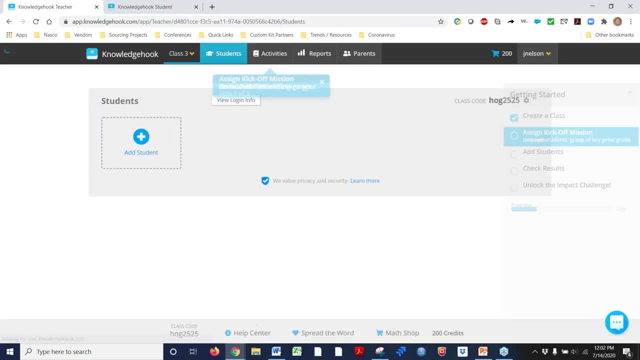 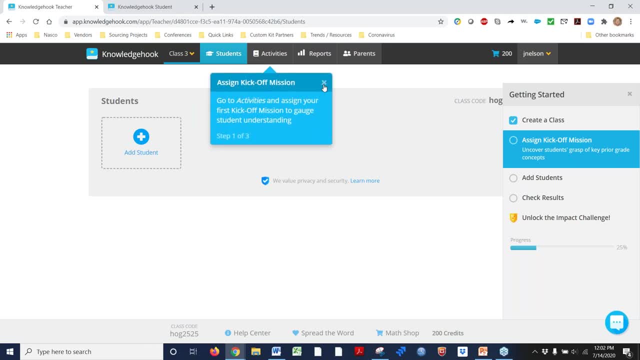 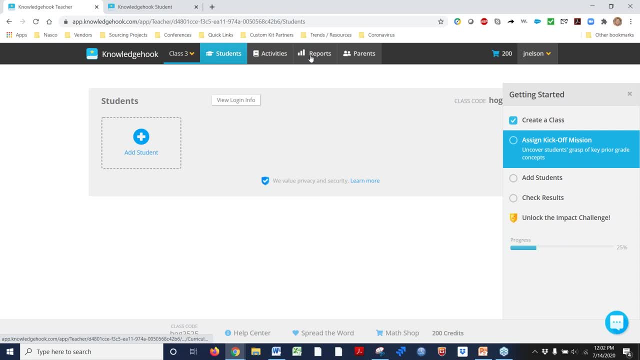 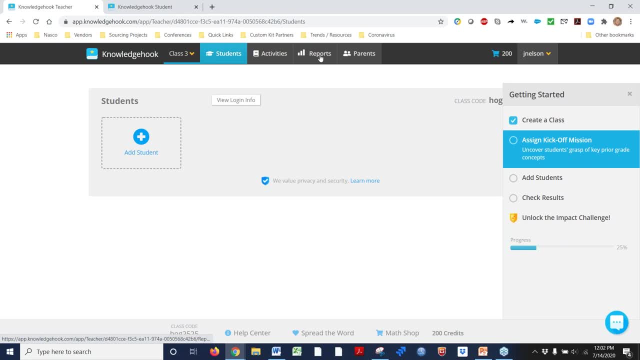 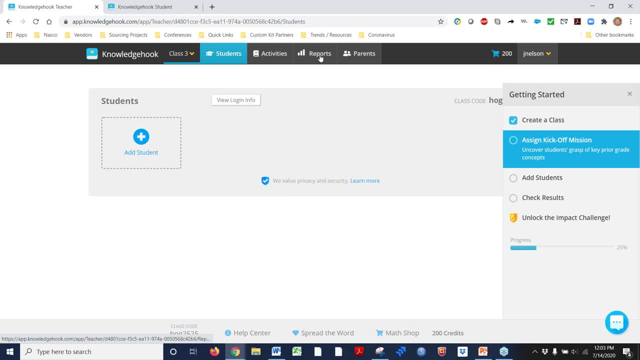 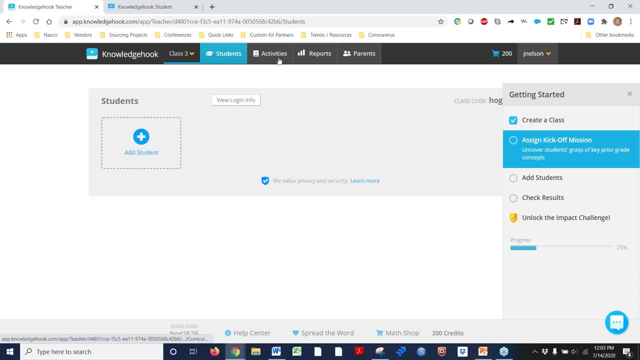 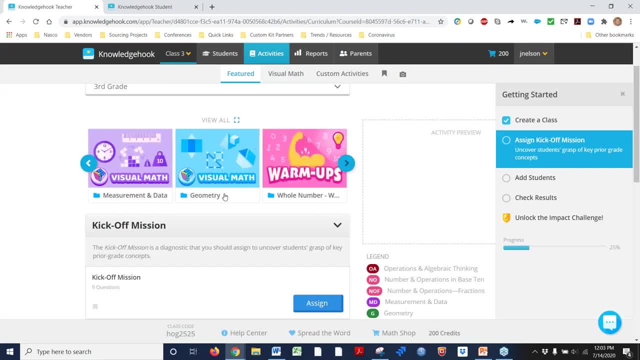 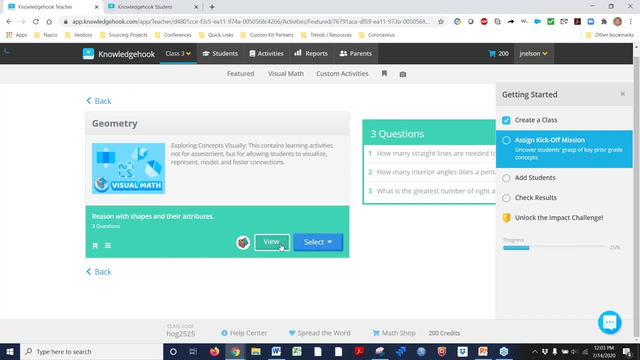 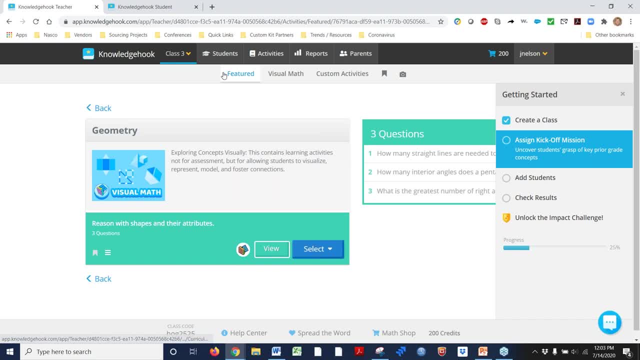 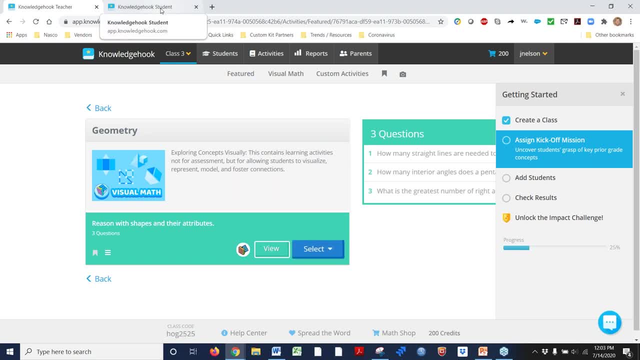 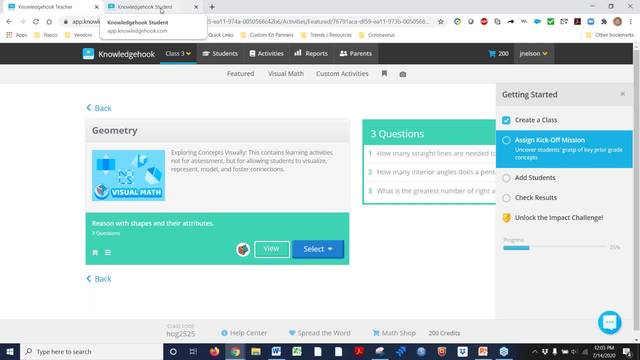 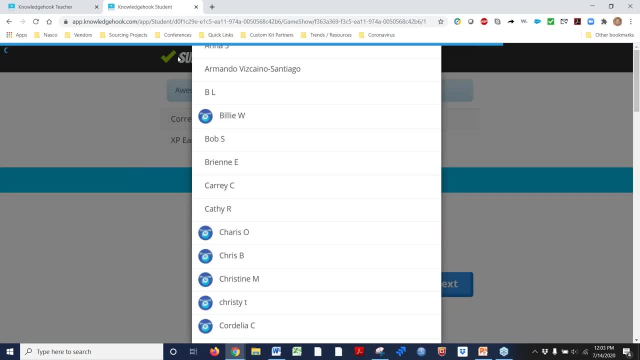 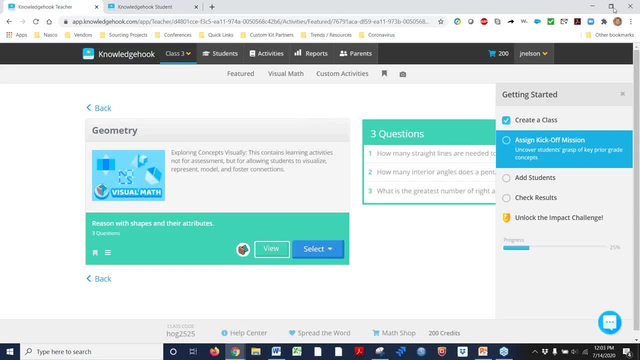 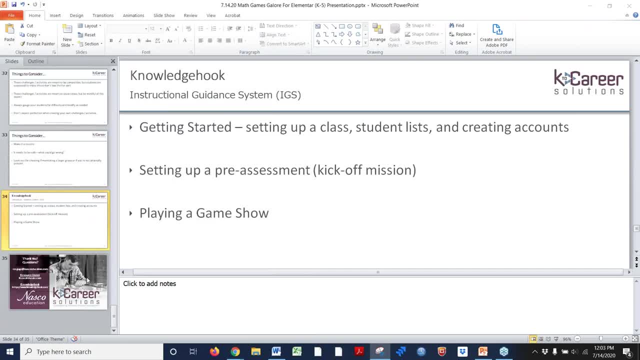 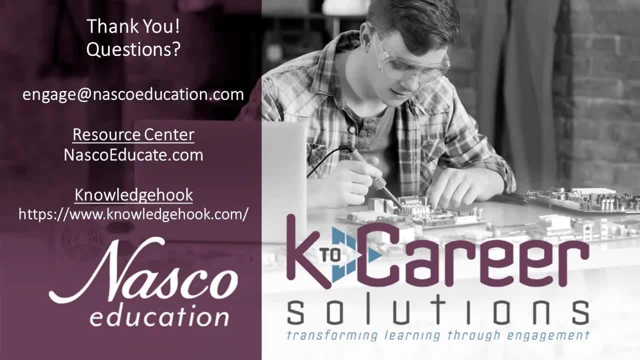 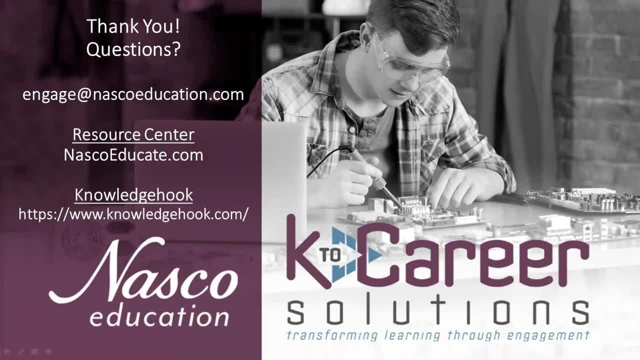 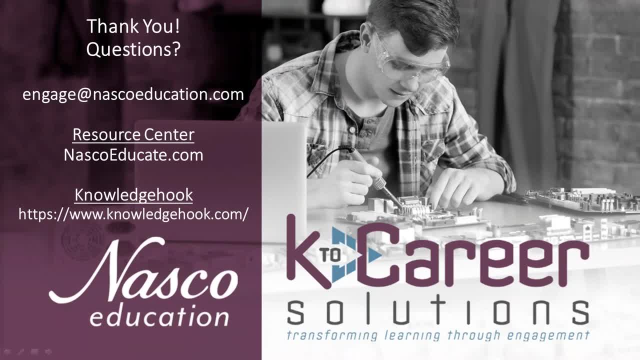 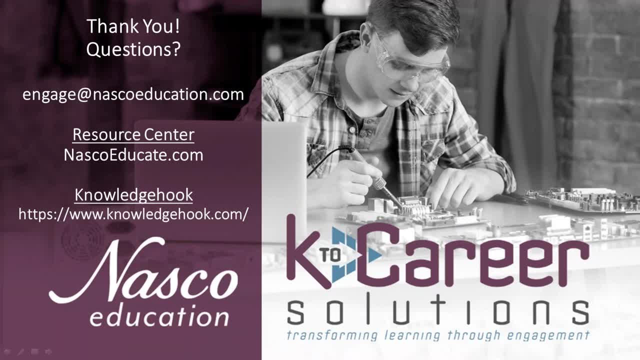 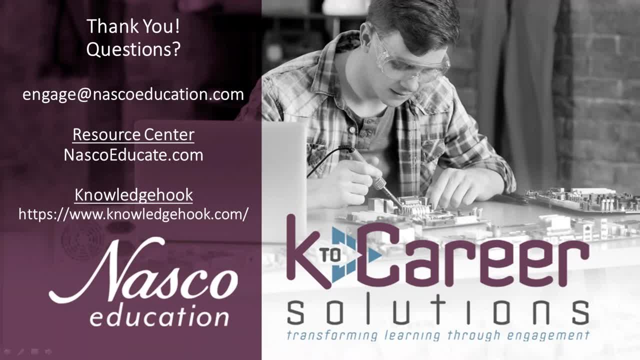 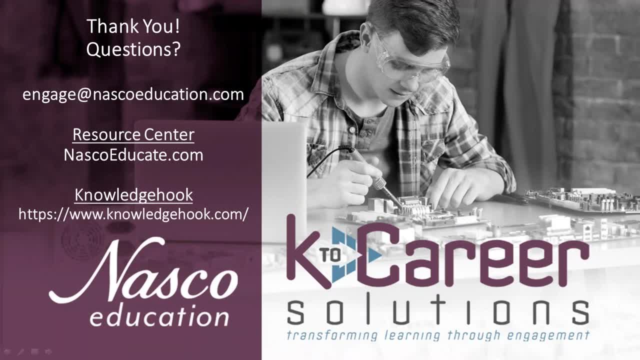 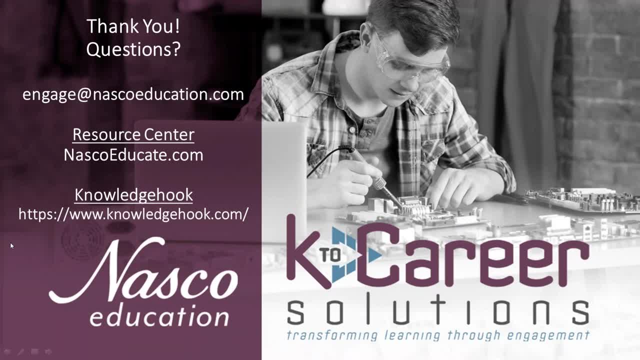 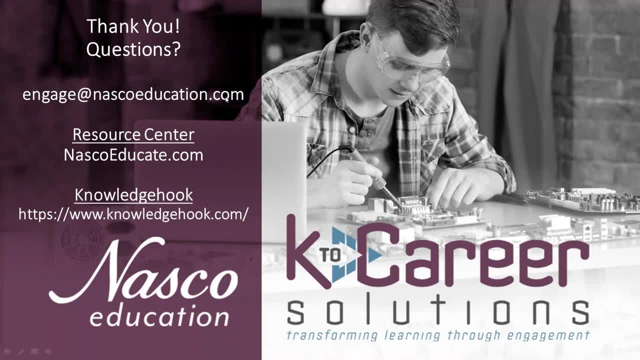 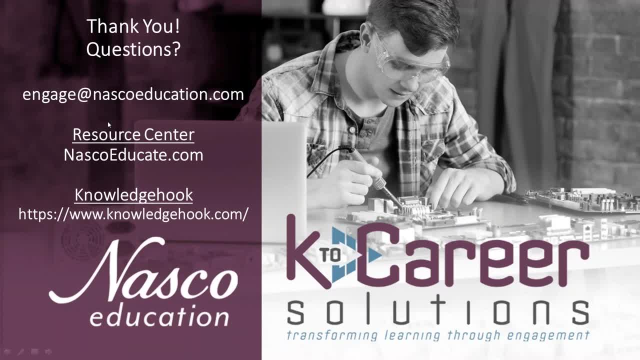 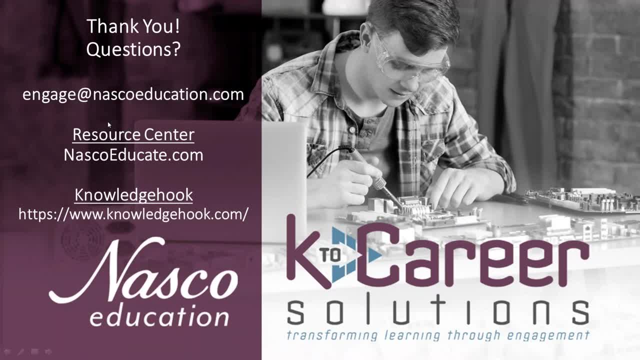 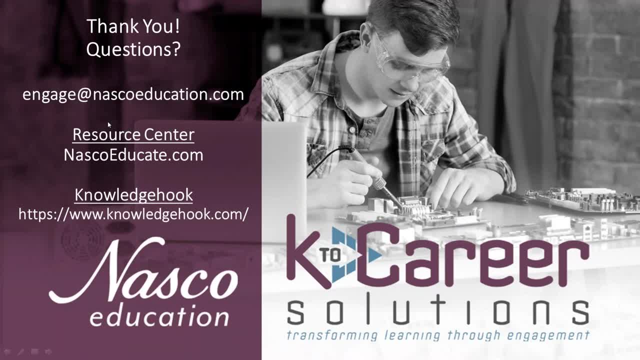 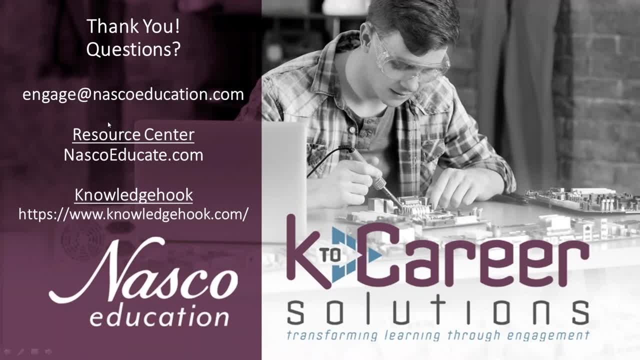 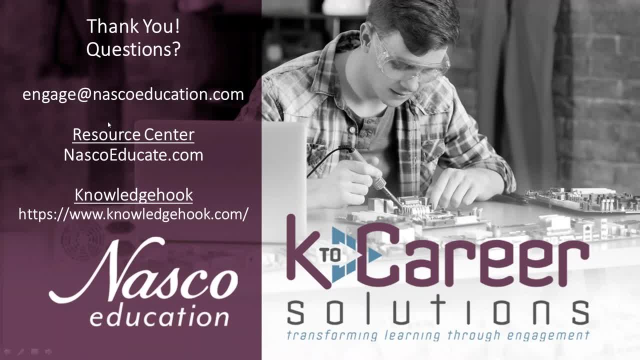 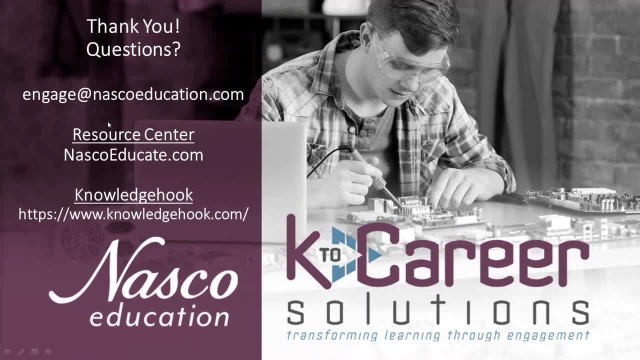 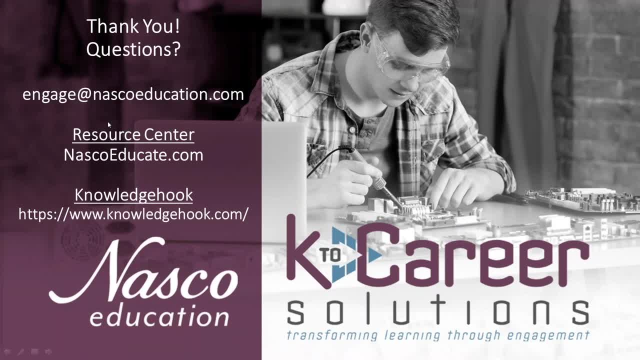 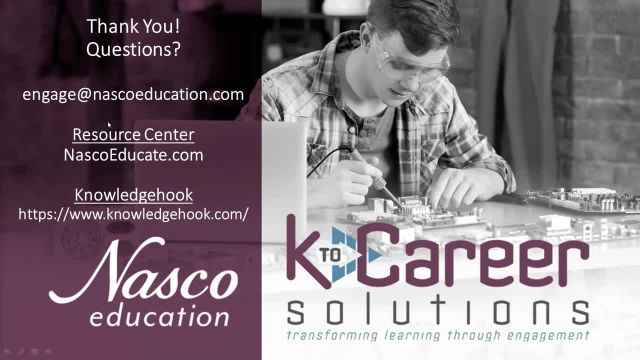 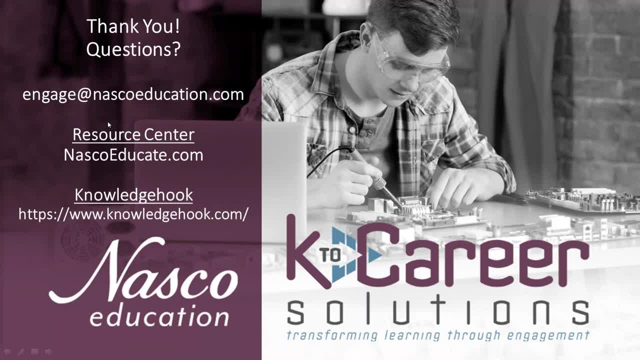 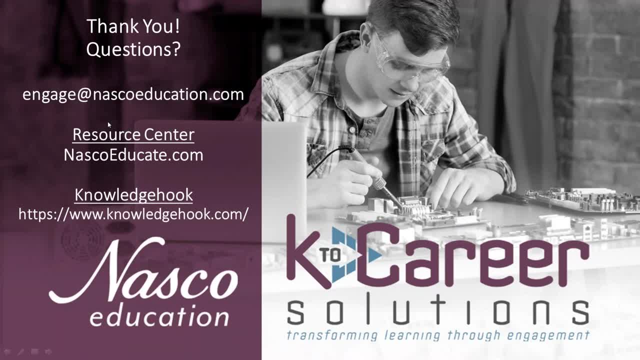 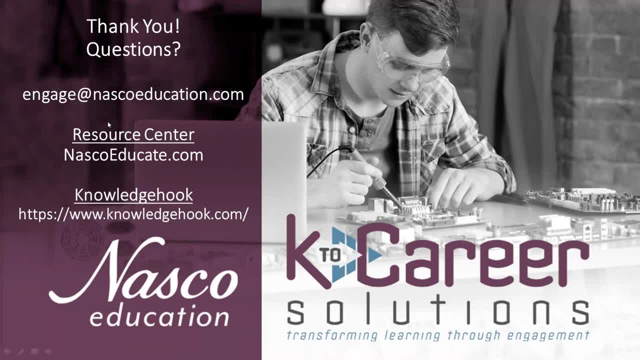 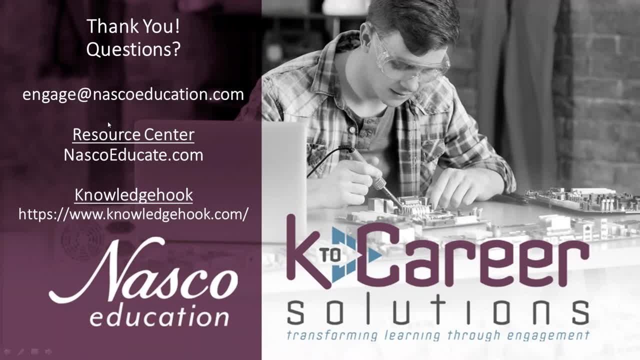 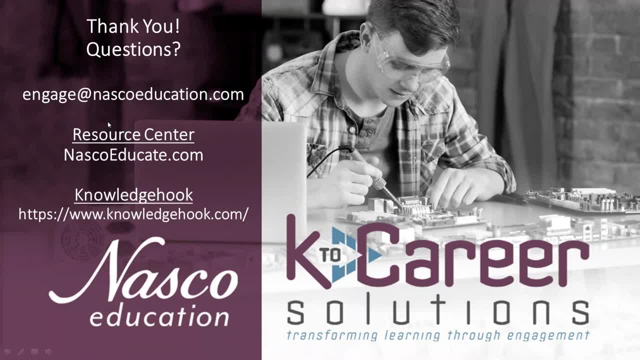 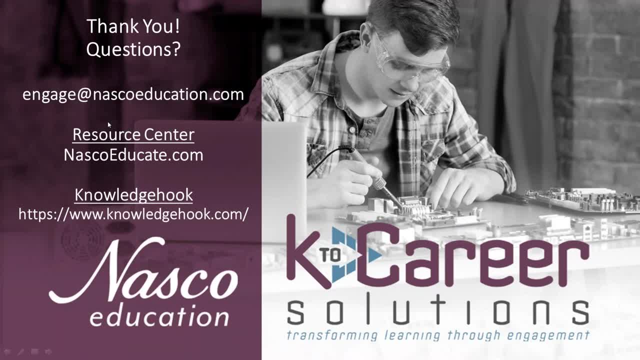 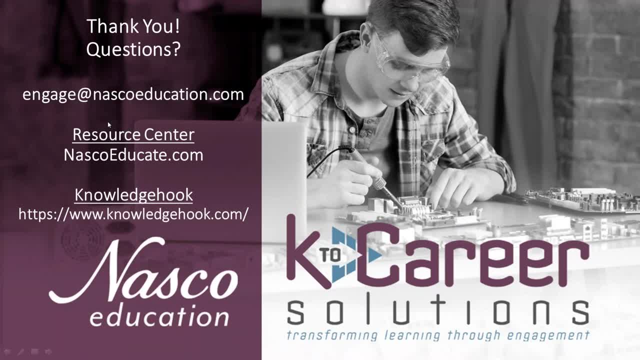 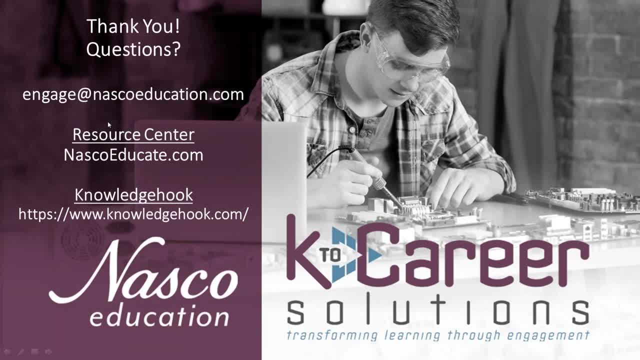 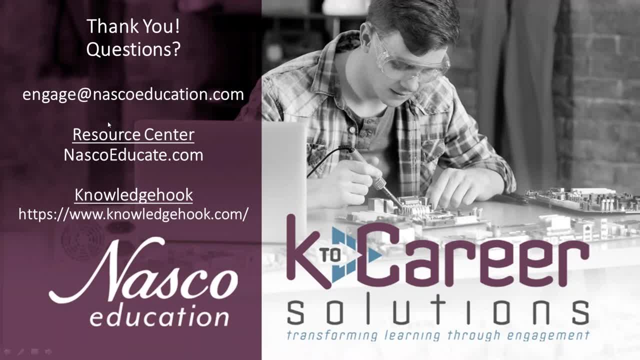 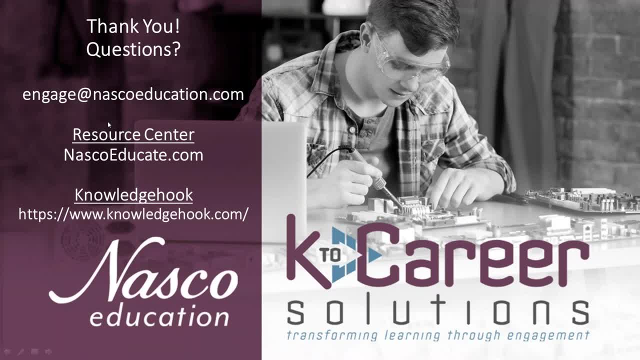 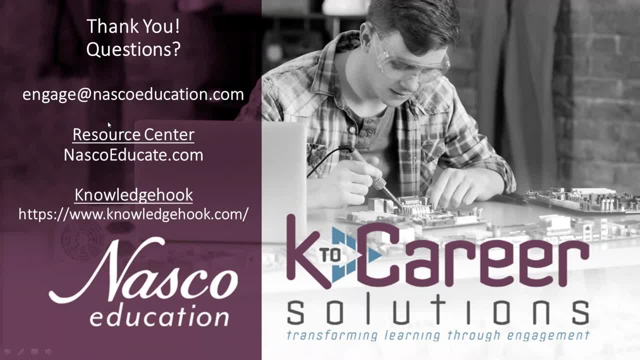 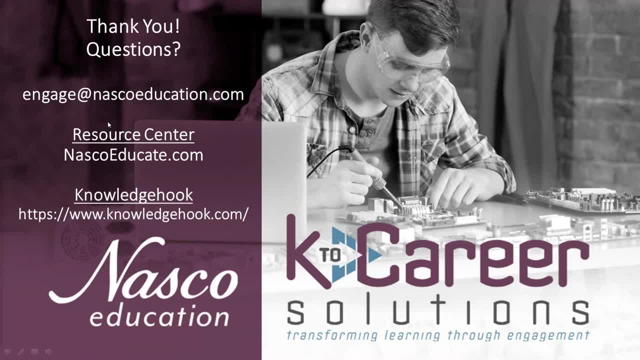 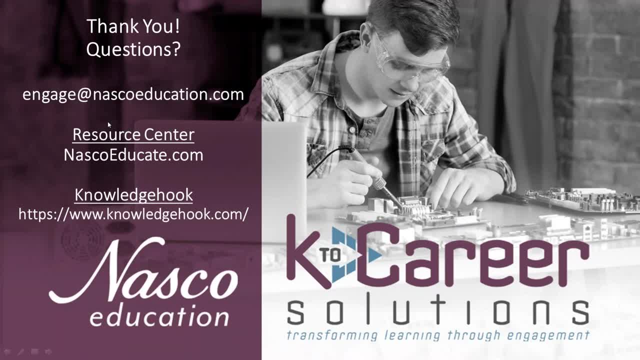 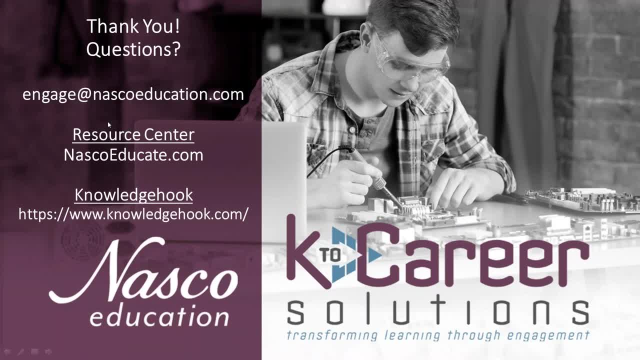 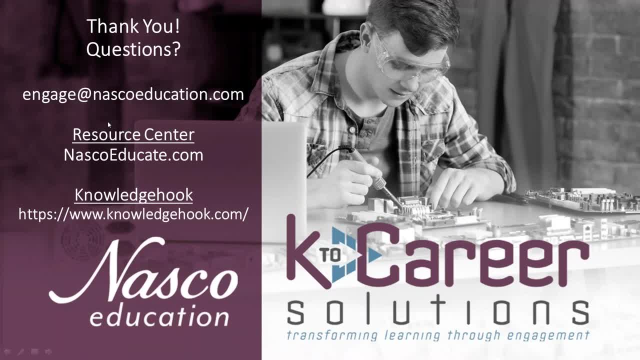 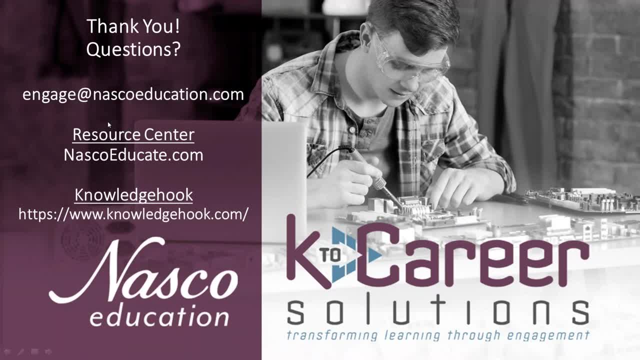 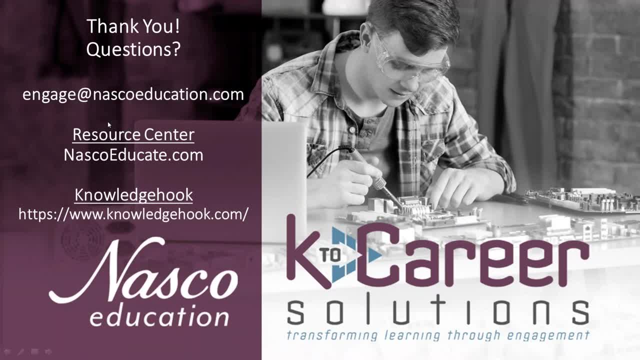 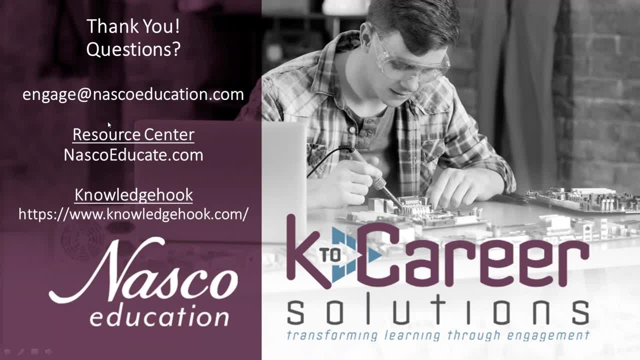 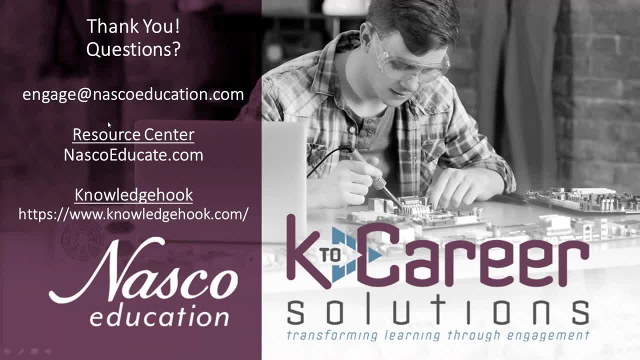 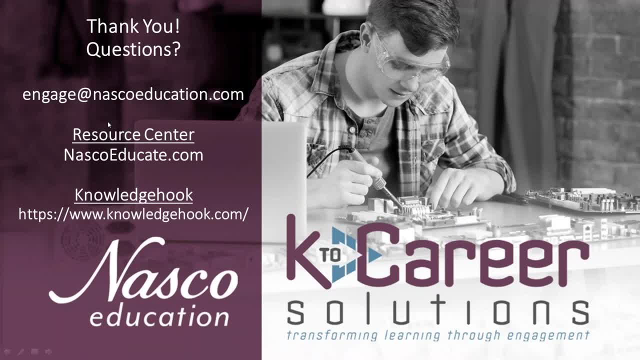 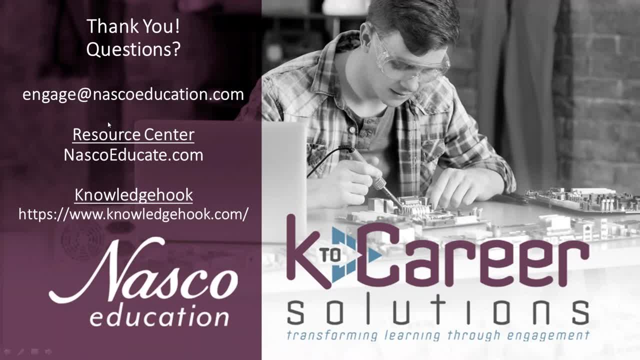 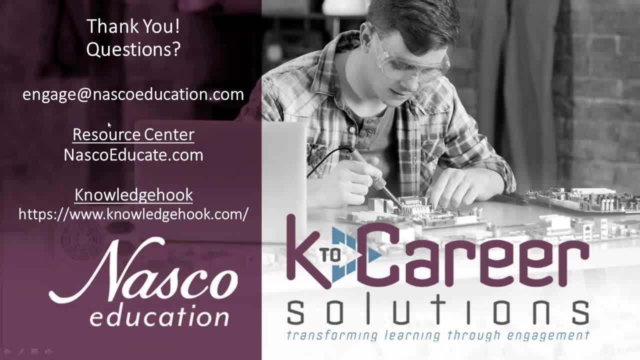 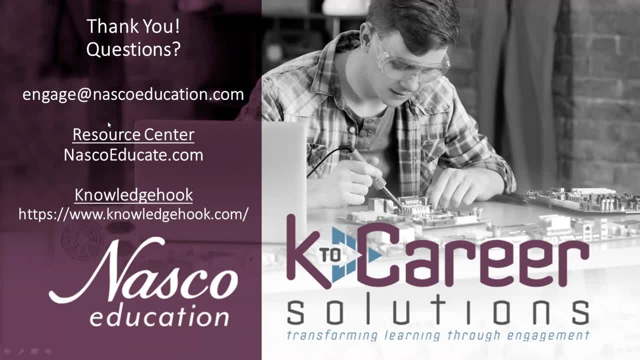 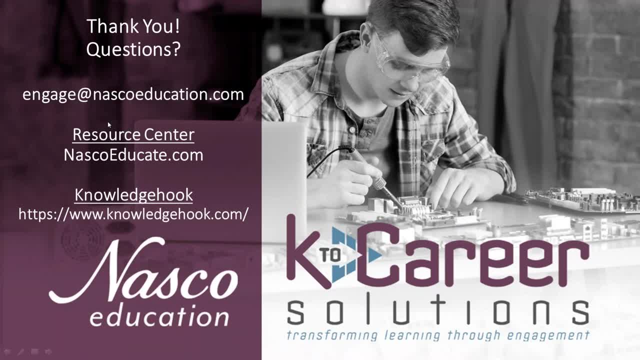 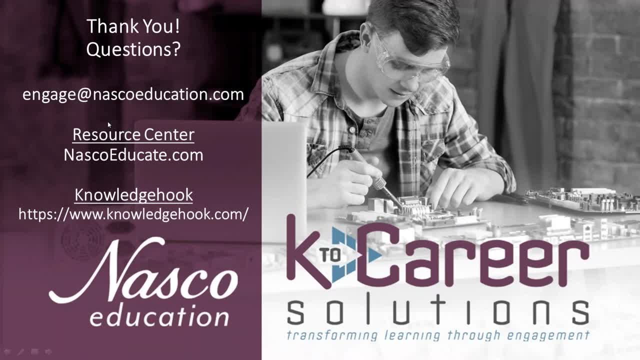 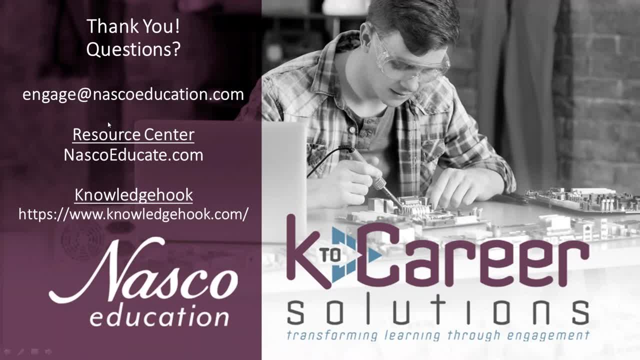 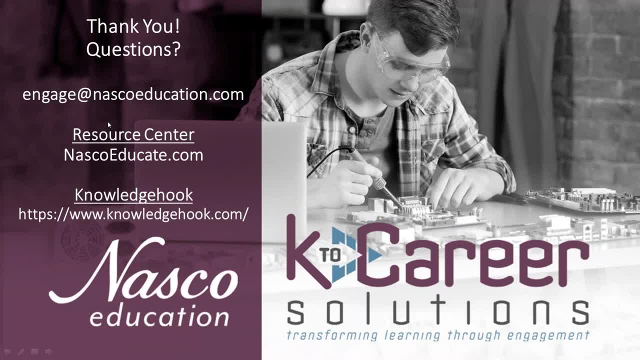 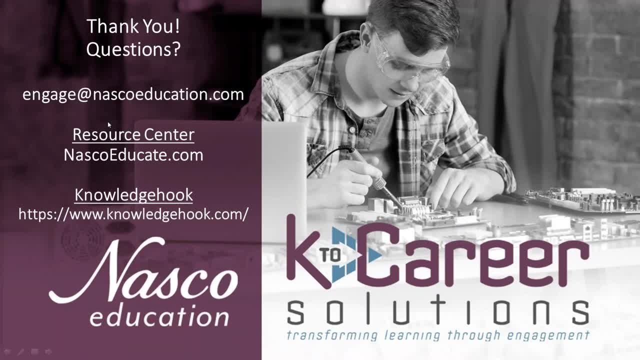 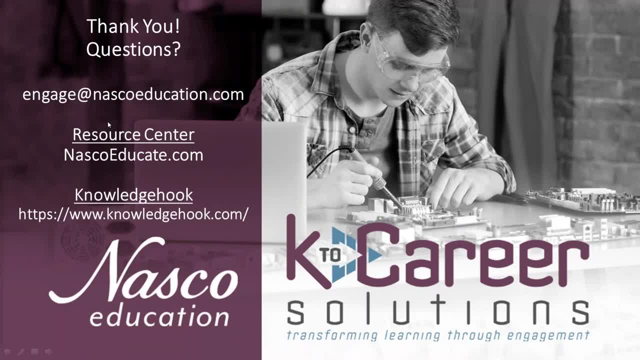 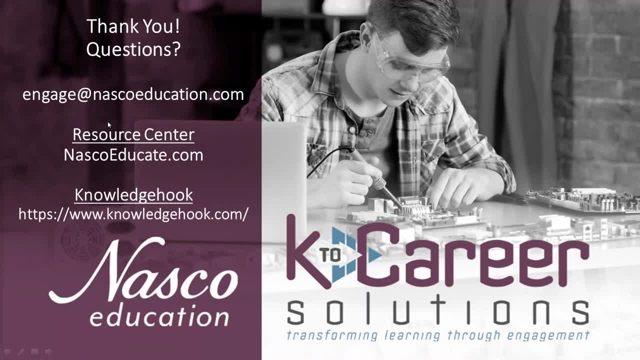 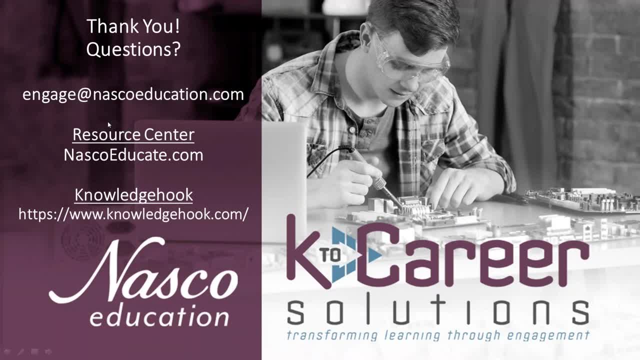 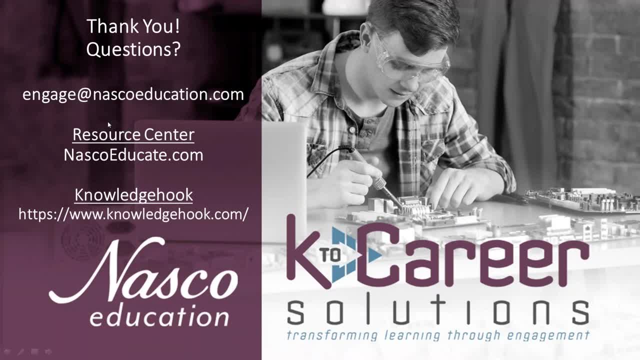 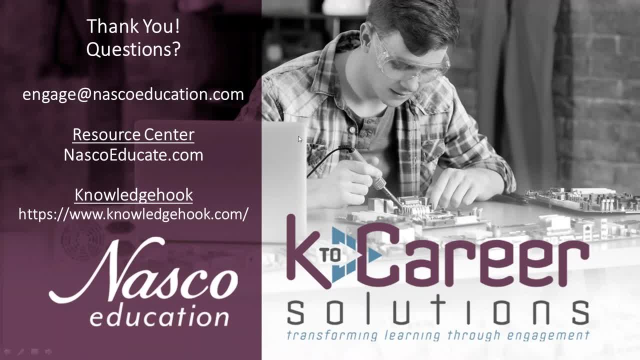 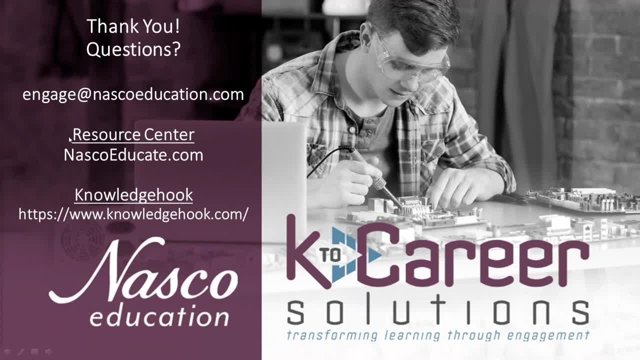 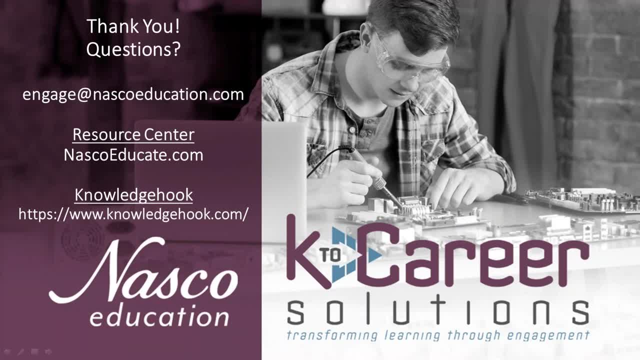 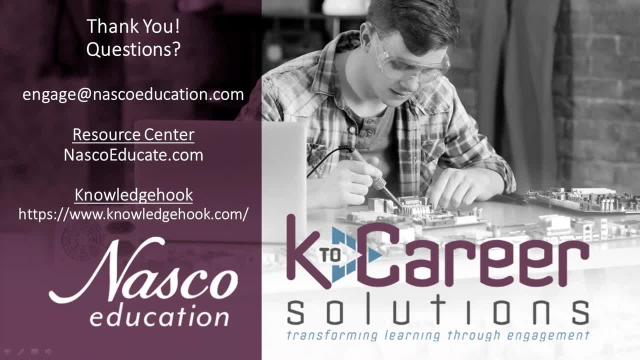 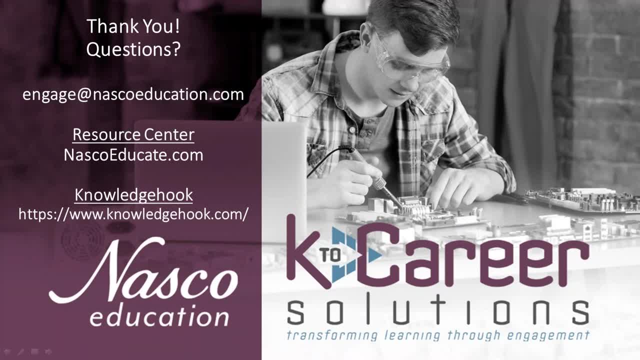 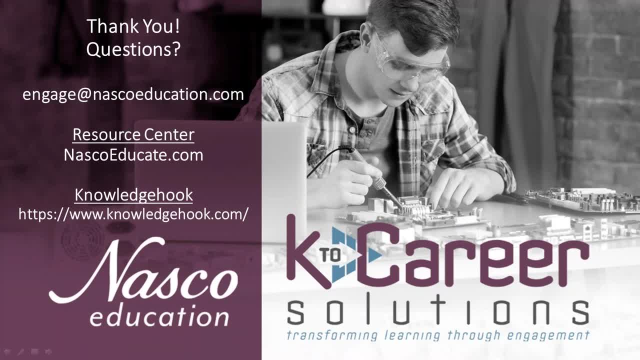 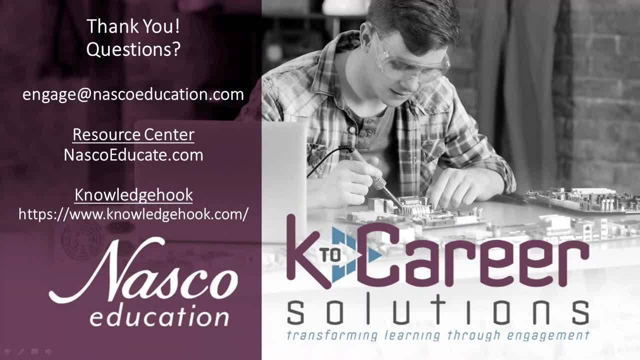 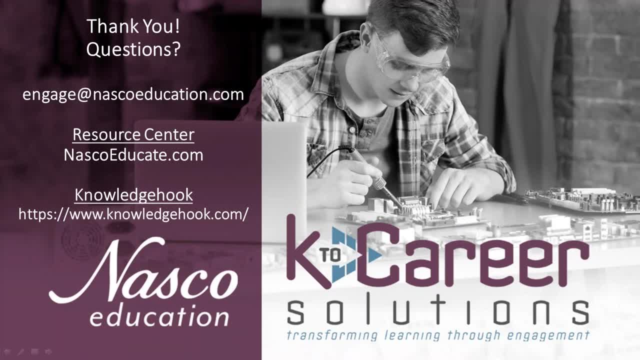 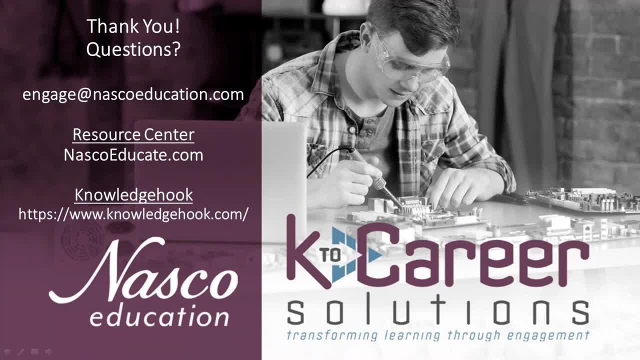